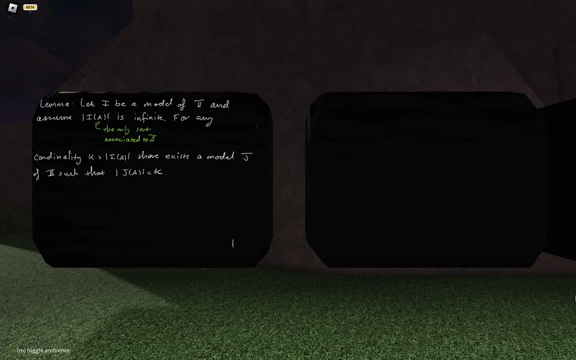 Such that the magnitude of J of A is equal to kappa. Okay, and the proof is. the proof crucially uses the compactness theorem. So all that we do is we fix a particular set of cardinality, kappa, any set whatsoever, So 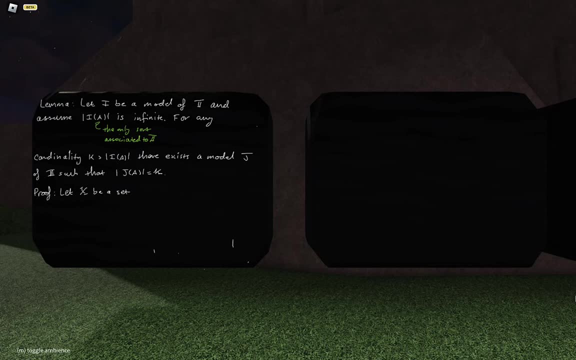 we fix a particular set of cardinality kappa. So we fix a particular set of cardinality kappa, any set whatsoever. We fix a particular set of cardinality kappa. x be such as it, Okay. and then for each x inside x, we construct a constant symbol. 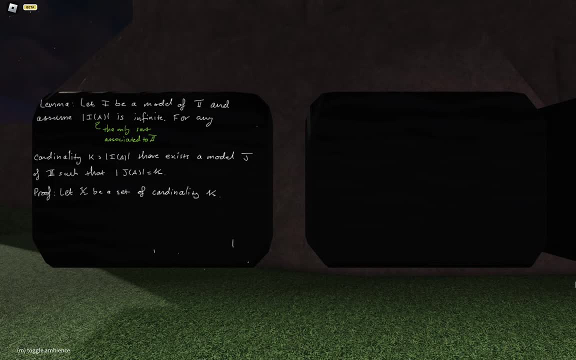 So we parameterize a collection of constants by x. So we parameterize a collection of constants by x. So we parameterize a collection of constants by x. Okay, and then what I do is I define the following set of first order formulas: 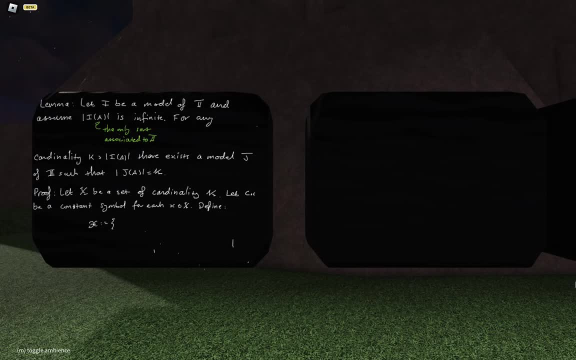 So I'm going to let squigglyX be the set of the following sentences, which is just: it's not the case that cX is equal to cY, given that X and Y are non-equal elements of X. So it's the dodgiest thing that you can possibly imagine. 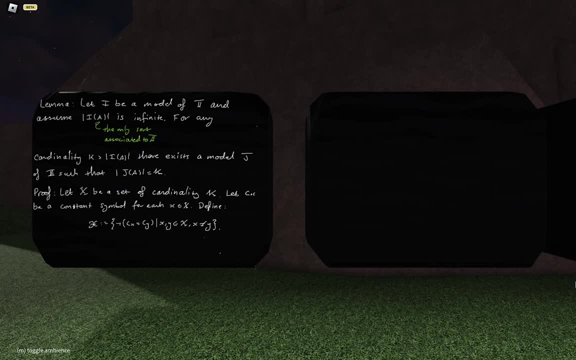 So what I'm going to do is I'm going to consider any finite subset of X and then prove that we have a model of the theory T extended by this finite subset. And all I do is I: I take the model I of A and then I interpret all of the cXs that come up inside my finite 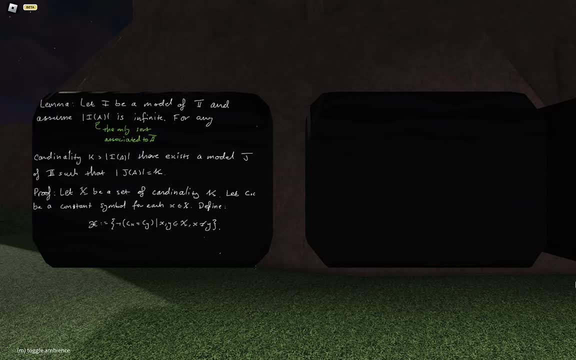 subset of X, of which there are finitely many of them as distinct elements inside I of A. Since I of A is an infinite set, this is always possible. And then by the compactness theorem, this implies that there exists a model of the union. 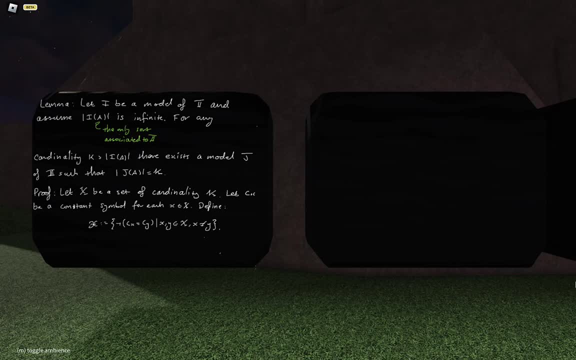 of all of these theories, which is T adjoin all of these constant symbols, Right, And then I can construct a model for the original T, which is just going to be the model for T extended to all of these constants, because I just throw away the constants and I don't. 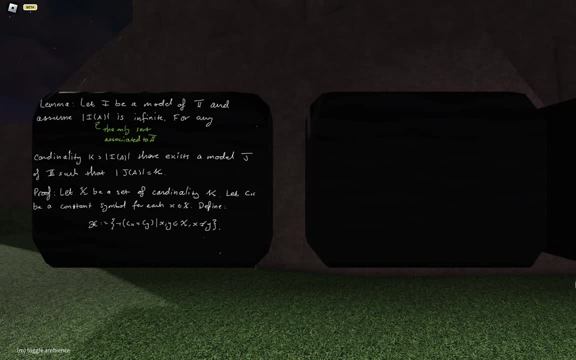 use them. And the point is, I have kappa-mini constants, and so I definitely end up with a model of size at least kappa right, And then I use the Lohenheim-Spelman theorem to reduce this down to exactly kappa. So 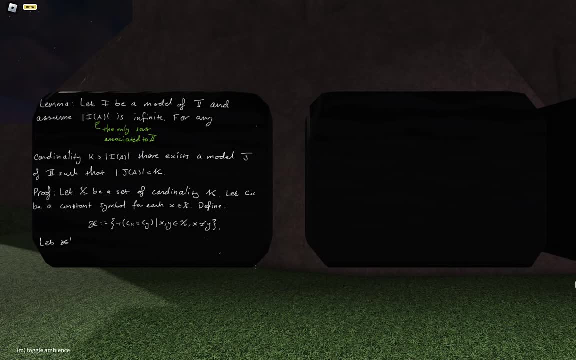 So, So, So, So So. Let squiggly be a finite subset of squiggly, then let c sub squiggly be the constants appearing in the sentences. All the formulas of squiggly. I'm on the second board now. 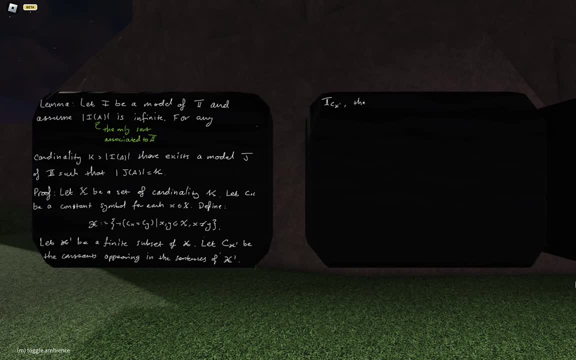 Then the theory T sub c, which is the theory T extended to the constants c. Yeah, Yeah, has a model. what I do is I take i and interpret each- let's say c- an element of cx prime as some element of i of a. 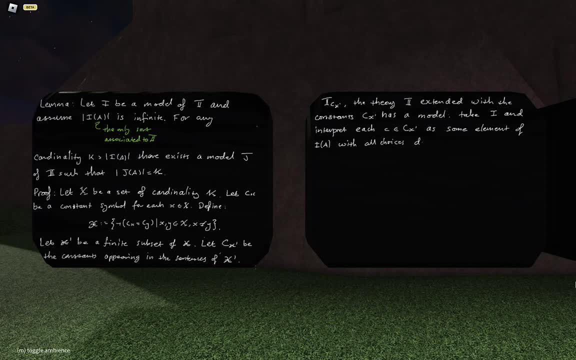 with all choices distinct. This is possible as, squiggly, x is finite and i of a is infinite. Cool, So it follows from the compactness theorem that t sub c- the theory with all extra constants- has a model. 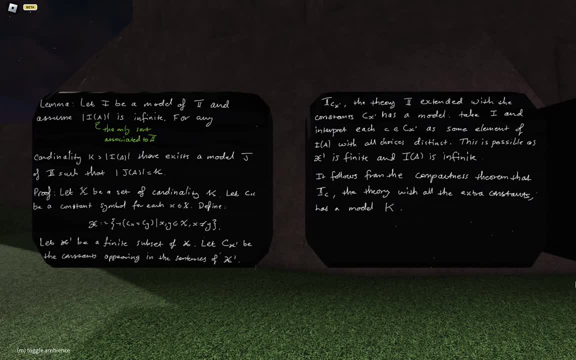 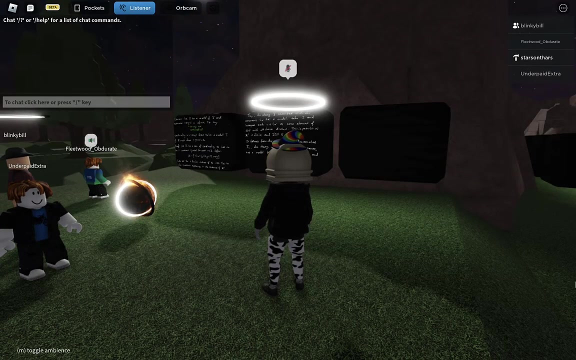 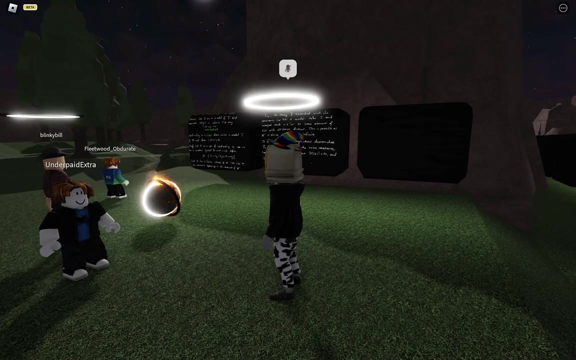 Let's call that k, Okay, and the point is that k has an interpretation for each of the constants, and they're all distinct elements, And so, therefore, the magnetism of k, of a is at least kappa, and, moreover, it is clear that kappa is a model of T. 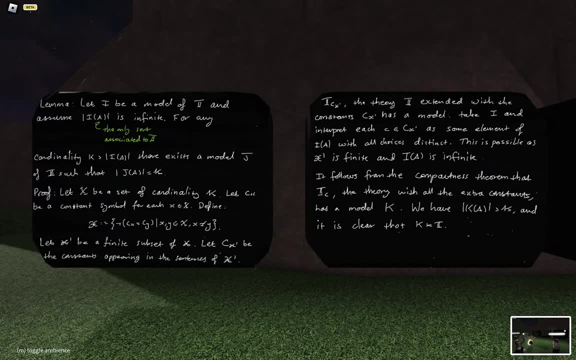 the original theory that we considered. so, lastly, we apply the lower- oh sorry, this- greater than this, greater than or equal to, so it might be of cardinality kappa on the nose, but if so, that's a coincidence. but if it's greater than that, no problem, we just pardon. oh, did someone say something? 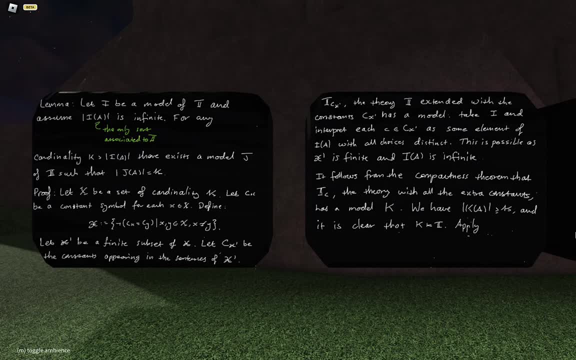 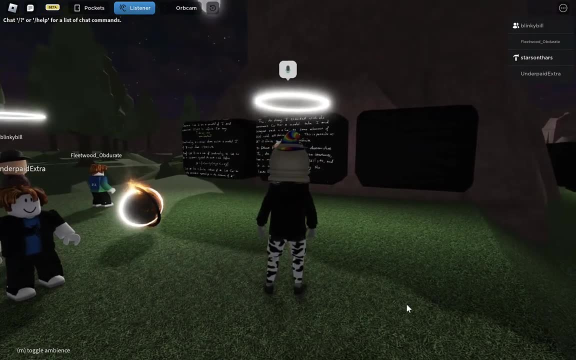 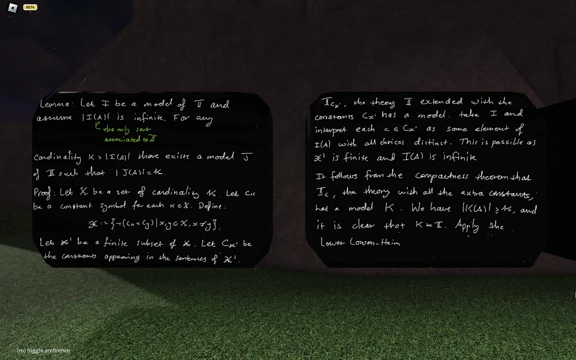 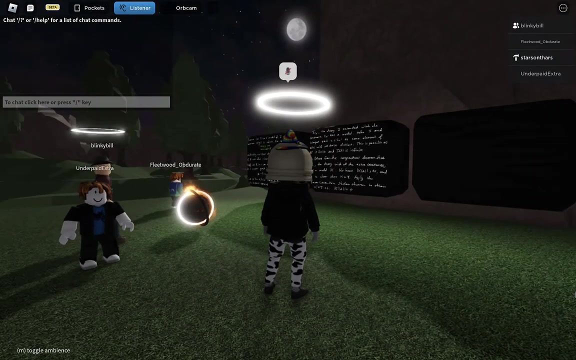 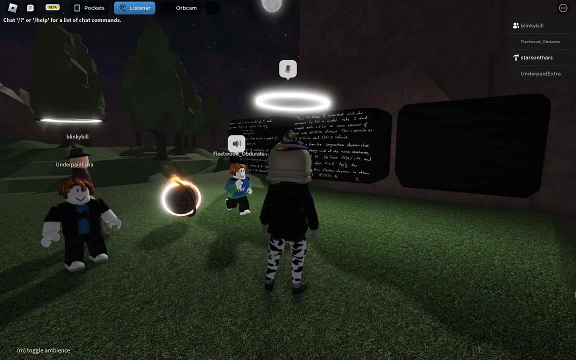 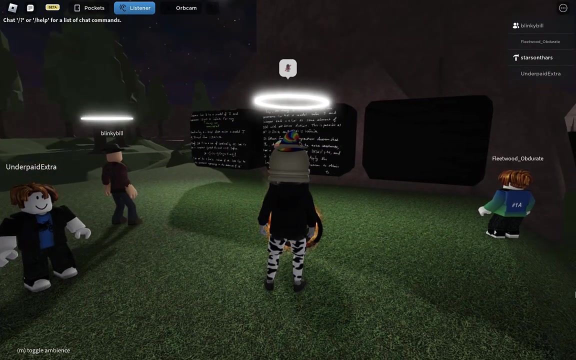 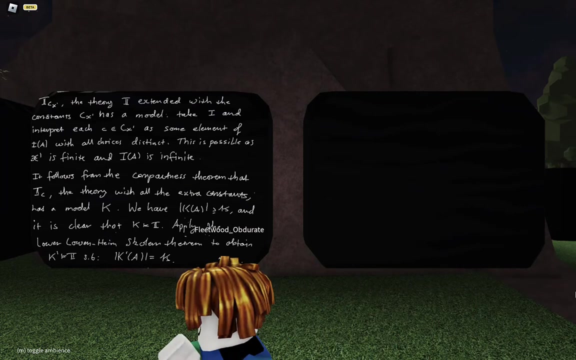 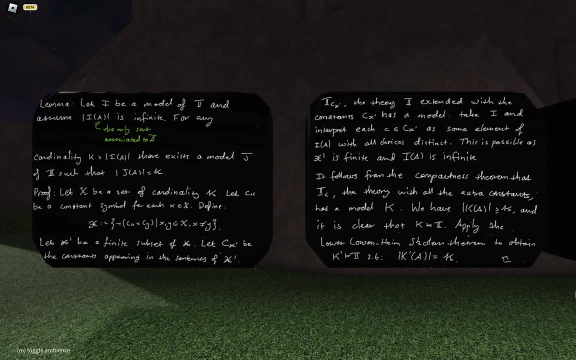 oh, I think that was actually my own voice echoing it might use for some reason. okay, apply the lower. yeah, definitely not. and some meta theory disagreement happening inside my own brain. okay, apply the lower lowenheim spelling theorem. uh, to you, you, the set x of just stuff. this is just something that we make a new constant. 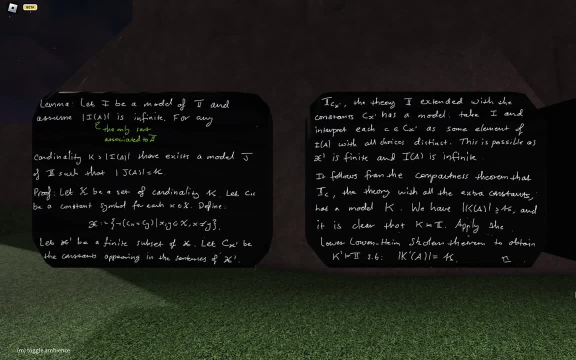 symbols out? it's not. is it related to any of the to the original model? i at all, or is it? it's just some set? no, no, so I need to assume the existence of some set of cardinality kappa, right and yeah. okay, yeah, and so I can just use the elements of x as the constant symbols. 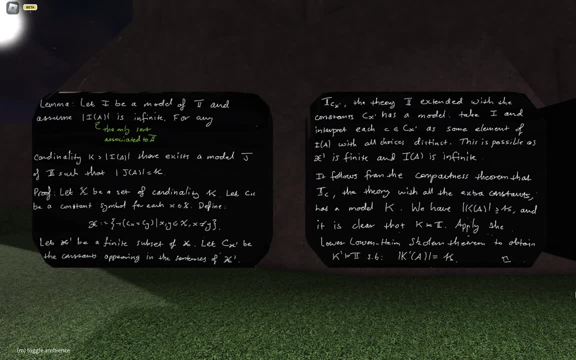 themselves, but for pedagogical reasons, I decided to make constants out of them, and I was trying to emphasize the fact that it totally doesn't matter. x is just some completely random set. as long as it has cardinality, kappa, okay, hang on. so, um, then the, so, the constant, cx, and 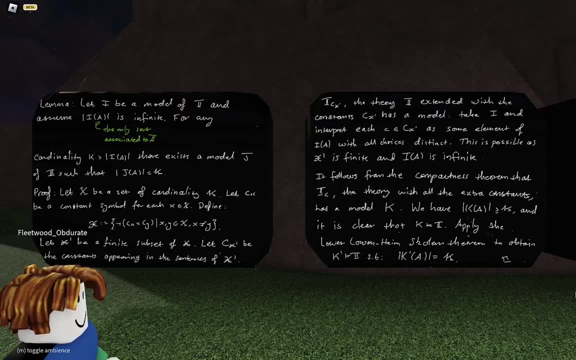 cy and so on. they they don't occur anywhere in the theory t, they're completely new, so so you can just consistently add them. add all these sentences, yeah, yeah, as you please can. what's the argument for saying like: uh, I'm just trying to try to follow why you don't just say like: 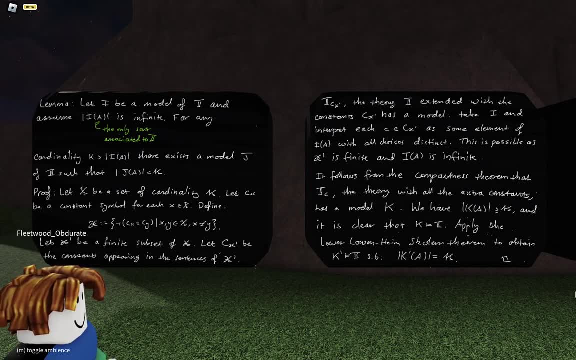 why? why doesn't the? why isn't it obvious that the whole thing has a model? oh, because the cardinality of x might be bigger than the cardinality of i of a. right now, in that situation, I'm not going to be able to pick distinct elements inside I of a in order to 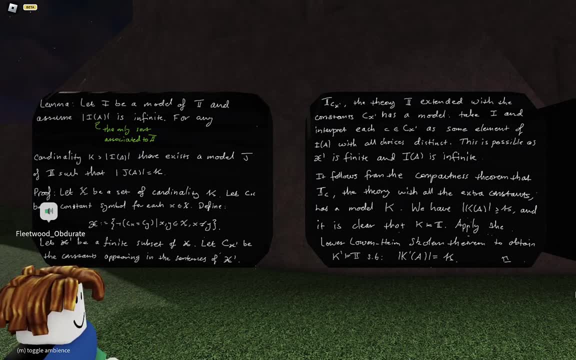 model the constants, and so in that circumstance I can't have a model of this extended Theory, because there will be some pair of constants that get mapped to the same thing. yeah, okay, um, okay, so so, but you can always do it when you you just take the finite subsets: yeah x, because then you're gonna. 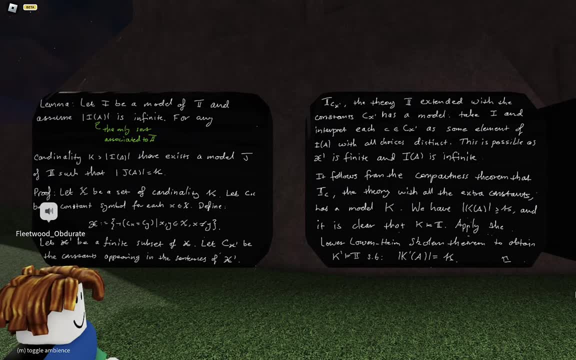 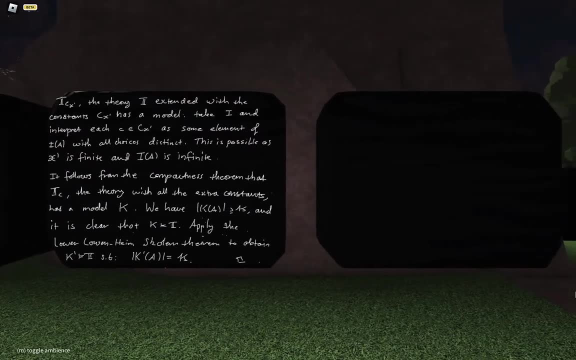 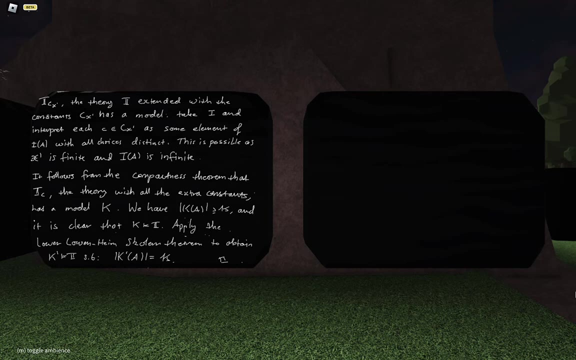 pick. finally, many distinct things. yeah, exactly, that's cool. that's like pretty crazy. yeah, like, what is your? what is your reaction to this? that like i guess is it. is it just saying that you can like, take a um, like, like the model and the the sentences in the original theory isn't really completely. 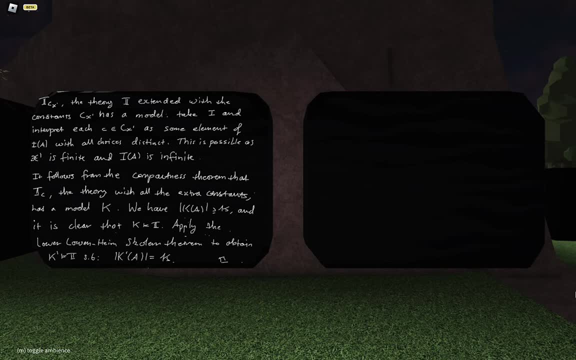 isolated from all this like extra garbage, because it's still when you have like universal quantifiers, like they have to like still be true, so they have to like still say something, or like they have to hold of all of this extra garbage that you've thrown into the, into the domain. yeah, but the 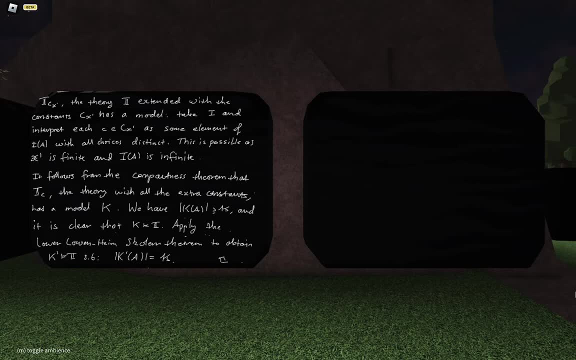 extra garbage that i've thrown in is completely disjoint, right? so what we're thinking about is so like- yeah, it's like a different. it like it is because the i haven't added elements to i of a, so i'm only considering finite collections of the constants at any particular time, and so the elements that i pick are genuine. 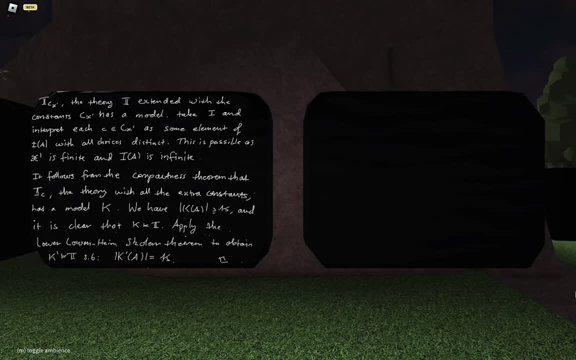 elements of i of a. so i'm only considering finite collections of the constants at any particular time. i don't think the right way is to extend to i of a. i don't extend i of a. i don't extend i of a until i appeal to the Compactness Theorem. 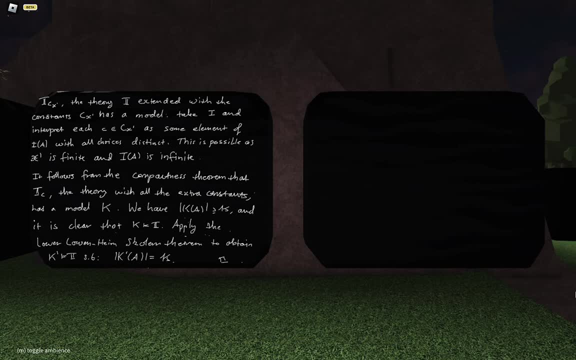 and at that point there's a lot involved in that maneuver, right? so i'm using the Compactness Theorem and you prove the Compactness Theorem using the Complete Ne's Theorem, right? so there is some crazy process that gets applied to i of a and all of its finite sub-models. 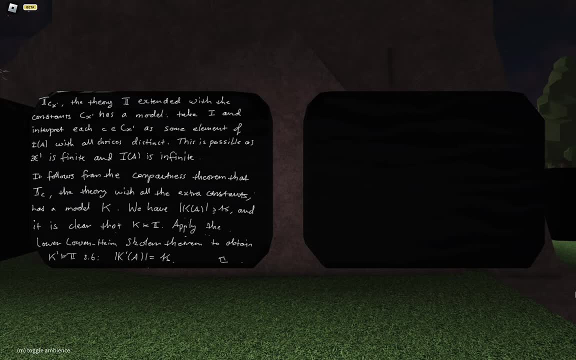 that then produces some unwieldy big thing, and i don't feel like i have off the top of my head that i think you're, along the a-act of time, the top of my head knowledge of that. i just believe that there is some process that we've 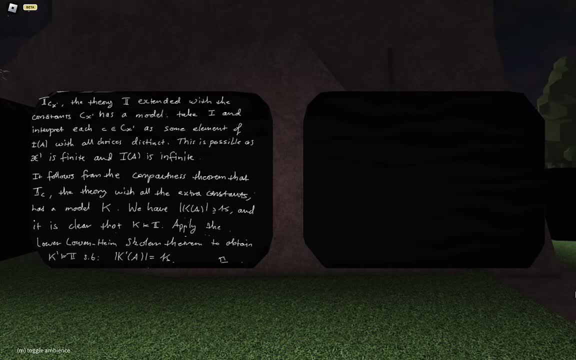 a priori discussed, and the result of it is some uh model which has to be consistent, and so there has to be at least kappa many distinct elements inside it, and so therefore it must have cardinality, at least kappa right. so it's a hands-off proof, it's an indirect argument, that last step, that 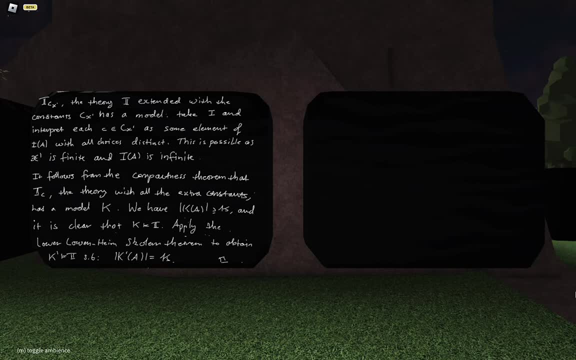 you just described like the, the logical step from uh- knowing that every every one of these sentences of squiggly x is true in the model um- to like uh, to knowing the size of the model k. oh so, like, like what? what's the like? how? how do you determine whether, like a set has a certain size? like, usually, you form like a. 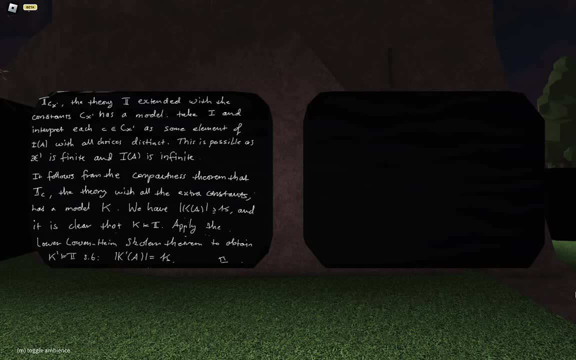 bijection or something right. so so there's an injection. there's an injection from x into the model that i end up with, because c- x is interpreted as some element. it's provably not equal to any of the other elements of the form: c sub y, where x is not equal to y, right, and so that element, that c, x, 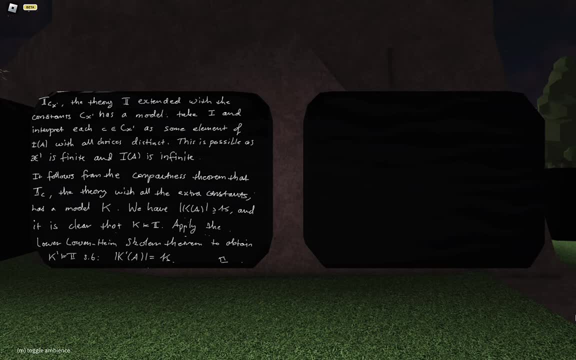 gets interpreted as map x inside capital x to that element. right, yeah, that's an injective map from x to the set, and so therefore, the set has cardinality, at least that of x, which means it has cardinality at least kappa you, yeah, okay, that seems pretty reasonable. 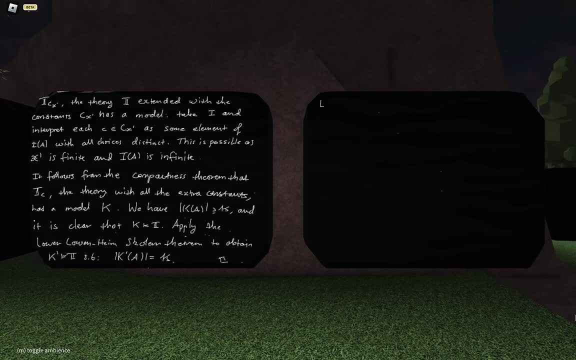 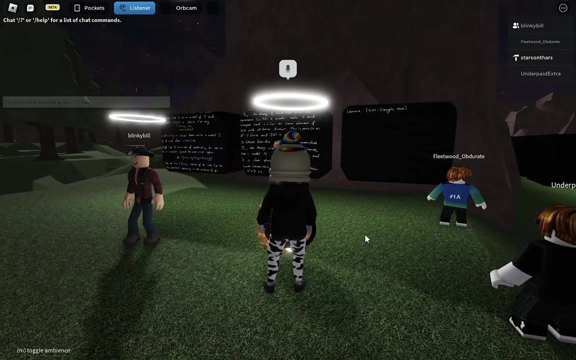 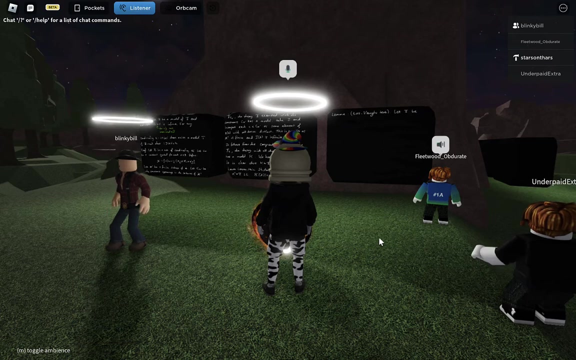 yeah, okay, let's move on. so now we get the wash vort test. i should spell it with an l, stupid comment, but every time i hear this, i think of the test in blade runner. i haven't seen blade runner, okay, okay, okay, it's the test for whether you're a replicant or not, whether you're a real human. 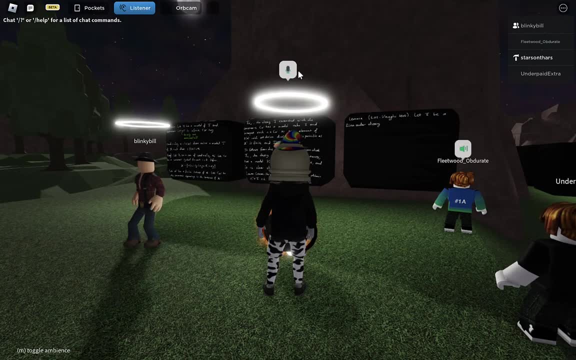 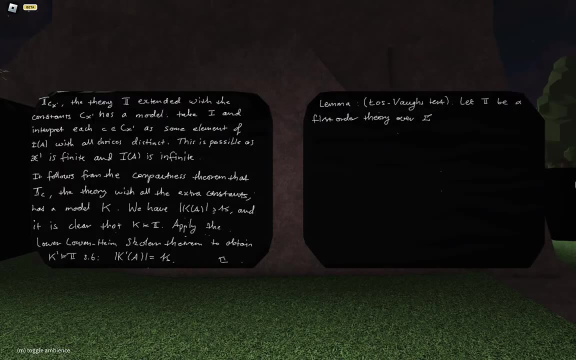 oh, i see it sounds sort of. i think it's going to sound more similar as i write out the level. okay, let t be some first order theory, um, over some first order signature sigma where, uh, and i'm not assuming that it has one thought, i'm sorry, one sort at this exact point in time, but that's going. 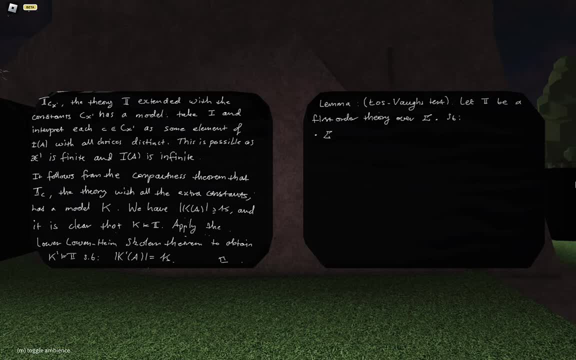 to be literally the test for whether you're a replicant or not, whether you're a real human or not. whether you're a real human, my first dot point, so assume sigma has only one sort. this lemma holds in more generality than this, but this is the only one that we've proven and this is the only one that we need for the x growth and 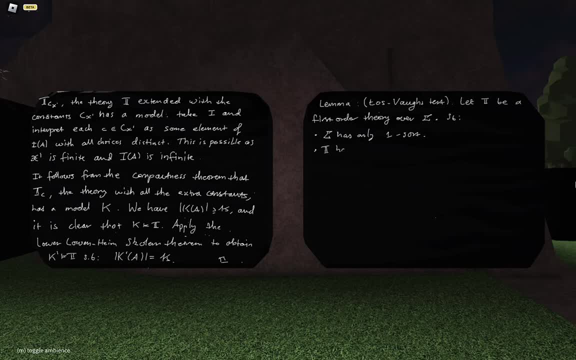 d theorem. so it's fine, sim t has no finite models, okay, and assume that there exists. okay, and assume that there exists. okay, and assume that there exists some cardinality kappa, which is necessarily infinite due to dot point two, for which there is exactly one model, up to isomorphism. 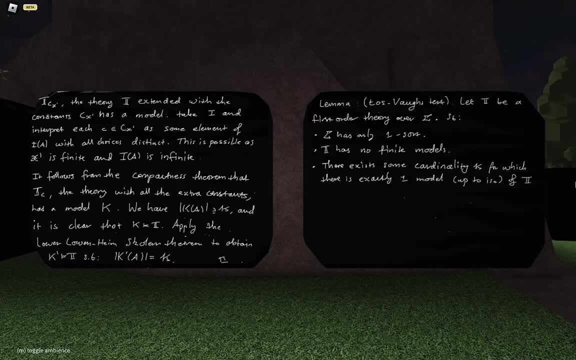 of t of size kappa. exactly one model up to isomorphism of t of size kappa. exactly one model up to isomorphism of t of size kappa. okay, and so the example that we want to have in our hands obviously are algebraically closed. okay, and so the example that we want to have in our hands obviously are algebraically closed. 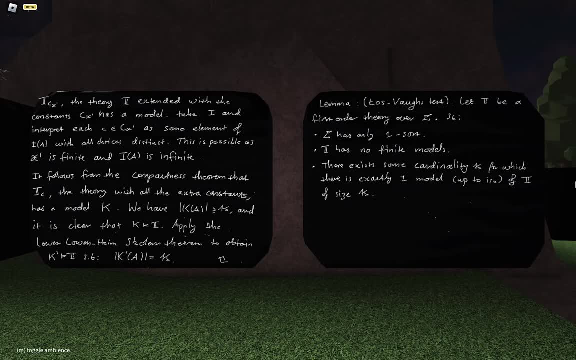 fields. okay, so to the geometries in the room. it's standard theory that there are no finite algebraically closed fields and for any cardinality there is exactly one algebraically closed field of that cardinality, up to isomorphism. when you, when you pick a particular characteristic as well, 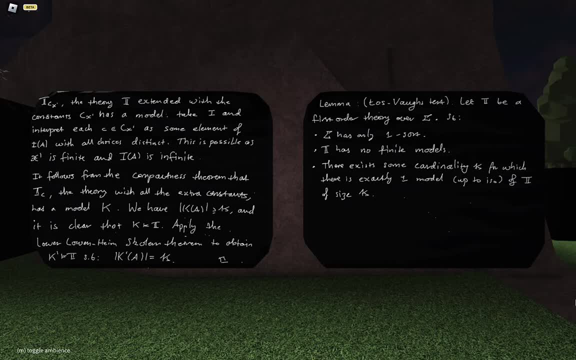 so that's the motivating example from our perspective, but this is a general test. so that's the motivating example from our perspective, but this is a general test that holds, um, and what it says is that if this holds, then t is complete. okay, and again, the proof is simple, but it seems a lot less hacky than than normal, so that's good. 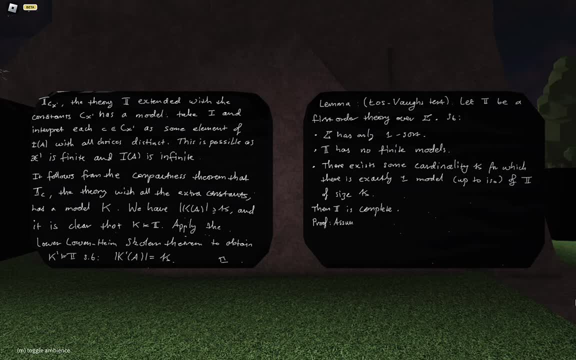 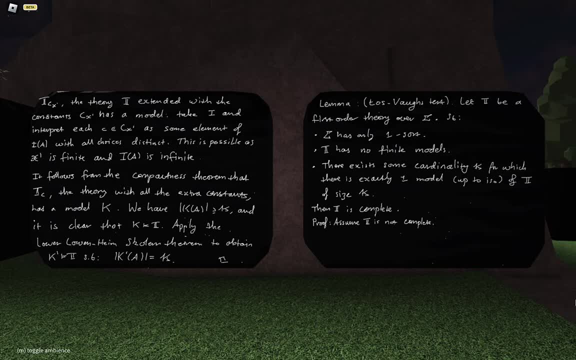 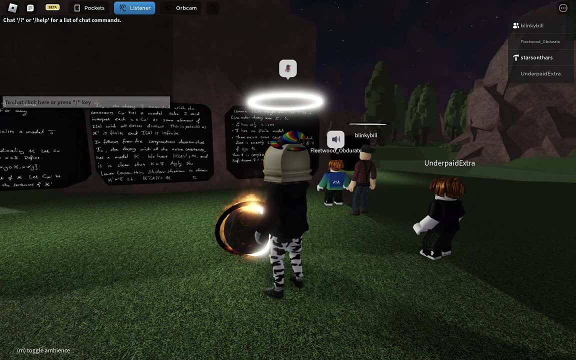 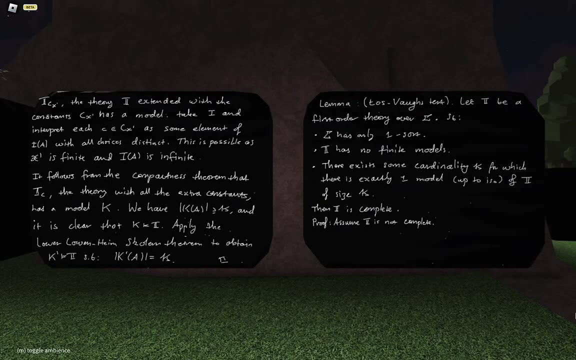 like model isomorphism, but you just mean like the like: is it just the size of the set, or uh, it's not necessarily the size of the set, it's yeah, so you need to talk about morphisms of uh, what models or theories? so i suppose, 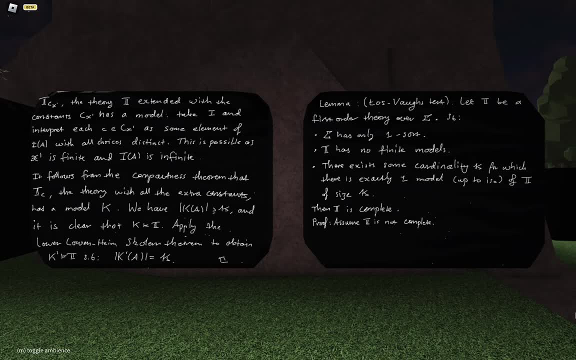 so i suppose. so you need to talk about morphisms of uh what models or theories. so i suppose the pause is i'm going through my notes. i think i the pause is i'm going through my notes. i think i the pause is i'm going through my notes. i think i actually had this at some point. 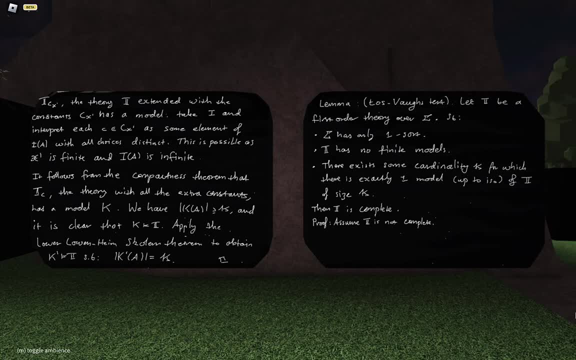 actually had this at some point, actually had this at some point. yeah, yeah, so there are morphisms of interpretations, yeah, so you have, you have a fixed first order. you have, you have a fixed first order. you have, you have a fixed first order. theory, theory, theory, and then you might have two different. and then you might have two different, and then you might have two different interpretations of it. and there is such interpretations of it and there is such interpretations of it. and there is such thing as a morphism thing, as a morphism thing, as a morphism, and there is such thing as a morphism. 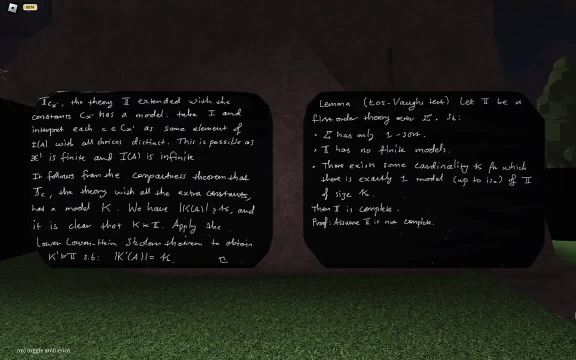 and there is such thing as a morphism from these interpretations, from these interpretations, from these interpretations, and it's it's obvious what it is and it's it's obvious what it is, and it's it's obvious what it is. so i need a more, i need a function. 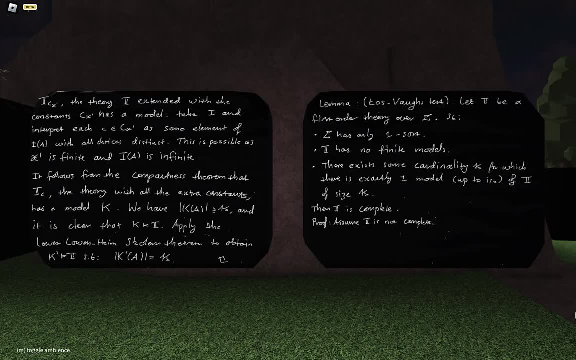 so i need a more. i need a function. so i need a more. i need a function from the domain of the first, from the domain of the first, from the domain of the first interpretation to the domain of the interpretation, to the domain of the interpretation, to the domain of the second interpretation. 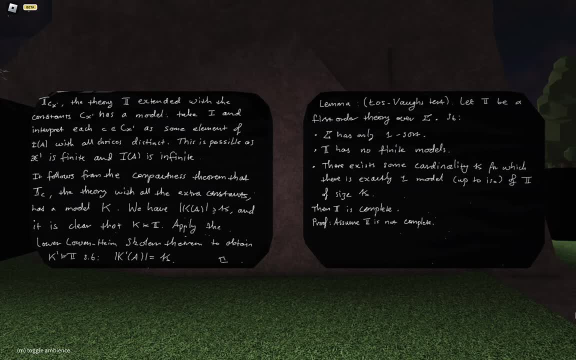 second interpretation, second interpretation, and i need these to be coherent and i need these to be coherent and i need these to be coherent with the, the interpretations of the, with the, the interpretations of the with the, the interpretations of the function symbols and the interpretations of function symbols and the interpretations of. 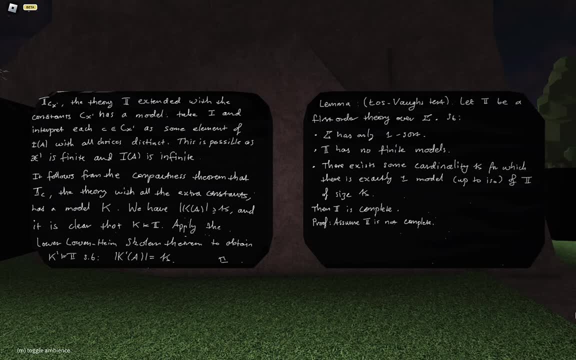 function symbols and the interpretations of the predicates or the relation symbols, and if you have a reverse map, then and if you have a reverse map, then. and if you have a reverse map, then, or an inverse map, then you have an, or an inverse map, then you have an. 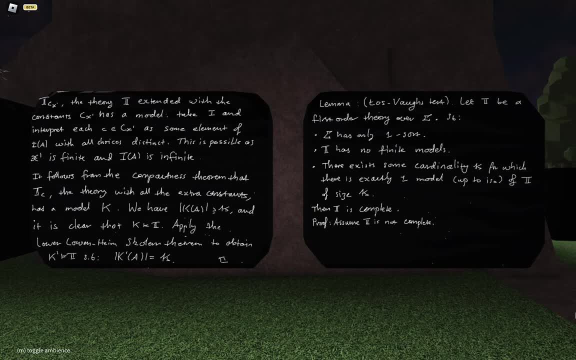 or an inverse map. then you have an isomorphism, isomorphism, isomorphism, so in, so in so, in the example of algebraically closed, the example of algebraically closed, the example of algebraically closed fields that's going to be a fields that's going to be a. 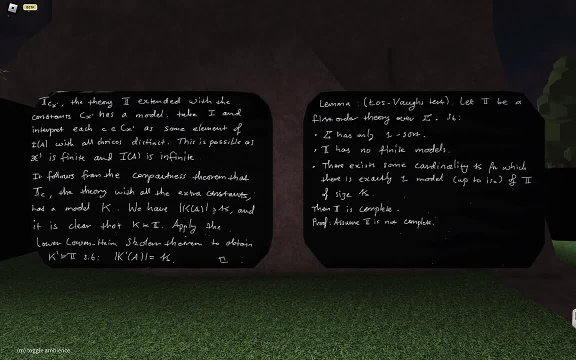 fields. that's going to be a field isomorphism field, isomorphism, field, isomorphism- yeah, yeah, yeah, cool, cool, cool, okay, okay, okay. now, if we assume that t is not complete now, if we assume that t is not complete now, if we assume that t is not complete, then 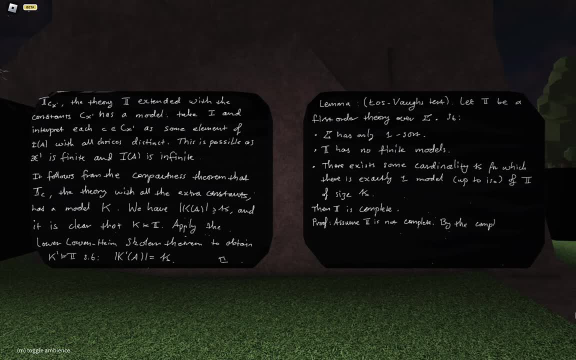 then, then, by by, by the completeness theorem, the completeness theorem, the completeness theorem, we actually have, we actually have. we actually have a pair of models in our hands, one of a pair of models in our hands, one of a pair of models in our hands, one of which models? 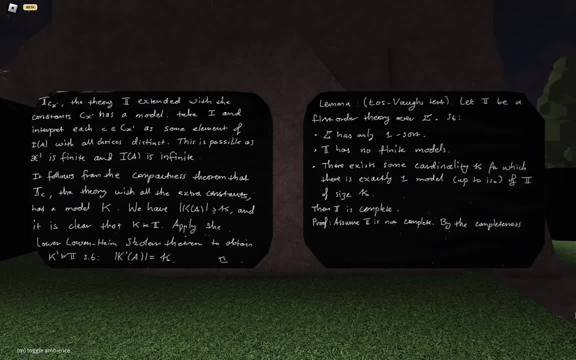 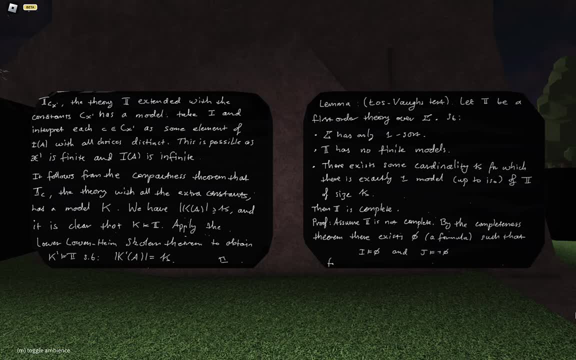 i models, phi and j models. the negation of phi and j models. the negation of phi and j models. the negation of phi. for some models i and j. for some models i and j okay, and then some models i and j okay, and then some models i and j okay, and then we're done because. 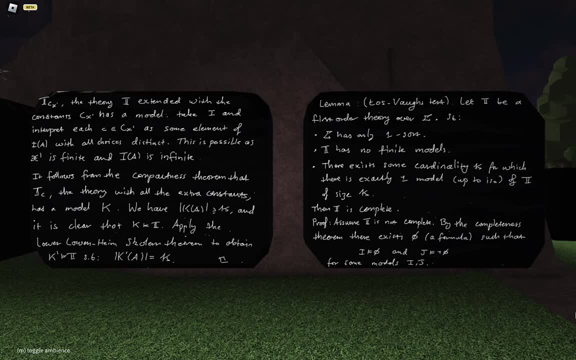 we're done. because we're done because we know that we have no. we know that we have no, we know that we have no finite models right, and so what that? finite models right, and so what that? finite models right? and so what that means is that i and j 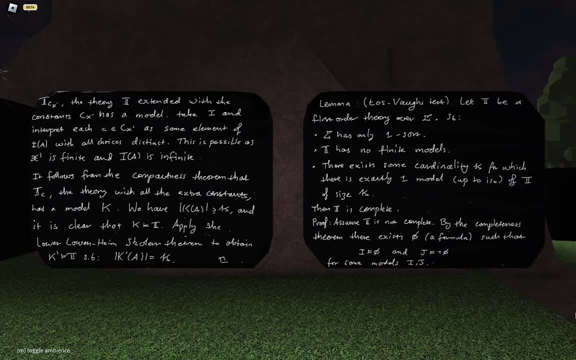 means is that i and j means is that i and j are both infinite, and then we can use the are both infinite, and then we can use the are both infinite, and then we can use the loewenheim's golem theorem. loewenheim's golem theorem. 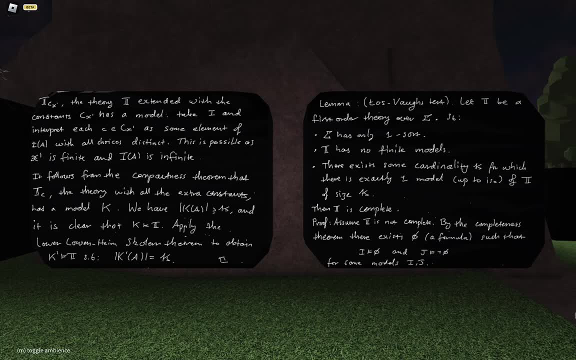 loewenheim's golem theorem. so i and j are both infinite of some, so i and j are both infinite of some. so i and j are both infinite of some. cardinalities: kappa 1 and kappa 2. cardinalities: kappa 1 and kappa 2. 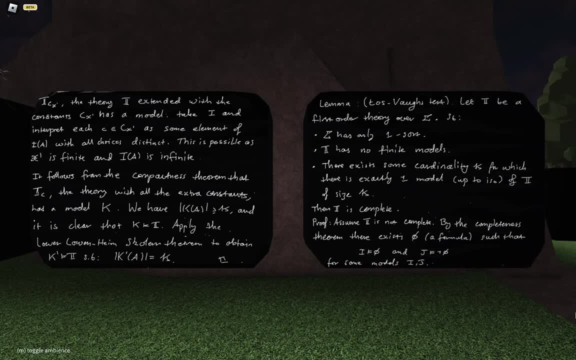 cardinalities, kappa 1 and kappa 2, say: but whatever they are um i can say: but whatever they are um. i can say: but whatever they are, um i can come up with a new model of come up with a new model of come up with a new model of uh. 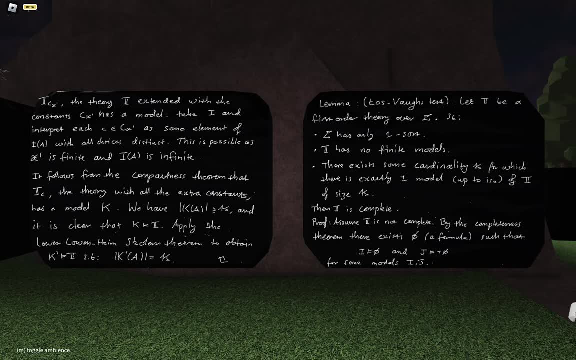 uh, uh, wait, sorry, wait, sorry, wait, sorry, yeah, yeah, yeah, yeah, there exists, yeah, there exists, yeah, there exists. oh, wait, how do i get the preservation? oh, i see okay, oh, i see okay, oh, i see okay, i, i see, okay, i, i see okay, i sorry, okay, let me move to the other. 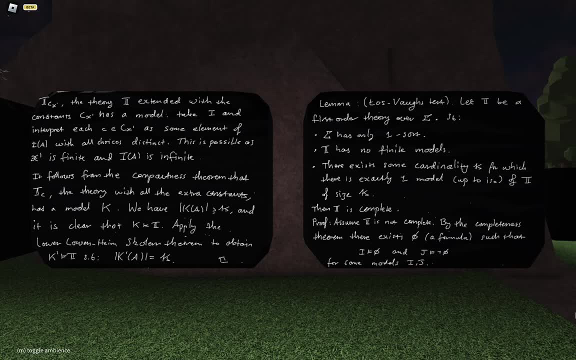 sorry, okay, let me move to the other. sorry, okay, let me move to the other board. to make this precise, i think it's board to make this precise. i think it's board to make this precise. i think it's confusing because i'm saying it that, confusing because i'm saying it that. 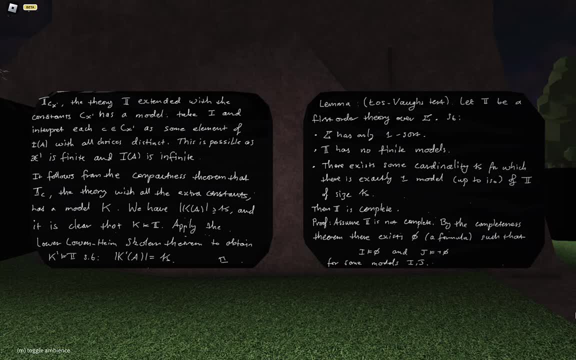 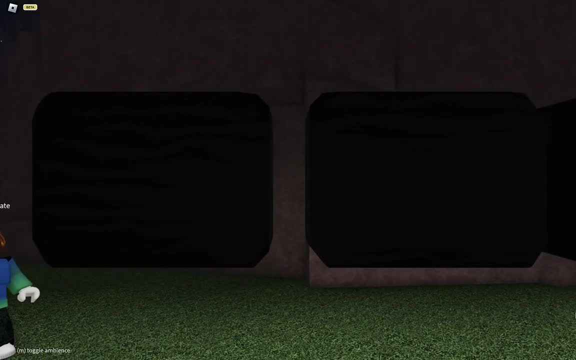 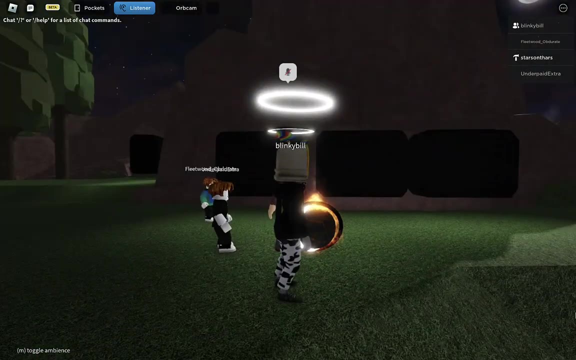 confusing because i'm saying it that loud. so let's move over to the next loud. so let's move over to the next loud. so let's move over to the next board. okay, so i and j okay. so i and j okay, so i and j are. 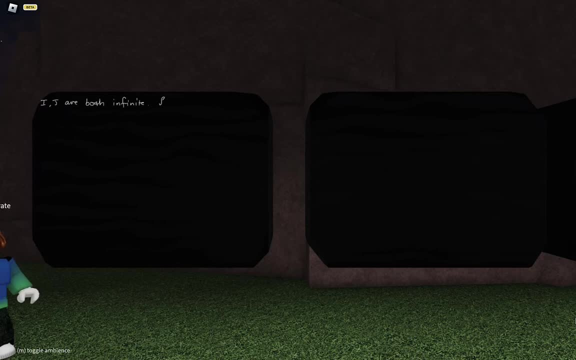 are, are, are both infinite. so, by lovenheim's column, there exists a. so, by lovenheim's column, there exists a. so, by lovenheim's column, there exists a model, model, model k, k, k of t, of t, of t, such that, such that. 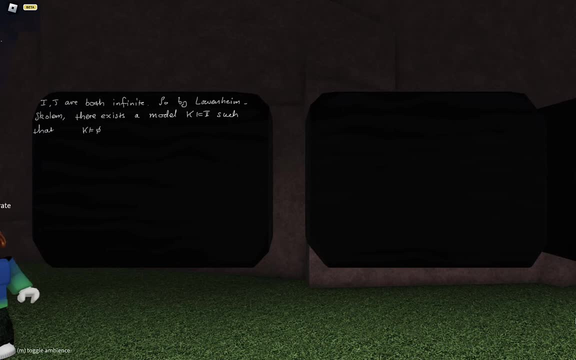 such that k models, phi, k models, phi, k models, phi and k and k and k models with a negation of phi, models with a negation of phi, models with a negation of phi, which is a contradiction right. so which is a contradiction right? so which is a contradiction right. so the way that you want to think about this, 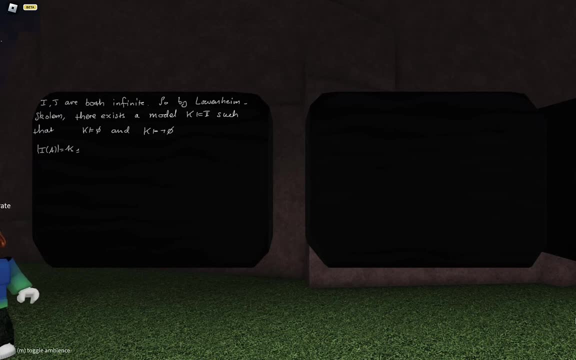 the way that you want to think about this. the way that you want to think about this, is i of a might have some cardinality? is i of a might have some cardinality? is i of a might have some cardinality? kappa one, and then the magnitude of j. 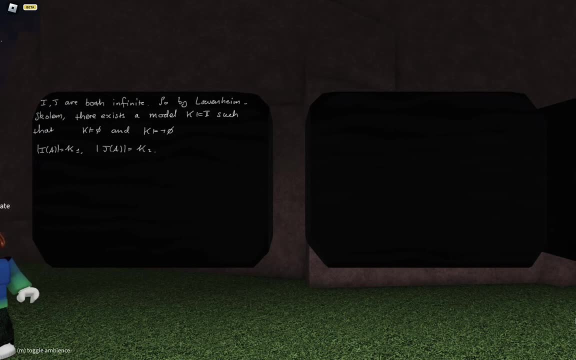 kappa one, and then the magnitude of j: kappa one, and then the magnitude of j of a might be equal to kappa two. say of a might be equal to kappa two. say of a might be equal to kappa two. say then, if kappa one and kappa two, then if kappa one and kappa two. 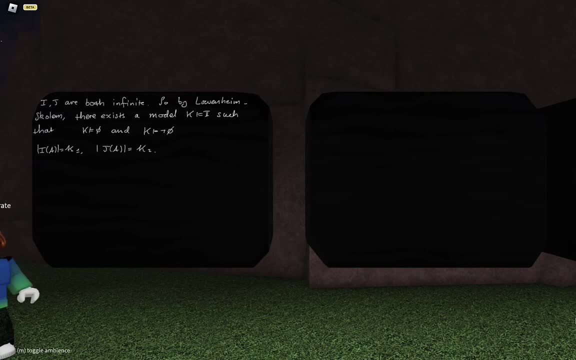 then if kappa one and kappa two are equal in cardinality, then you're are equal in cardinality, then you're are equal in cardinality, then you're already done right, because we only have already done right, because we only have already done right, because we only have one model up to isomorphism for a. 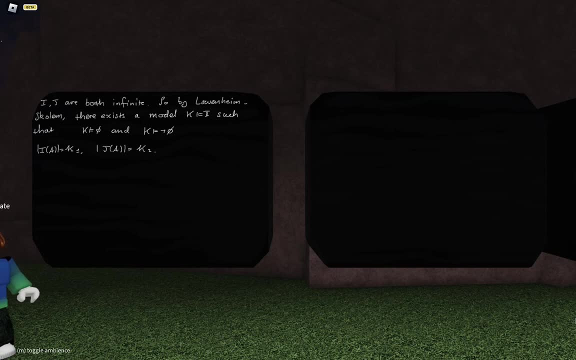 one model up to isomorphism for a. one model up to isomorphism for a particular, particular, particular. oh, i guess we need to okay. oh, i guess we need to okay. oh, i guess we need to okay. so the assumption in the hypothesis was: so the assumption in the hypothesis was: 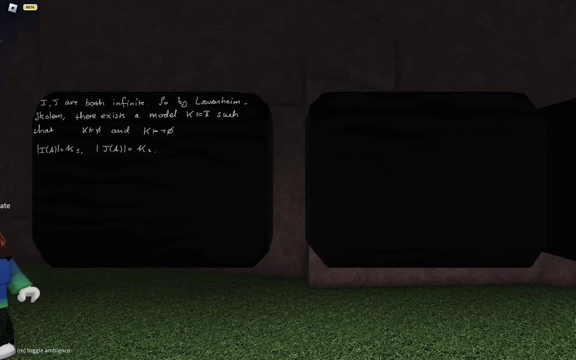 so the assumption in the hypothesis was that there exists, that there exists, that there exists some kappa for which there is exactly some kappa, for which there is exactly some kappa, for which there is exactly one model, one model, one model, um of t, of size, kappa, up to isomorphism. 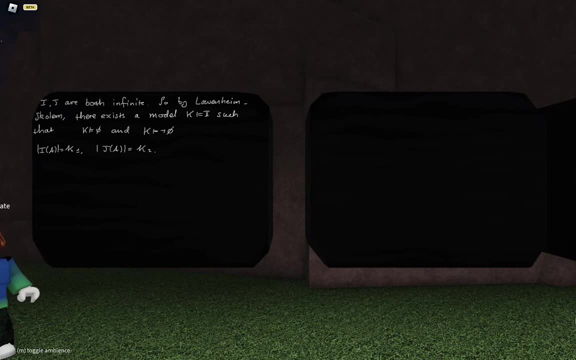 um of t of size kappa up to isomorphism. um of t of size kappa up to isomorphism. so i actually have a kappa sitting. so i actually have a kappa sitting, so i actually have a kappa sitting around, around around. so so yeah, this isn't quite correct. 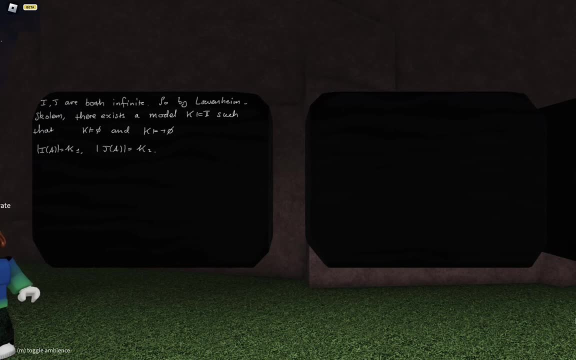 so so, yeah, this isn't quite correct. so so, yeah, this isn't quite correct- what i've written on the board, what i've written on the board, what i've written on the board. so so that, yep, no, that is fine, just ignore. so that, yep, no, that is fine, just ignore. 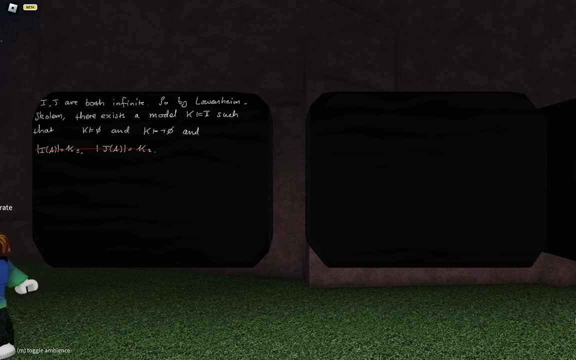 so that, yep, no, that is fine, just ignore that sentence, that sentence, that sentence essentially this holds, and the essentially this holds, and the essentially this holds, and the magnitude of k, magnitude of k, magnitude of k of a is equal to kappa of a is equal to kappa. 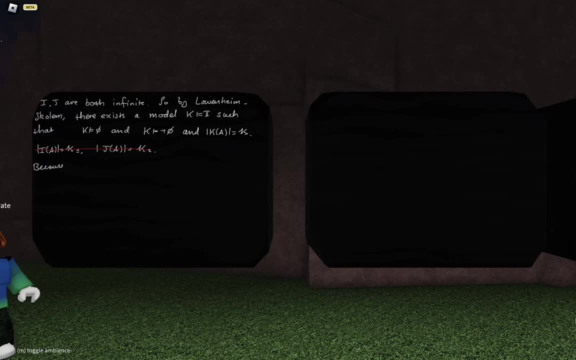 of a is equal to kappa, right? this is because there is only one. there is only one. there is only one model of size. model of size, model of size kappa up to isomorphism. okay, and where we used the lohenheim: okay, and where we used the lohenheim. 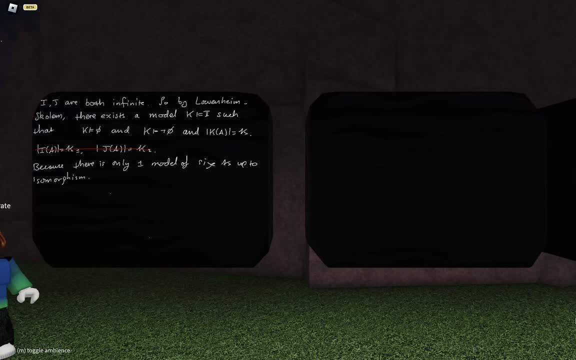 okay, and where we used the lohenheim. scolem theorem is in the construction. scolem theorem is in the construction. scolem theorem is in the construction of the model. okay of the model. okay of the model. okay, does that make sense? sorry, that's a. does that make sense? sorry, that's a. 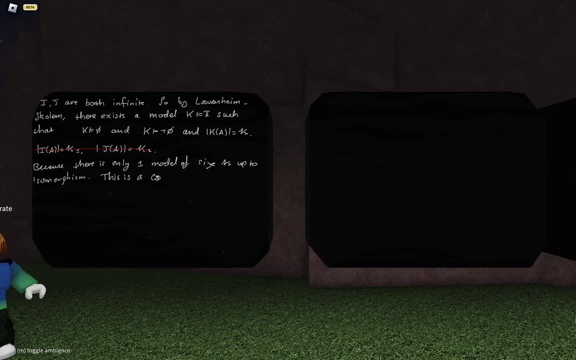 does that make sense? sorry, that's a contradiction. contradiction- does that make sense? sorry, that's a contradiction. so t is complete, okay. so the next step is to okay. so the next step is to okay. so the next step is to show that the first order theories of 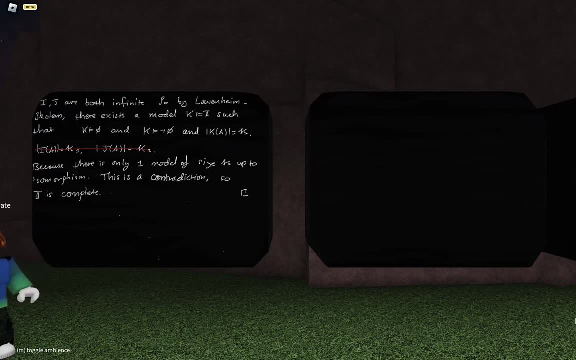 show that the first order theories of show that the first order theories of algebraic closed fields of either algebraic closed fields of either algebraic closed fields of either characteristic zero or p when p is in characteristic zero, or p when p is in characteristic zero, or p when p is in prime. 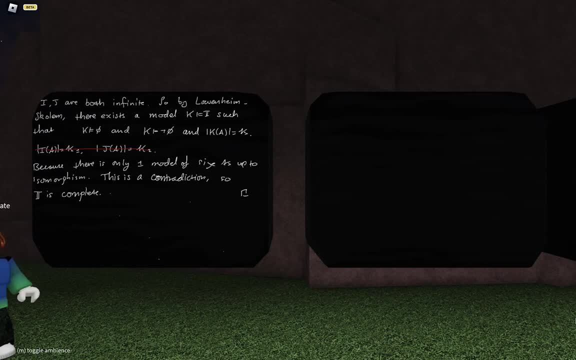 prime, prime. satisfy the criteria inside. satisfy the criteria inside. satisfy the criteria inside the uh wash vort test. the uh wash vort test, the uh wash vort test. so before i jump over to algebraic um, so before i jump over to algebraic um, so before i jump over to algebraic um stuff, are there any questions on this? 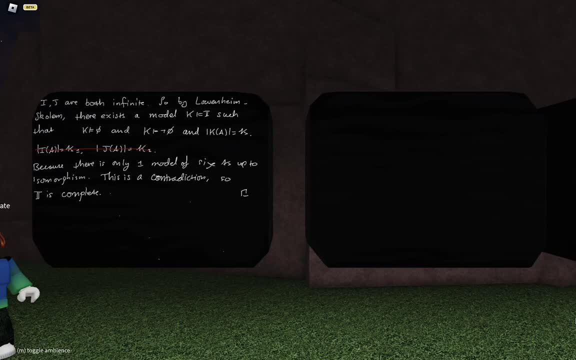 stuff. are there any questions on this stuff? are there any questions on this proof? okay, so, lemma, if k, lemma, if k, lemma, if k is algebraically closed, is algebraically closed, is algebraically closed, then then then k is infinite and cardinality. k is infinite and cardinality. 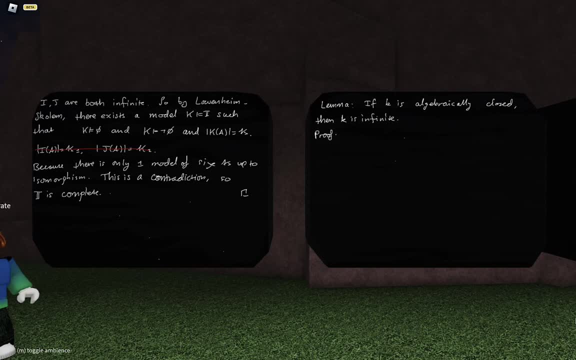 k is infinite and cardinality, and this is a really slick argument. and this is a really slick argument and this is a really slick argument. it's one of those. it's one of those, it's one of those very simple but nice ideas. so very simple but nice ideas. so 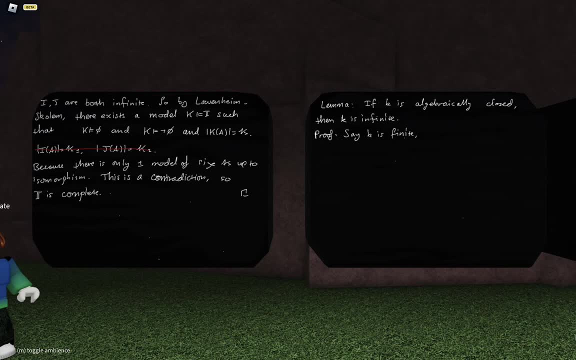 very simple but nice ideas. so say k is finite, say k is finite, say k is finite, then then, then consider, consider, consider the following polynomial: so i set f of x. the following polynomial: so i set f of x. the following polynomial: so i set f of x to be one. 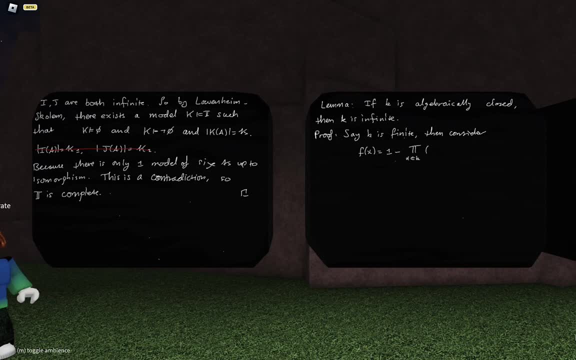 to be one to be one minus the product over all alpha. in minus the product over all alpha. in minus the product over all alpha. in element in kappa of x minus alpha. this is element in kappa of x minus alpha. this is element in kappa of x minus alpha. this is an element of: 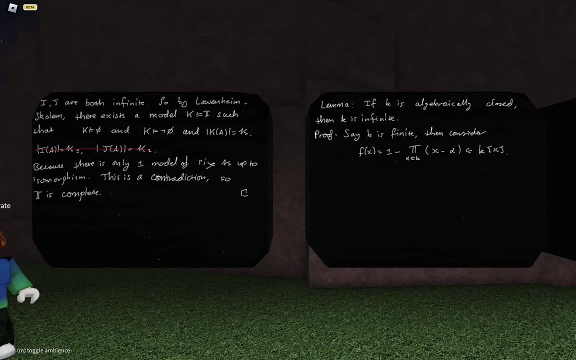 an element of an element of this polynomial root right. and if i this polynomial root right and if i this polynomial root right, and if i evaluate f at any alpha inside k, then we evaluate f at any alpha inside k. then we evaluate f at any alpha inside k, then we can see that i get the value one which 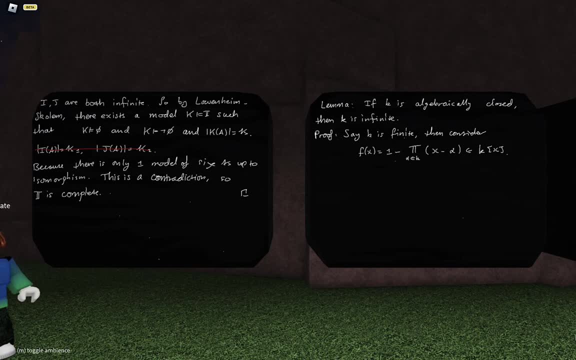 can see that i get the value one, which can see that i get the value one which is not equal to zero is not equal to zero, is not equal to zero, and so therefore k is not algebraically, and so therefore k is not algebraically, and so therefore k is not algebraically closed. 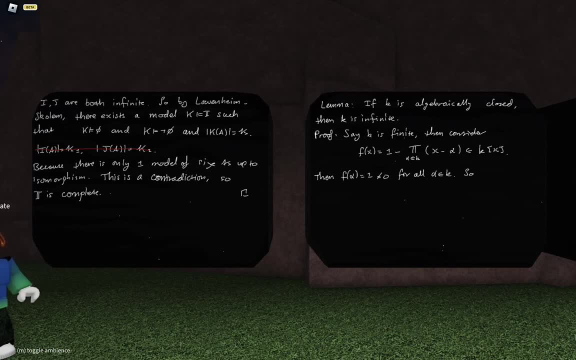 next, next, next. yes, it's nice, isn't it okay? and so that's the second dot point. okay, and so that's the second dot point. okay, and so that's the second dot point of the of the, of the? uh, what vort test, uh telling us that. 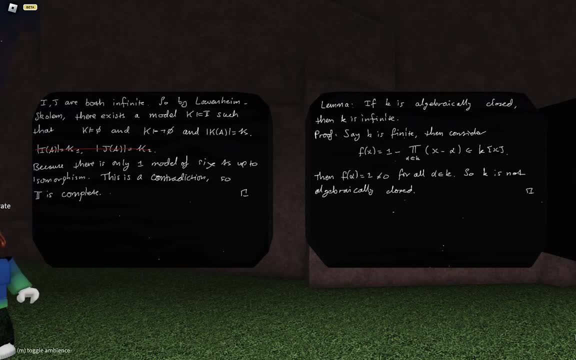 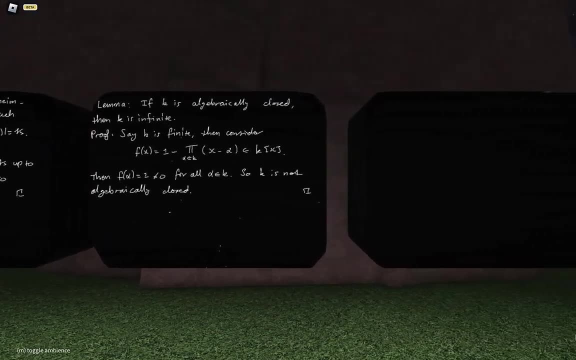 uh, what vort test uh telling us that? uh, what vort test uh telling us that there are no, there are, no, there are no finite models of these algebraically finite models of these algebraically finite models of these algebraically closed, closed, closed uh, fields. sorry, no finite. 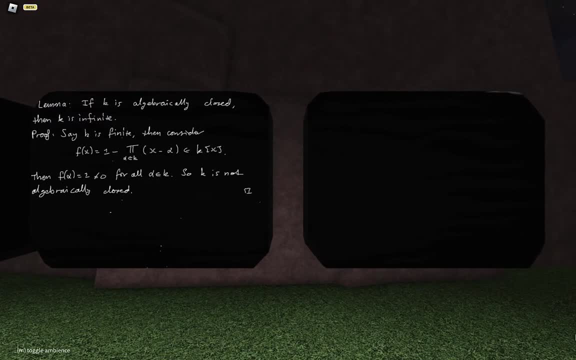 sorry, no finite, sorry, no finite models of the algebraically closed models of the algebraically closed models of the algebraically closed theories, which is theories, which is theories, which is which is just the algebraically closed, which is just the algebraically closed, which is just the algebraically closed fields. 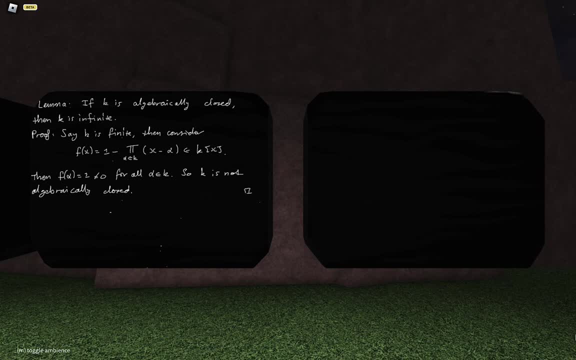 fields, fields. okay, hearing this theorem also kind of okay. hearing this theorem also kind of okay. hearing this theorem also kind of like, like, like it is also saying that, uh, it is also saying that, uh, it is also saying that, uh, like, there's no way to sort of. 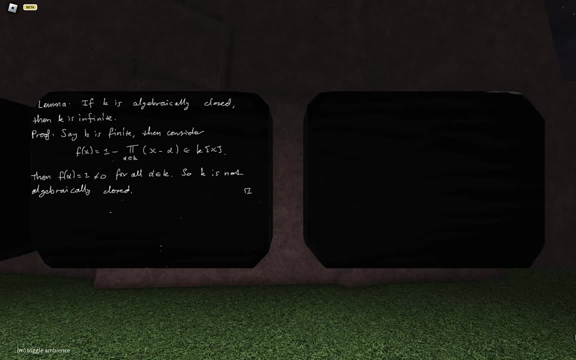 like. there's no way to sort of like. there's no way to sort of come up with an idea of a product over. come up with an idea of a product over. come up with an idea of a product over like, like, like. infinitely many elements of a field. 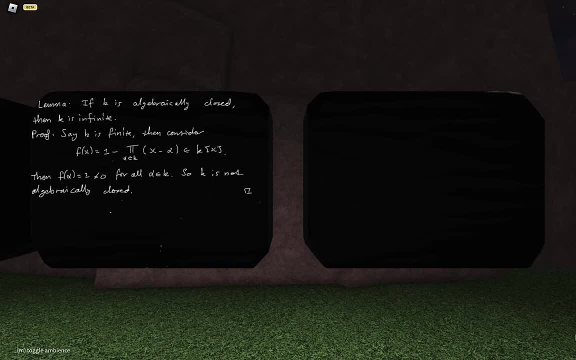 infinitely many elements of a field, infinitely many elements of a field. because, because, because then you could sort of like violate, then you could sort of like violate, then you could sort of like violate this theorem. i don't know if this, oh, do you buy this? i don't know if this, oh, do you buy this? 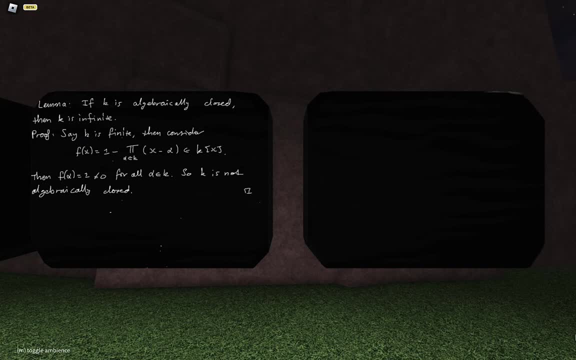 i don't know if this: oh, do you buy this theorem? do you just mean the lemma that i theorem? do you just mean the lemma that i theorem? do you just mean the lemma that i just did, just did, just did. dilemma, yeah, yeah, um, as in like you can't define. 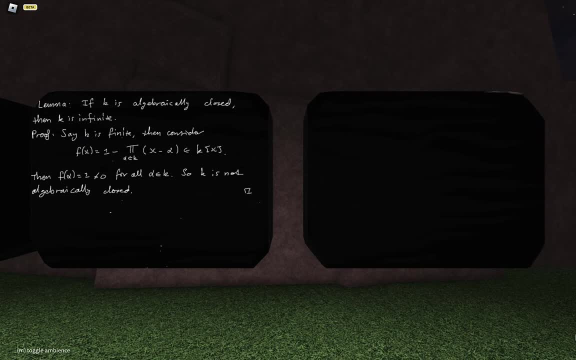 as in like you can't define. as in like you can't define. some thing with infinitely many inputs, some thing with infinitely many inputs, some thing with infinitely many inputs that sort of behaves like a product. that sort of behaves like a product. that sort of behaves like a product. word in that, if one of the things is: 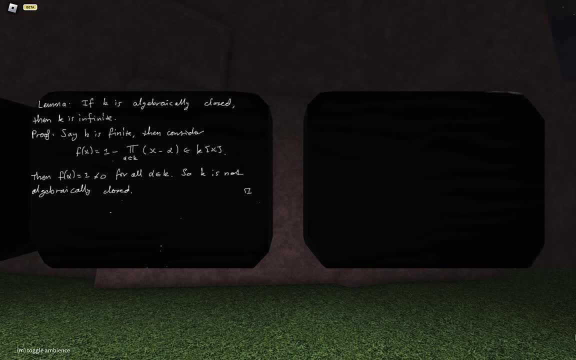 word in that if one of the things is. word in that if one of the things is zero, then the whole thing is zero, or zero, then the whole thing is zero, or zero, then the whole thing is zero, or something, something, something. yeah, i don't know if 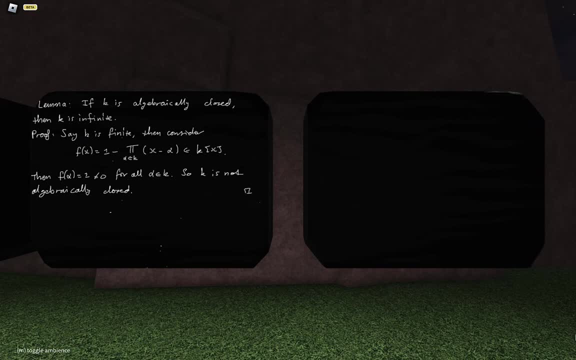 yeah, i don't know if. yeah, i don't know if that's that's. that's like the thing is the finiteness, like the thing is the finiteness, like the thing is the finiteness. assumption of polynomials and of assumption of polynomials and of. 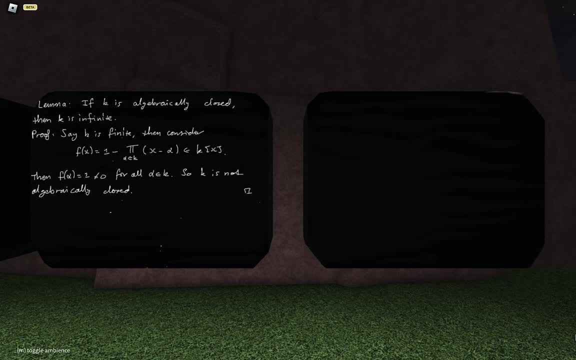 assumption of polynomials and of products inside groups and algebras etc. products inside groups and algebras etc. products inside groups and algebras etc. i mean they're certainly motivated by. i mean they're certainly motivated by. i mean they're certainly motivated by more than just the fact that you can't. 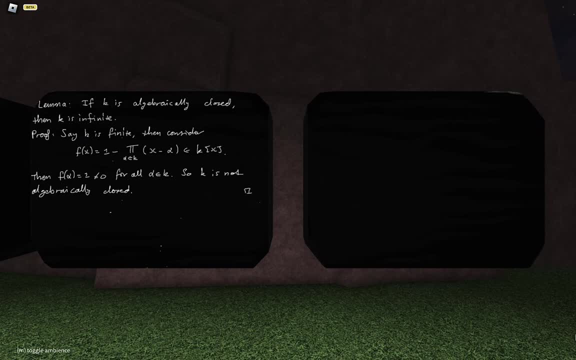 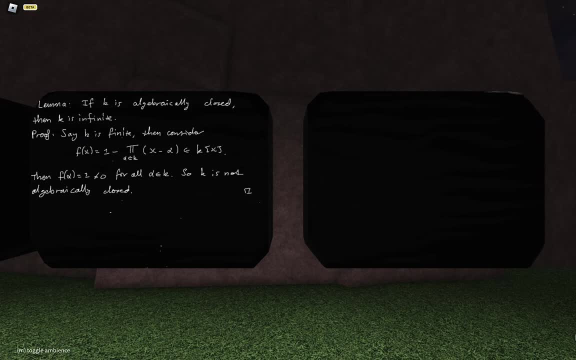 infinite sums out there, but we're infinite sums out there, but we're considering structures that don't do that, considering structures that don't do that, considering structures that don't do that. so so so, correct? i'm not sure. correct, i'm not sure. correct, i'm not sure. i guess, the idea of algebraically closed. 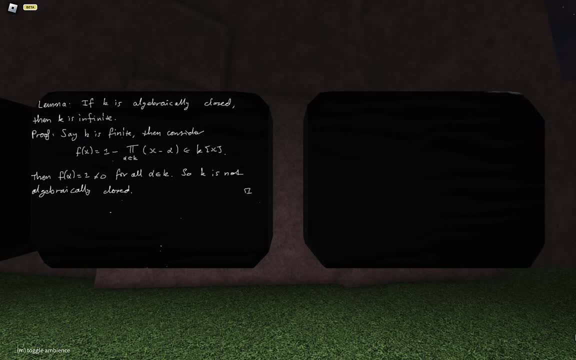 i guess the idea of algebraically closed, i guess the idea of algebraically closed has the finiteness baked into it like: has the finiteness baked into it like has the finiteness baked into it like? it's a question about. it's a question about 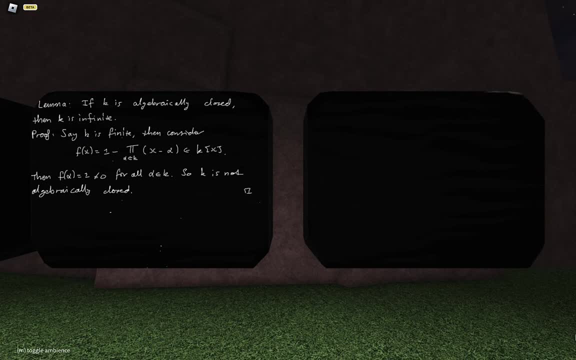 it's a question about, because it's a question about, because it's a question about, because it's a question about polynomials, yeah, yeah, polynomials, yeah, yeah, polynomials, yeah, yeah, okay, okay, okay. model of each infinite cardinality for. model of each infinite cardinality for. 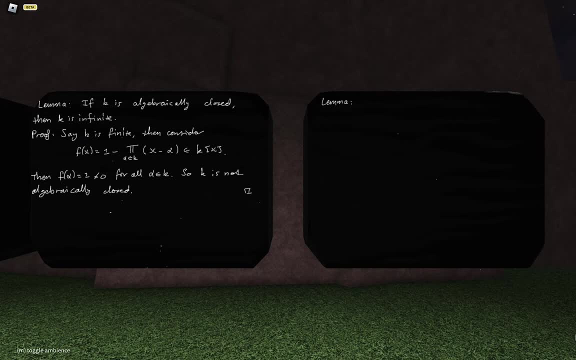 model of each infinite cardinality for algebraically closed fields. algebraically closed fields. algebraically closed fields. for this, i just need to get my hands a for this. i just need to get my hands a for this. i just need to get my hands a little bit dirty with. 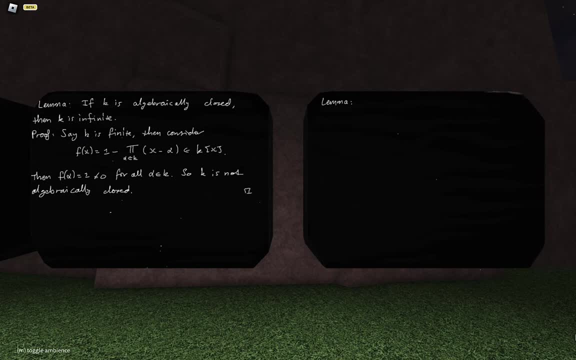 little bit dirty with little bit dirty with the uh canonical construction. the uh canonical construction, the uh canonical construction of an algebraically closed field, of an algebraically closed field, of an algebraically closed field, from a non algebraically closed field, from a non algebraically closed field. 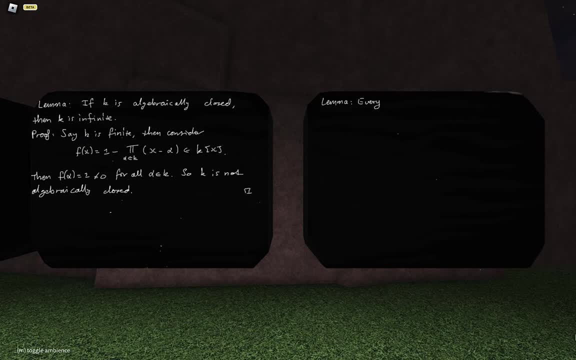 from a non algebraically closed field. so maybe, let me just remind you, so maybe, let me just remind you, so maybe, let me just remind you that every, every field, that every, every field, that every, every field f can be embedded into an algebraic, f can be embedded into an algebraic. 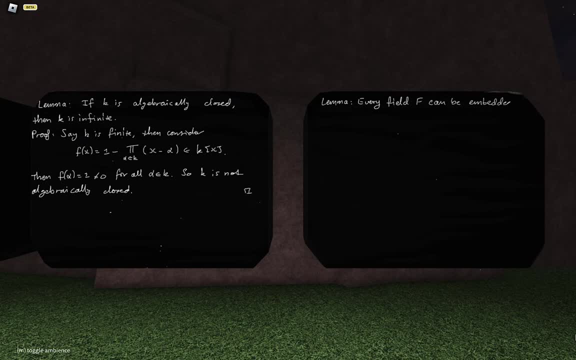 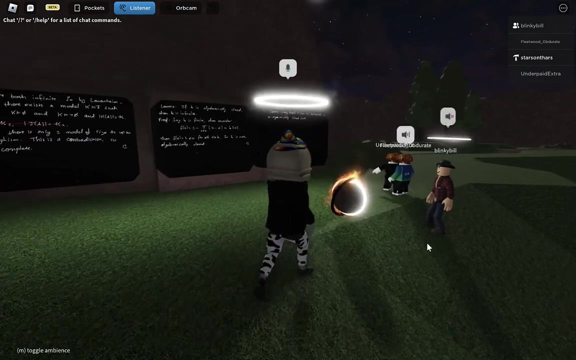 f can be embedded into an algebraic closed field. hey, have i lost sound, can you still hear? hey, have i lost sound, can you still hear? hey, have i lost sound. can you still hear me? yeah, i can hear you okay, thank you. yeah, i can hear you okay, thank you. 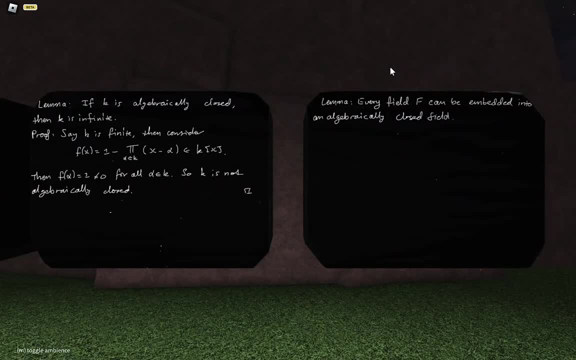 yeah, i can hear you okay. thank you, sorry, my headphones sounded strange and sorry, my headphones sounded strange and sorry. my headphones sounded strange and i was worried that i lost it. i was worried that i lost it. i was worried that i lost it. okay, um, okay um. 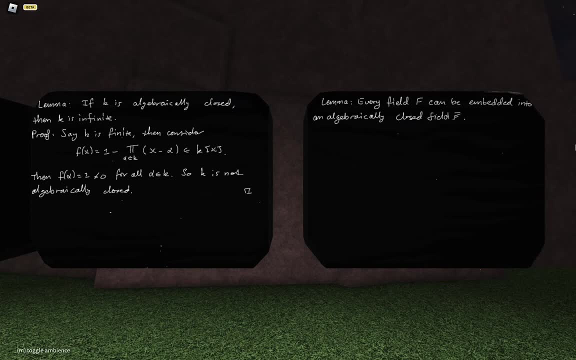 okay, um, if can be, if can be, if can be embedded into an algebraically closed, embedded into an algebraically closed, embedded into an algebraically closed field. i mean, only just pull that f bar field. i mean, only just pull that f bar field. i mean only just pull that f bar. and 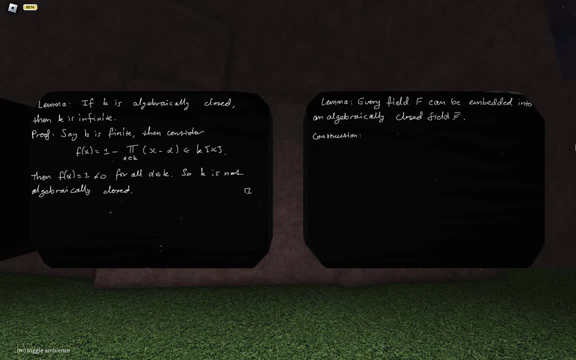 and and the construction is like this, so is like this, so is like this, so for every monic, for every monic, for every monic, irreducible f, f, f, inside, inside, inside, f of x, f of x, f of x. we introduce formal indeterminates. 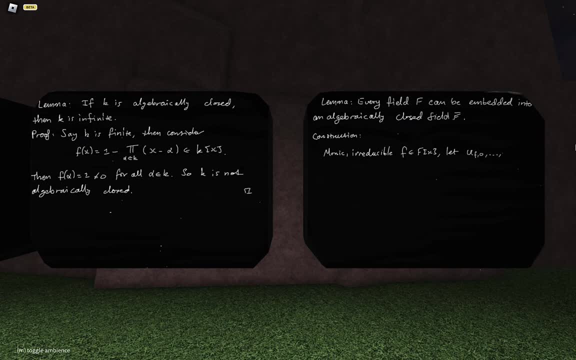 we introduce formal indeterminates. we introduce formal indeterminates necessarily finitely. many of them necessarily finitely, many of them necessarily finitely, many of them so. so so u sub f dot dot dot u. u sub f dot dot dot u. u sub f dot dot dot u sub f d. 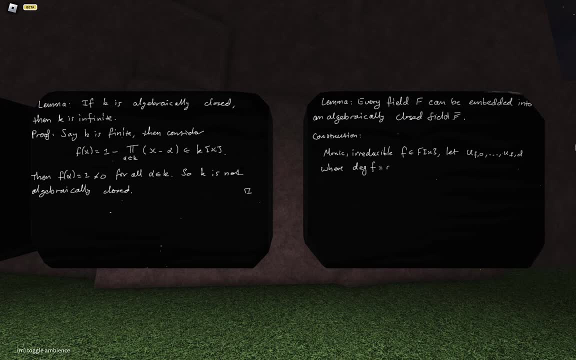 sub f d. sub f d, where, where, where the degree, the degree, the degree of f equals d right, so of f equals d right, so of f equals d right. so for each monic irreducible polynomial i. for each monic irreducible polynomial i. for each monic irreducible polynomial i, introduce d plus one. 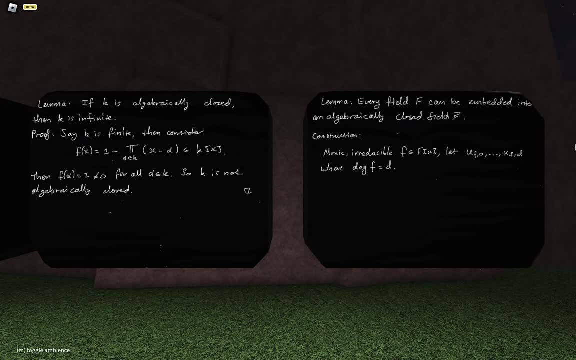 introduce d plus one. introduce d plus one. is it d plus one? yeah, d plus one. is it d plus one? yeah, d plus one. is it d plus one? yeah, d plus one. indeterminates, indeterminates, indeterminates, where d is the degree of f. 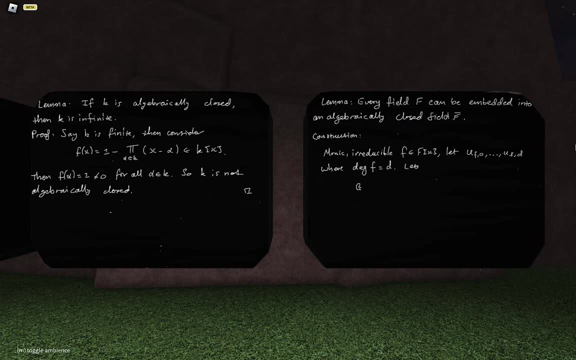 where d is the degree of f, where d is the degree of f. and then i define, and then i define, and then i define this, this, this: u f zero, yeah. so u f zero, yeah, so u f zero, yeah. so each u has a pair of subscripts. 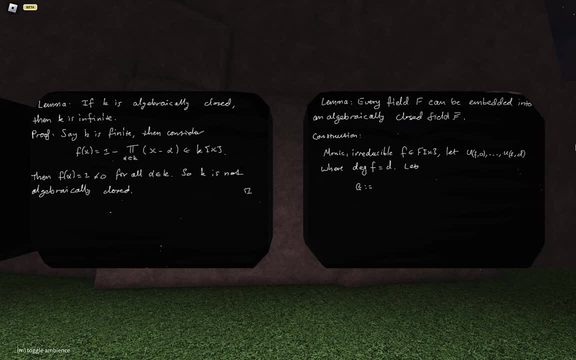 each? u has a pair of subscripts. each? u has a pair of subscripts: u sub f zero up to u sub fd. u sub f zero up to u sub fd. u sub f zero up to u sub fd. and what are they? they're just two. 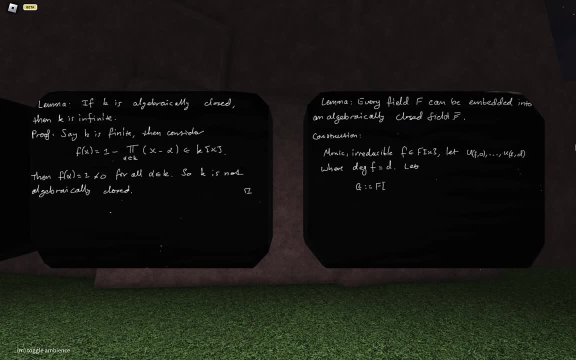 and what are they? they're just two. and what are they? they're just two variables. or what formal symbols? yeah, variables. or what formal symbols? yeah, variables. or what formal symbols? yeah, these are going to, these are going to, these are going to be indeterminates inside of the 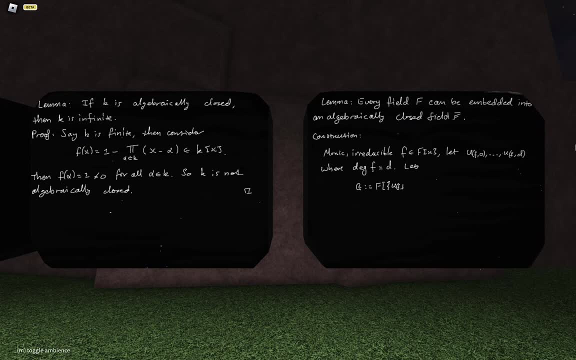 be indeterminates inside of the be indeterminates inside of the polynomial ring. and i'm just about to polynomial ring and i'm just about to polynomial ring and i'm just about to write down, so i'll let g be the polynomial ring over all of these. 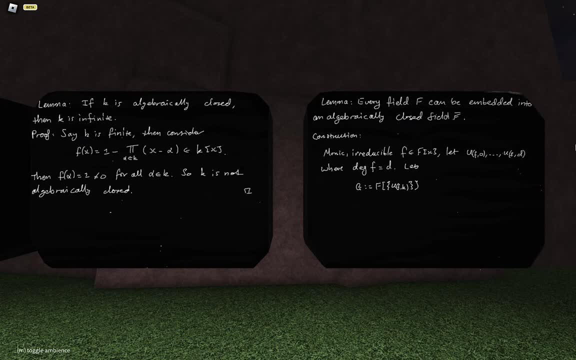 the polynomial ring over all of these, the polynomial ring over all of these indeterminates, indeterminates, indeterminates with base field f, with base field f, with base field f, and then and then and then. the clever, the clever, the clever, trick, trick trick is you write f. 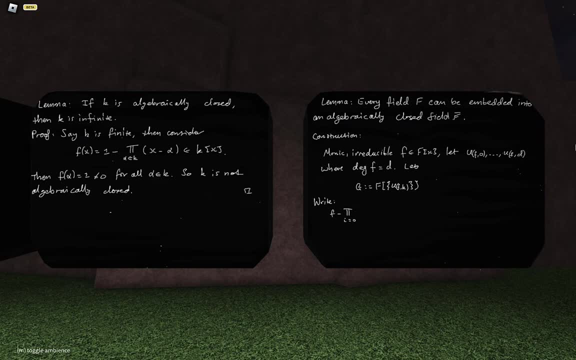 is you write f, is you write f minus, minus minus the product, the product, the product of all of these corresponding to f. so of all of these corresponding to f, so of all of these corresponding to f. so this is x minus u, this is x minus u. 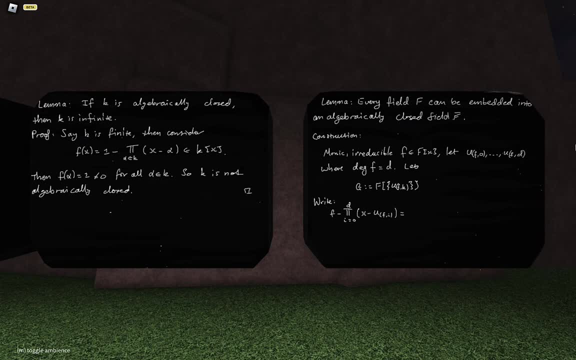 this is x minus u, sub f, i, sub f, i, sub f, i and and and yeah, yeah, yeah. g equals f of this set of form. g equals f of this set of form. g equals f of this set of form. more symbols, more symbols, more symbols. is that set? 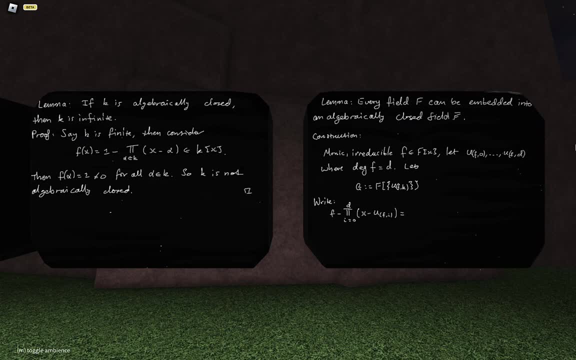 is that set? is that set also like ranging over all f, or is it also like ranging over all f? or is it also like ranging over all f, or is it? this is fixed. this is fixed. this is fixed. it's ranging over all f. it's ranging over all f. 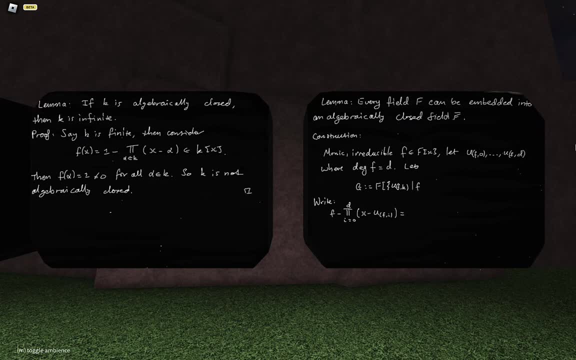 it's ranging over all f. okay, okay, okay, and then and then and then. now you're now. you're now. you're below here you're fixing f again. or below here you're fixing f again. or below here you're fixing f again, or yeah, yeah, yeah, yeah. 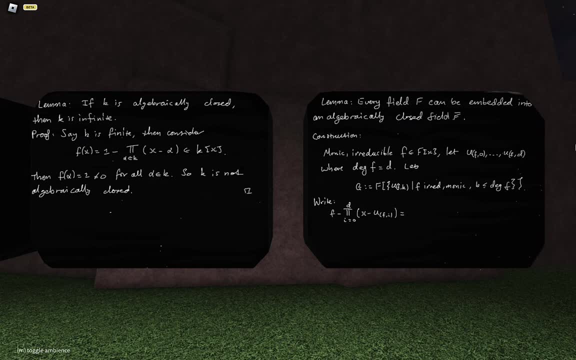 okay, so then for each. okay, so then for each. okay, so then for each, for each of these, for each of these, for each of these. uh, uh, uh uh. monica, irreducible polynomials. i take f. monica, irreducible polynomials. i take f. monica, irreducible polynomials. i take f minus this product. 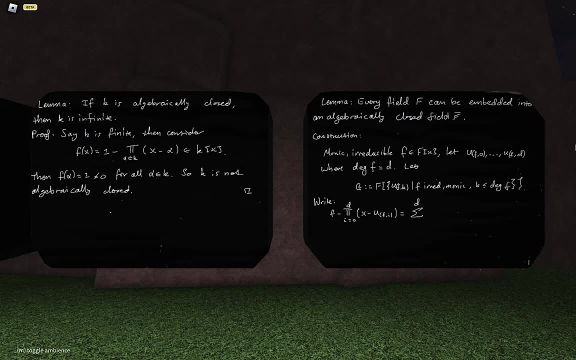 minus this product, minus this product, and i expand that out right, and and i expand that out right, and, and i expand that out right, and i'm going to end up with some, i'm going to end up with some, i'm going to end up with some sum that looks like this: 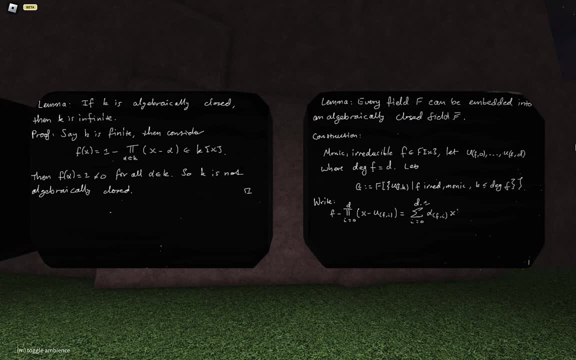 sum that looks like this. sum that looks like this: where i have alpha sub f i multiplied by where i have alpha sub f, i multiplied by where i have alpha sub f i multiplied by x to the i, and this is an element of x to the i, and this is an element of. 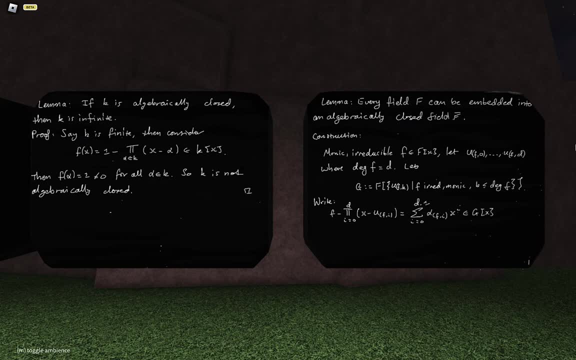 x to the i and this is an element of g as the base ring, g as the base ring, g as the base ring, um in a polynomial ring right, so um in a polynomial ring right, so um in a polynomial ring right. so we work inside this polynomial ring. i can. 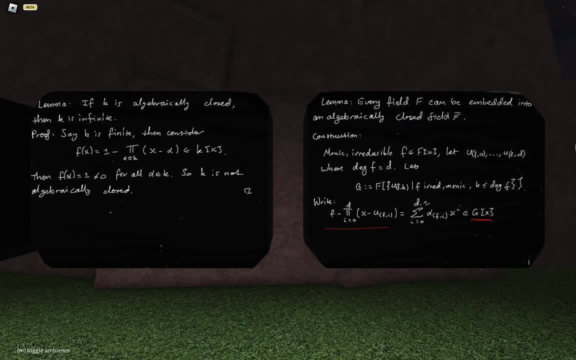 we work inside this polynomial ring. i can we work inside this polynomial ring, i can construct this polynomial and i just construct this polynomial and i just construct this polynomial and i just do the massive expansion of the big, do the massive expansion of the big, do the massive expansion of the big product and simplify everything and i 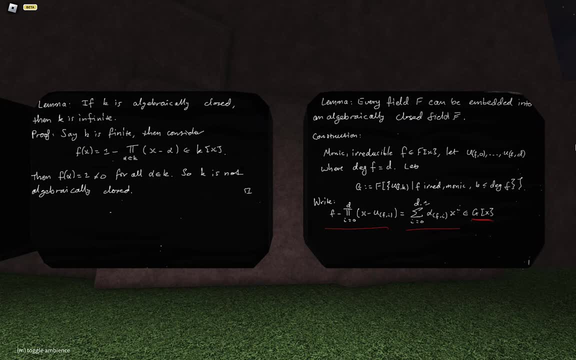 product and simplify everything, and i product and simplify everything, and i ended up with, ended up with, ended up with some some some polynomial over x, with polynomial over x, with polynomial over x, with uh coefficients inside g, and then i uh coefficients inside g, and then i uh coefficients inside g, and then i take all of those coefficients. 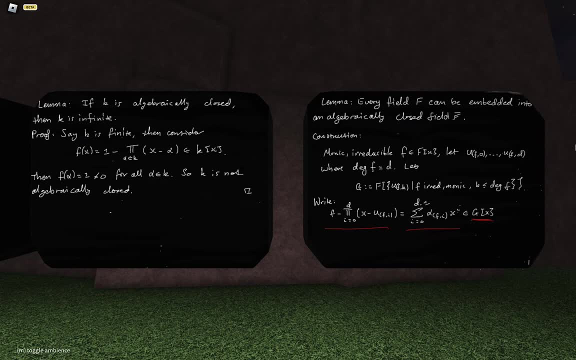 take all of those coefficients. take all of those coefficients- alpha fi, and i'm mod out by all of alpha fi and i'm mod out by all of alpha fi and i'm mod out by all of those, and so you can see what i'm doing. those, and so you can see what i'm doing. 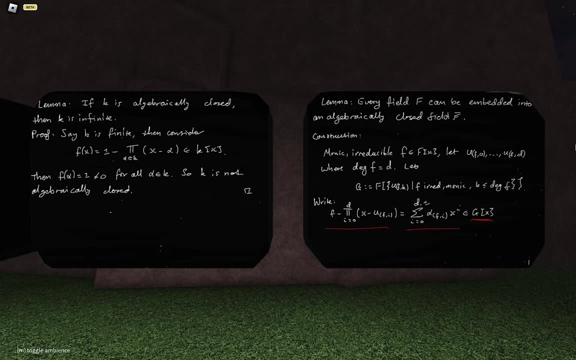 those, and so you can see what i'm doing is i'm forcing this, is i'm forcing this, is i'm forcing this difference of polynomials to be zero, difference of polynomials to be zero, difference of polynomials to be zero, which means i've introduced a. 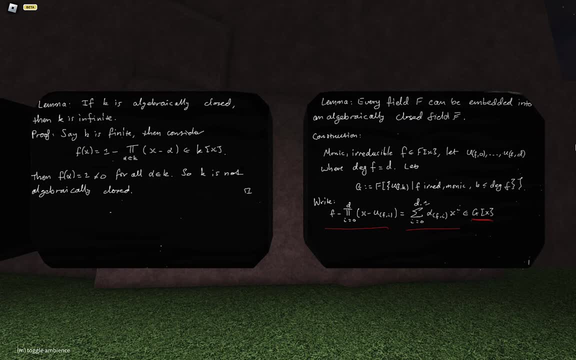 which means i've introduced a, which means i've introduced a factorization of f which wasn't there. factorization of f which wasn't there. factorization of f which wasn't there earlier, earlier, earlier, right, right, right. so i'm constructing an algebraically. so i'm constructing an algebraically. 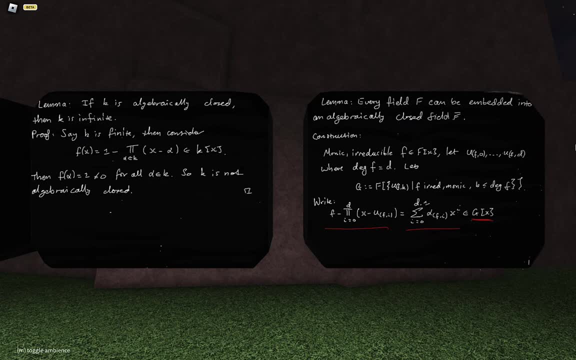 so i'm constructing an algebraically closed field: closed field, closed field. okay so, okay, so, okay. so the point is the, the ideal, the ideal, the ideal i, the ideal i, the ideal i, generated by all, generated by all, generated by all. alpha f i. alpha f i. 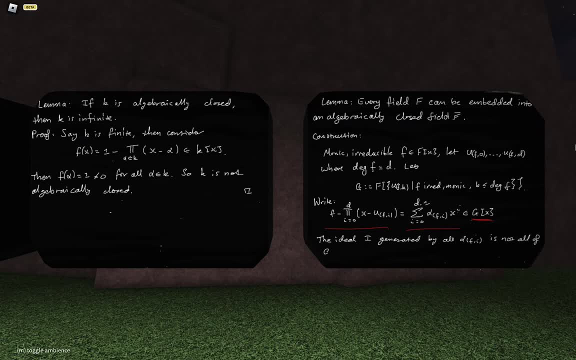 alpha f, i is not, is not, is not all of g, so it's contained in a maximal ideal, and so it's contained in a maximal ideal. and so it's contained in a maximal ideal, and that's using zorn's lemma. that's using zorn's lemma. 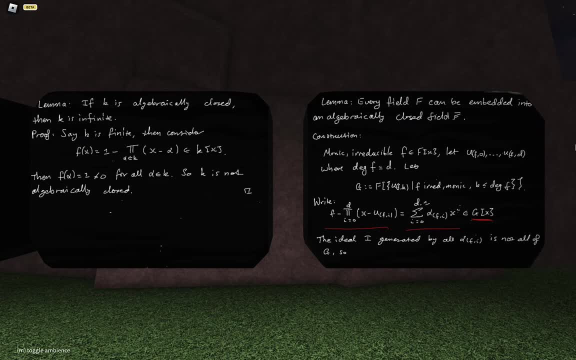 that's using zorn's lemma, so i've, i've just used, so i've, i've just used, so i've, i've just used zfc, um, zfc, um zfc, um. i've used choice in zfc. i'm trying to. i've used choice in zfc. i'm trying to. 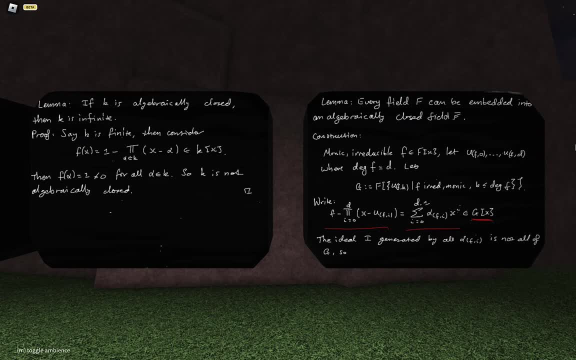 i've used choice in zfc. i'm trying to think if i'm using it in the meta theory. think if i'm using it in the meta theory. think if i'm using it in the meta theory or in the theory because this is inside, or in the theory because this is inside. 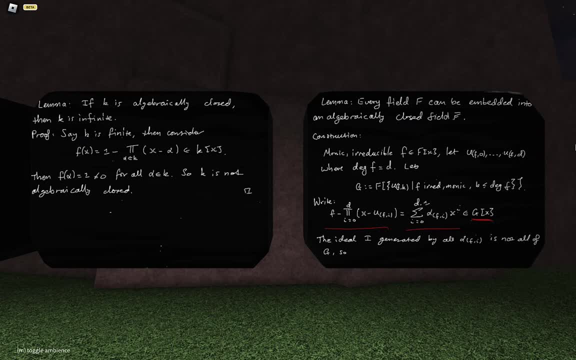 or in the theory, because this is inside a model, so i'm using it inside z of c, a model. so i'm using it inside z of c, a model, so i'm using it inside z of c. so that's fine, so that's fine, so that's fine, okay. 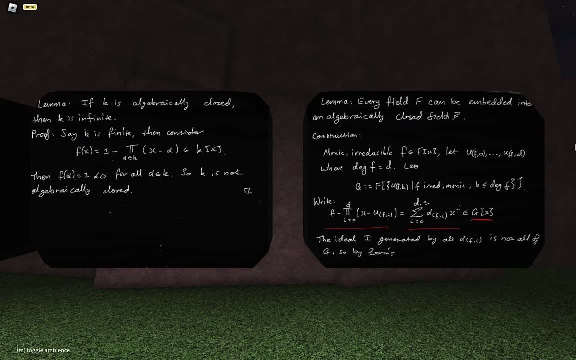 okay, okay, this is all g. so this is all g. so this is all g. so by by, by zorn's lemma: i is a subset of m with m. i is a subset of m with m. i is a subset of m with m maximal. okay, i need to move to the next board. 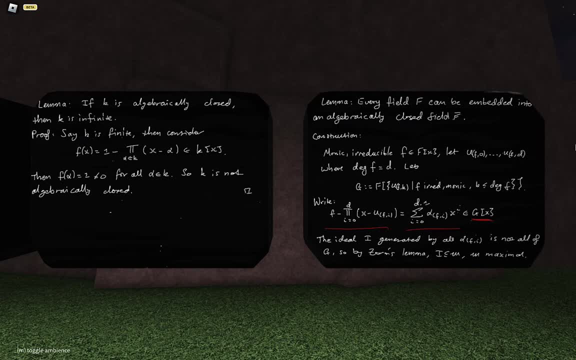 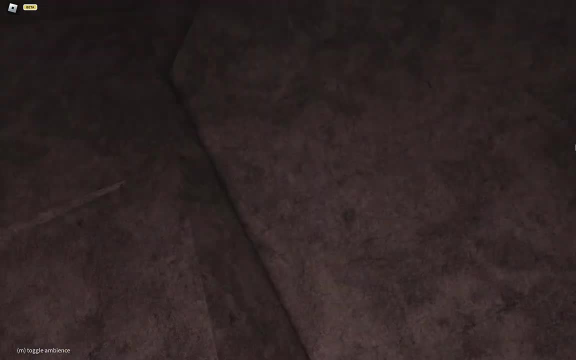 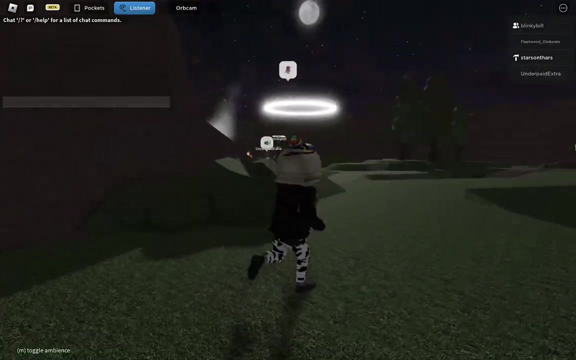 okay, i need to move to the next board. okay, i need to move to the next board, okay. and so then, what i do is i define okay. and so then, what i do is i define okay. and so then, what i do is i define f1, f1. 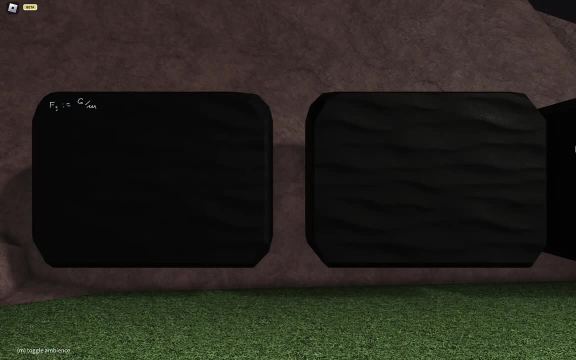 f1 to be equal to g, modded out by the. to be equal to g, modded out by the. to be equal to g, modded out by the maximal ideal m. maximal ideal m. maximal ideal m. okay, okay, okay and okay and okay, and that that. 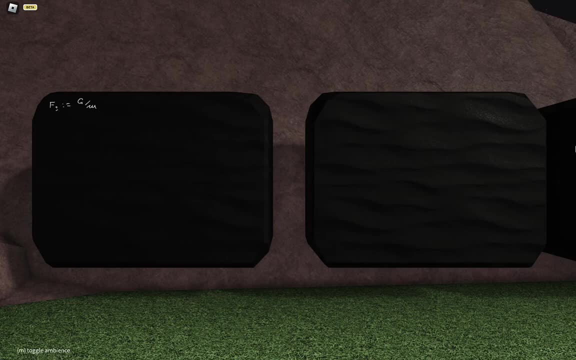 that is going to give me a new field, because i've modded out by a field, because i've modded out by a field, because i've modded out by a maximal ideal, maximal ideal, maximal ideal. so that's a field but i've introduced. so that's a field, but i've introduced. 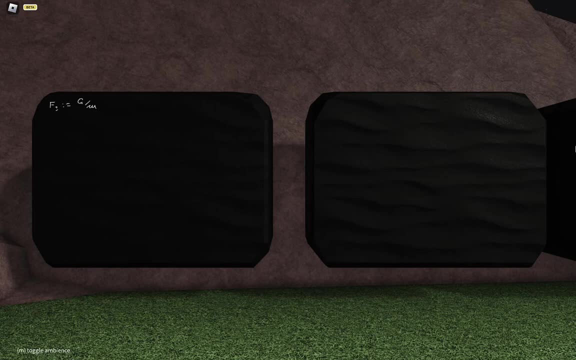 so that's a field. but i've introduced new indeterminants, so there might now be new indeterminants. so there might now be new indeterminants. so there might now be new monic irreducible polynomials inside. new monic irreducible polynomials inside. 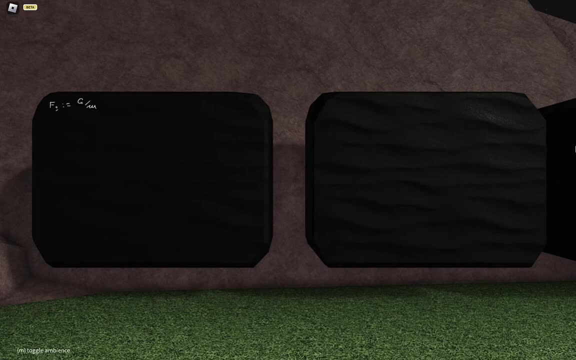 new monic: irreducible polynomials inside f1 and i need f1, and i need f1 and i need uh algebraic closure, i need uh algebraic closure. i need uh algebraic closure. i need factorizations of those, factorizations of those, factorizations of those as well. okay, so i need to repeat this. 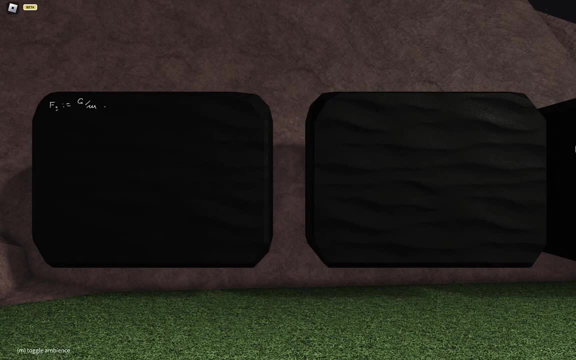 as well. okay, so i need to repeat this as well. okay, so i need to repeat this process in order to define process, in order to define process, in order to define f? j for all j in elements of the natural. f? j for all- j in elements of the natural. 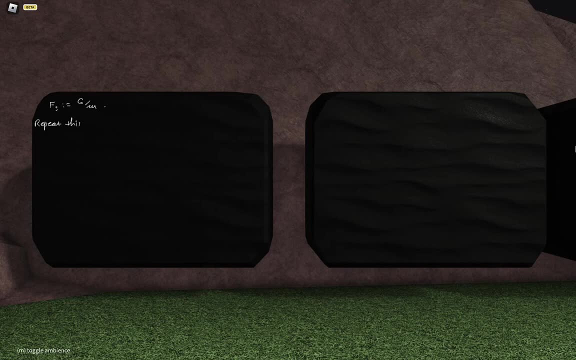 f j for all j in elements of the natural numbers to obtain for all j greater than zero, and then for all j greater than zero, and then for all j greater than zero, and then define, define, define f bar to be equal to in the union. f bar to be equal to in the union. 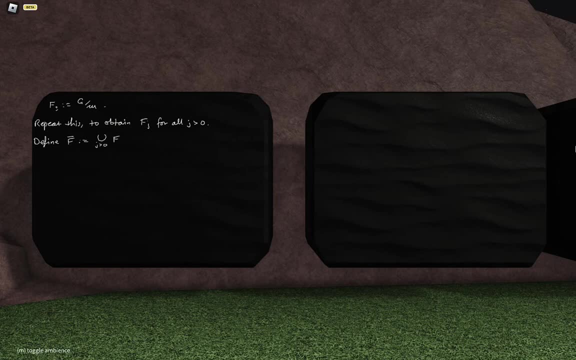 f bar to be equal to in the union of all j greater than zero of all j greater than zero of all j greater than zero, f j, f, j, f, j. okay then, okay then, okay then, f bar, f bar. f bar is algebraically closed and f. 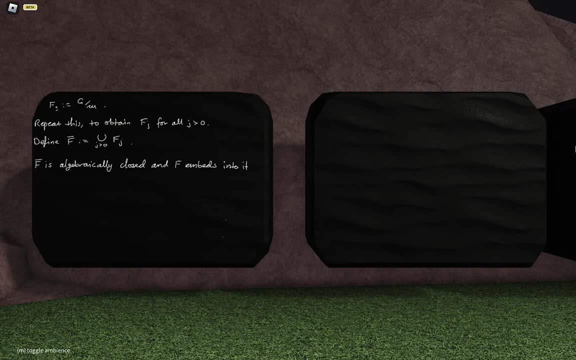 and f and f embeds into it, embeds into it, embeds into it. okay, so that's the proof of the lemma. okay, so that's the proof of the lemma. okay, so that's the proof of the lemma. that's just the standard construction of. that's just the standard construction of. 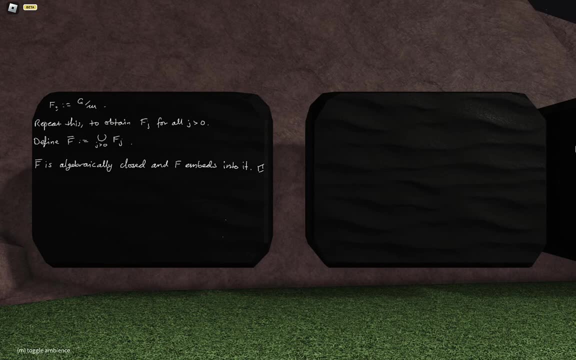 that's just the standard construction of the algebraic closure of a field. but the algebraic closure of a field, but the algebraic closure of a field. but the reason why i wrote it out again is the reason why i wrote it out again is the reason why i wrote it out again is because i need to look at this and 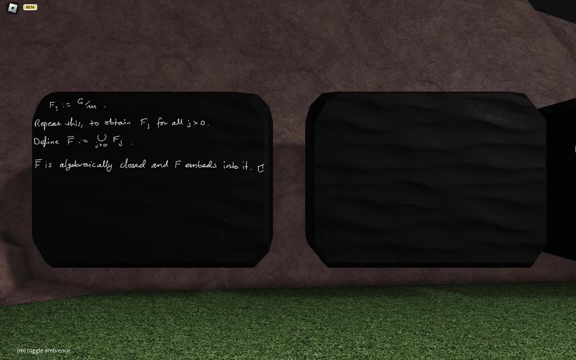 because i need to look at this and because i need to look at this and observe that the cardinality of the observe, that the cardinality of the observe, that the cardinality of the algebraic closure of a field is algebraic closure of a field is. 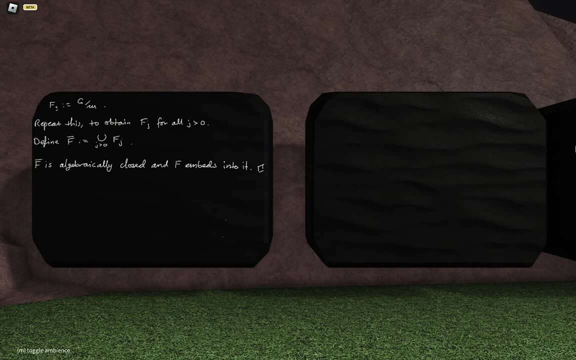 algebraic closure of a field is uncountably infinite if the original uncountably infinite. if the original uncountably infinite, if the original field was finite and it's of cardinality field was finite and it's of cardinality field was finite and it's of cardinality kappa if the original field is of. 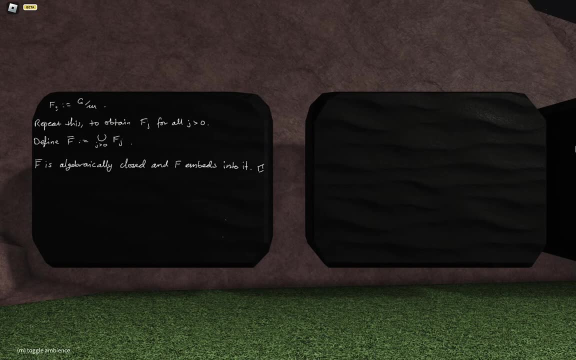 kappa. if the original field is of kappa, if the original field is of cardinality, kappa, cardinality, kappa, cardinality, kappa. so the crucial argument for that, i would so the crucial argument for that, i would so the crucial argument for that. i would really like to point to something that's 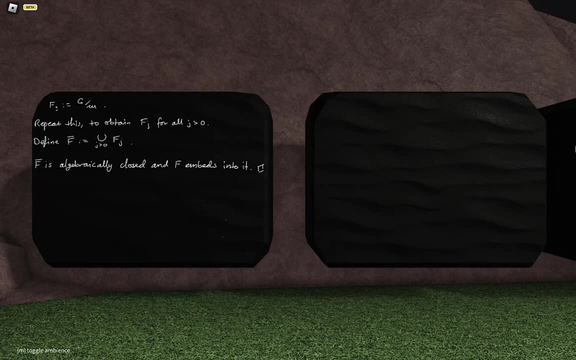 really like to point to something. that's really like to point to something that's on the previous board. that's a shame on the previous board. that's a shame on the previous board. that's a shame. whatever is that. whatever is that. whatever is that? i add indeterminates. 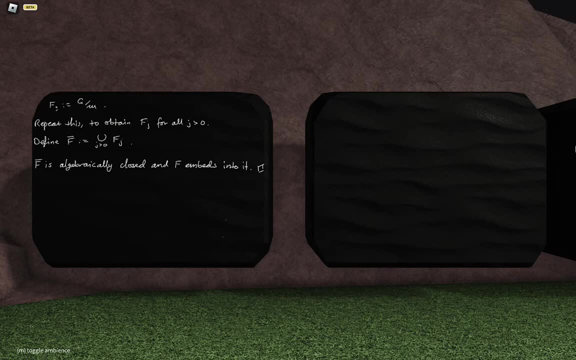 i add indeterminates. i add indeterminates. why is it uncountable if f was? why is it uncountable if f was? why is it uncountable if f was finite, finite, finite? because, because, because i have, i have, i have introduced, introduced. 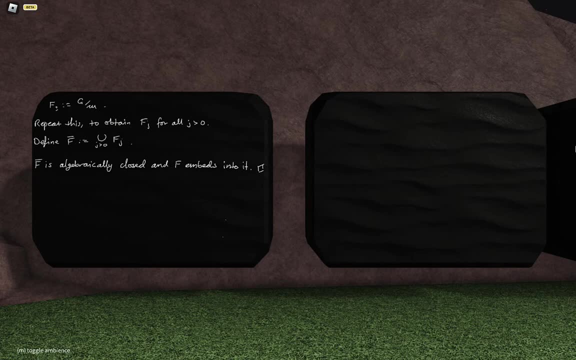 introduced polynomials over a finite field and as polynomials over a finite field and as polynomials over a finite field. and as soon as you do that, you end up with an. soon as you do that you end up with an. soon as you do that, you end up with an uncountable set. 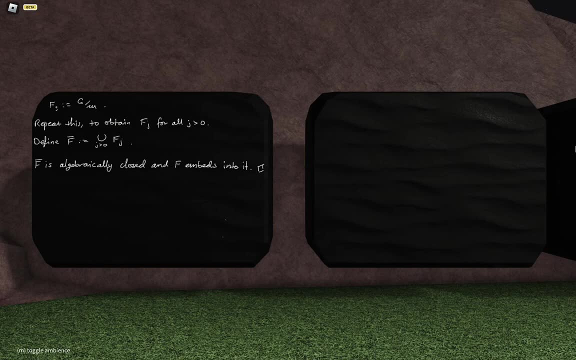 uncountable set. uncountable set. can you see that? because can you see that? because can you see that? because a, a a polynomial could be, polynomial, could be, polynomial, could be how it could have arbitrary degree, how it could have arbitrary degree, how it could have arbitrary degree, and so 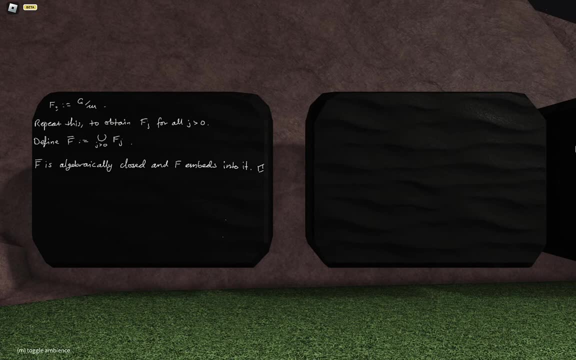 and so, and so all polynomials look like all polynomials, look like all polynomials. look like: coefficients plus coefficient times x. coefficients plus coefficient times x. coefficients plus coefficient times x plus coefficient plus coefficient times x plus coefficient times x. squared plus dot plus coefficient. squared plus dot plus coefficient. 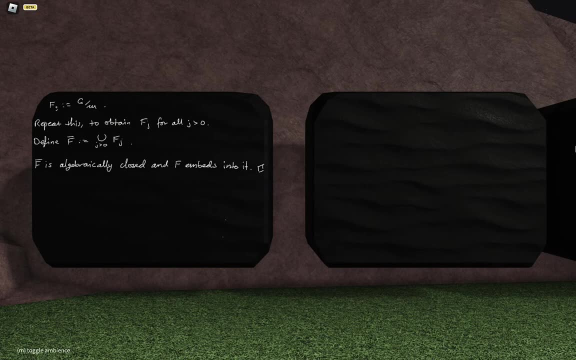 squared plus dot, plus coefficient, times x to the n, times x to the n, times x to the n, and so and so, and so i'm looking at the set, i'm looking at the set, i'm looking at the set of of, of sequences of length n. 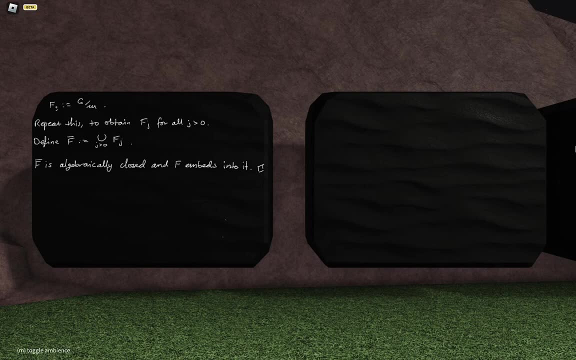 sequences of length n. sequences of length n where each element is an element of, where each element is an element of, where each element is an element of the finite field, and n is ranging over all the finite field, and n is ranging over all the finite field and n is ranging over all natural numbers. 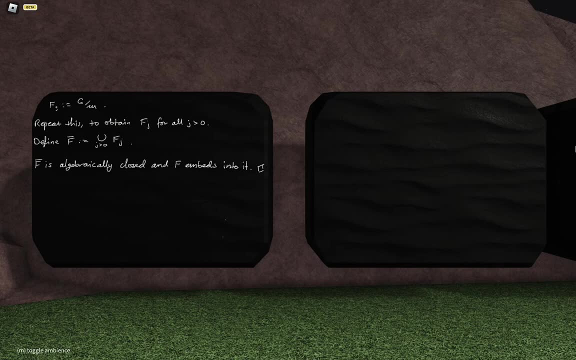 natural numbers, natural numbers. that set, that set, that set is uncountably- sorry, it's countably- is uncountably infinite. well, what did i say infinite? well, what did i say infinite? well, what did i say? uncountably infinite, uncountably infinite, uncountably infinite. oh okay, sorry, that was a slip of the. 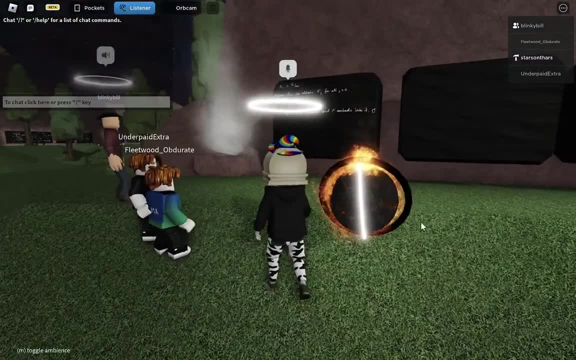 oh okay, sorry, that was a slip of the. oh okay, sorry, that was a slip of the tongue. it's countably infinite tongue. it's countably infinite tongue. it's countably infinite. we were both sitting there like that. we were both sitting there like that. we were both sitting there like that sounds countable to me. 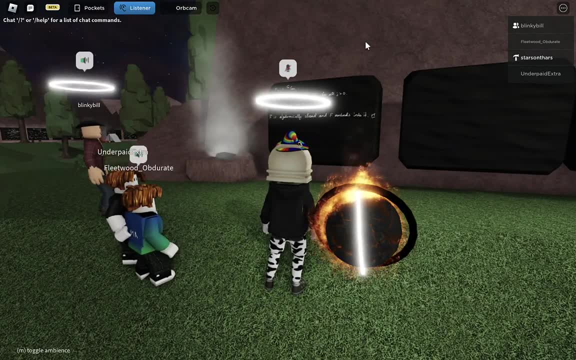 sounds countable to me. sounds countable to me. yeah, it's like just gave you the most. yeah, it's like just gave you the most. yeah, it's like just gave you the most. telling me mathematical proof of nerd. telling me mathematical proof of nerd. telling me mathematical proof of nerd. some pretty funny exercise to give a. 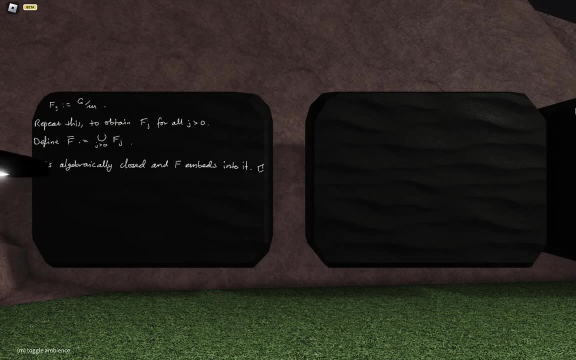 some pretty funny exercise to give a. some pretty funny exercise to give a proof of the statement. you're exactly proof of the statement. you're exactly proof of the statement. you're exactly trying not to trying, not to trying, not to. well, you haven't stated okay, so yeah. 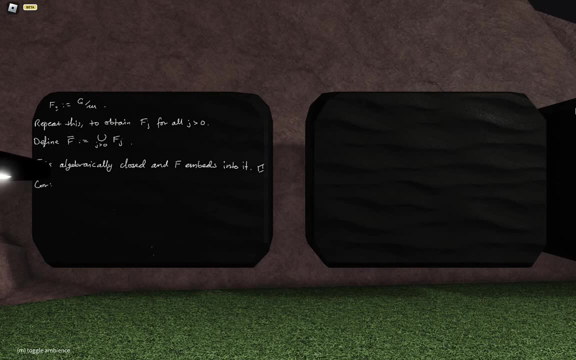 well, you haven't stated okay, so yeah. well, you haven't stated okay, so yeah, sorry, it's countably infinite. if f is sorry, it's countably infinite. if f is sorry, it's countably infinite. if f is finite, finite, finite. so that's the next corollary. 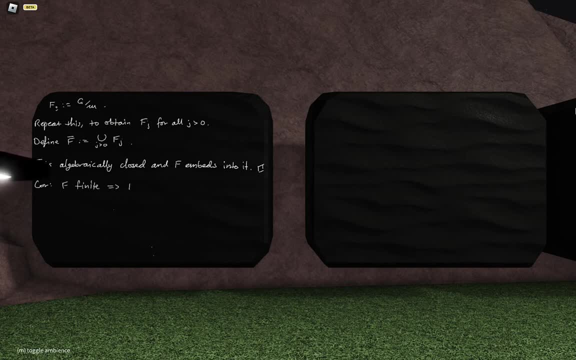 so that's the next corollary. so that's the next corollary: f, f, f. finite implies f bar. finite implies f bar. finite implies f bar is countably infinite and the magnitude of f equaling kappa and the magnitude of f equaling kappa. 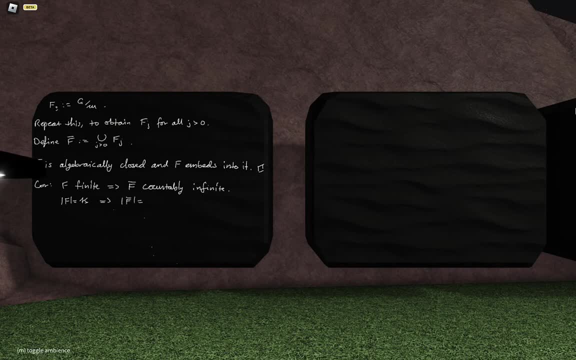 and the magnitude of f equaling kappa implies that the magnitude of f implies that the magnitude of f implies that the magnitude of f is is is. f bar is also kappa, f bar is also kappa, f bar is also kappa. okay, and it's the same argument for both. 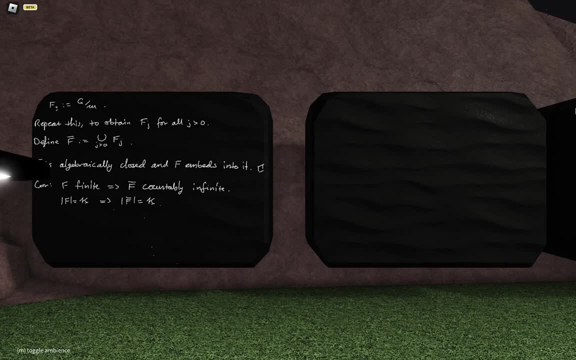 okay, and it's the same argument for both. okay, and it's the same argument for both of them, of them, of them. so you're taking polynomials over a, so you're taking polynomials over a. so you're taking polynomials over a field, field, field, and this is called kappa, at least, 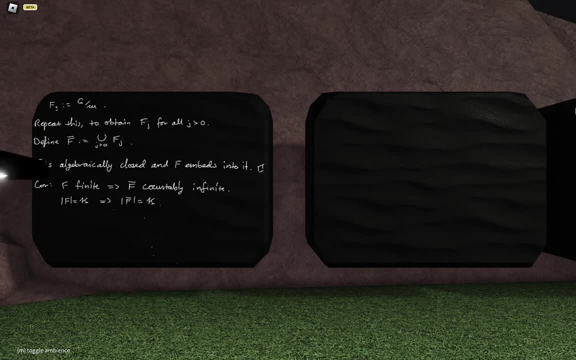 and this is called kappa at least, and this is called kappa at least. countable, countably infinite right. countable, countably infinite right. countable, countably infinite right. yeah, good, good, good, good, okay, okay, okay, okay. so now we can do the final lemma of the entire theorem. 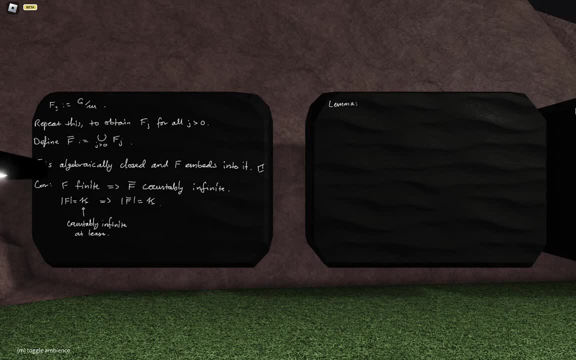 so, lemma, let p be either prime or zero. let's, let's. kappa be greater than, or equal to kappa be greater than or equal to kappa be greater than or equal to lf, lf, lf, one. i guess that's so stupid to say, okay, let one. i guess that's so stupid to say, okay, let. 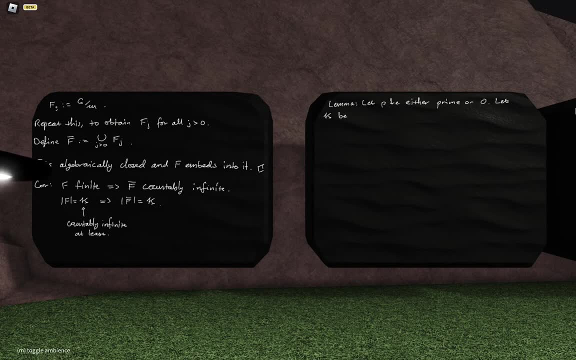 one. i guess that's so stupid to say, okay, let kappa be uncountable. oh, how do i say that i don't be uncountable? oh, how do i say that i don't be uncountable? oh, how do i say that i don't want to like assume? 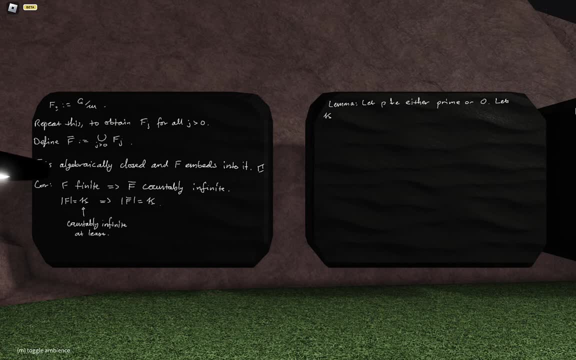 want to like assume, want to like assume continuum or something. let kappa continuum or something. let kappa continuum or something. let kappa be the cardinality of the real numbers, of the real numbers, of the real numbers. okay then, oh actually i don't know how to do that. 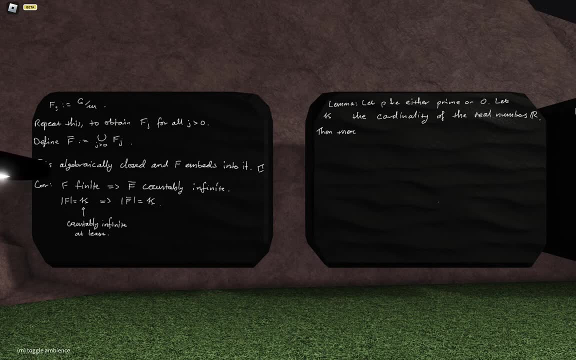 okay, let me sorry the statements have. okay, let me sorry the statements have. okay, let me sorry, the statements have been awkward because i don't know been awkward because i don't know been awkward because i don't know. i don't want to like get into lf. 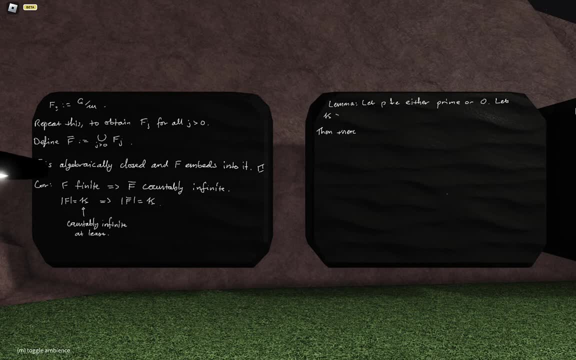 i don't want to like get into lf. i don't want to like get into lf one and lf zero and stuff, but i can say one and lf zero and stuff, but i can say one and lf zero and stuff. but i can say let kappa be greater than lf. 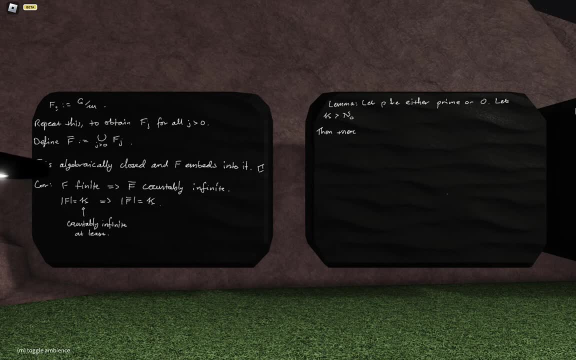 let kappa be greater than lf. let kappa be greater than lf. null, and i'll leave it there. null, and i'll leave it there. null, and i'll leave it there. okay, and the statement is, and the statement is, and the statement is: there exists- uh, there exists exactly one algebraically: 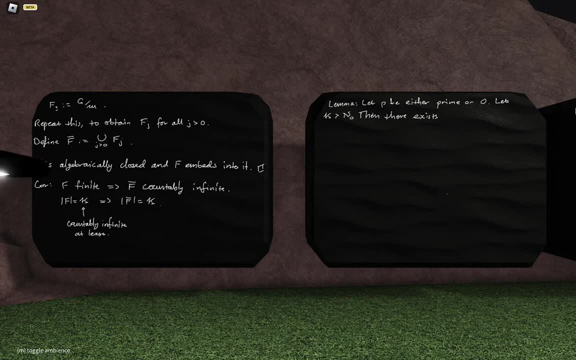 uh, there exists exactly one algebraically. uh, there exists exactly one algebraically. closed field of characteristic p. closed field of characteristic p. closed field of characteristic p. his cardinality is kappa up to his cardinality is kappa up to his cardinality is kappa up to isomorphism. 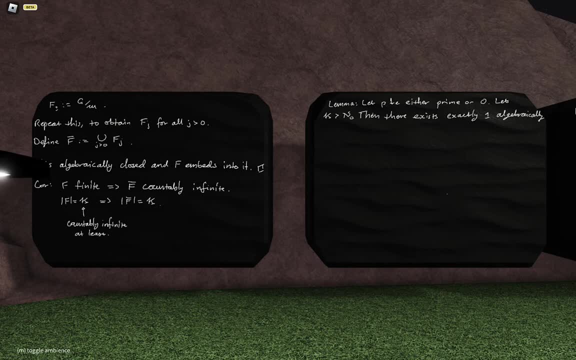 isomorphism, isomorphism. this is the premise of the washboard. this is the premise of the washboard. this is the premise of the washboard test, test test. exactly, yeah, so this is dot point three. okay proof, so, okay proof, so, okay proof. so first i'll take a particular choice of: 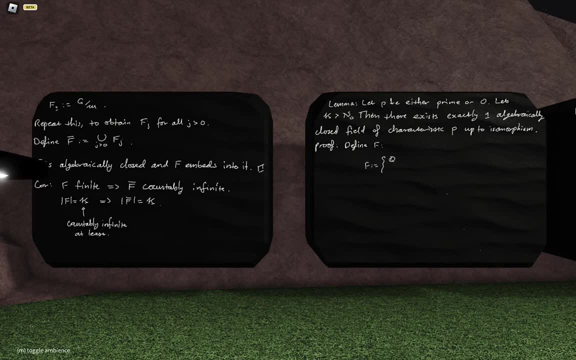 first, i'll take a particular choice of: first, i'll take a particular choice of base field, base field, base field. so i'm going to define it to be so i'm going to define it to be. so i'm going to define it to be the rational numbers. if p is equal to: 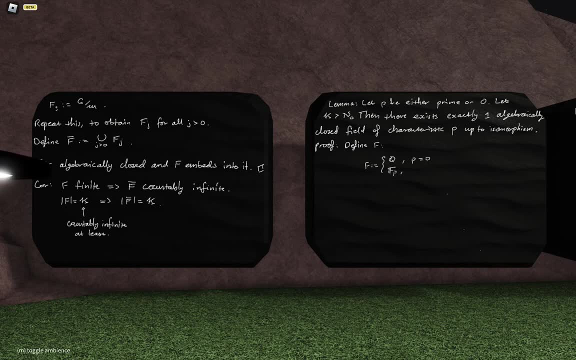 the rational numbers, if p is equal to the rational numbers, if p is equal to zero, zero, zero. and the field with p elements and the field with p elements and the field with p elements. so if a finite field of characteristic p, so if a finite field of characteristic p. 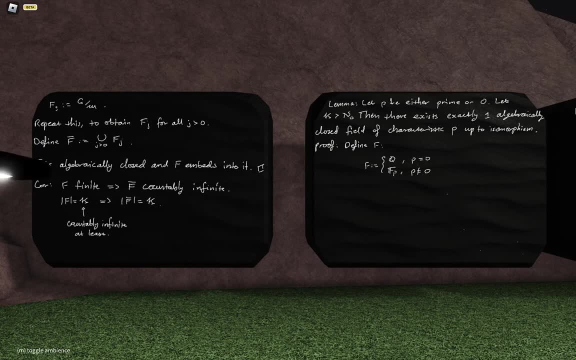 so if a finite field of characteristic p, if p is not equal to zero, if p is not equal to zero, if p is not equal to zero, and then let s, and then let s, and then let s. yeah, this is kind of hacking again this. yeah, this is kind of hacking again this. 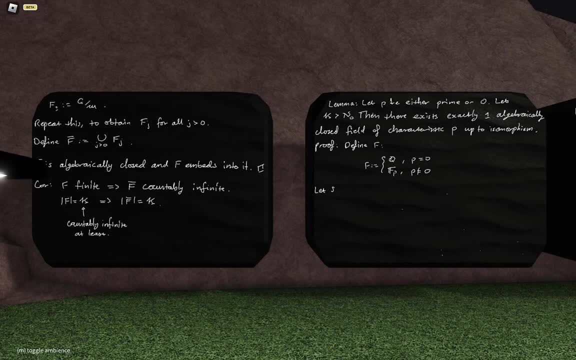 yeah, this is kind of hacking again. this is actually a very similar argument to. is actually a very similar argument to. is actually a very similar argument to what i did in the proof of the, what i did in the proof of the, what i did in the proof of the watch vote test. so i'm going to introduce 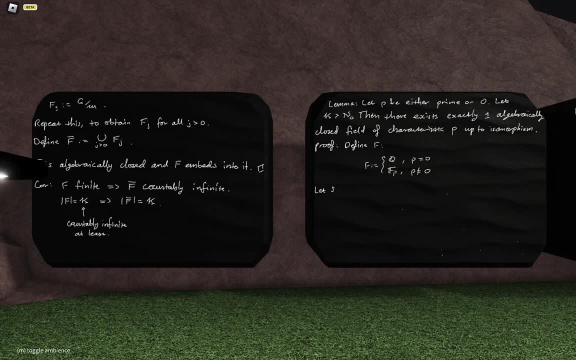 watch vote test. so i'm going to introduce watch vote test. so i'm going to introduce a collection of indeterminants, a collection of indeterminants, a collection of indeterminants parameterized by a set of cardinality, parameterized by a set of cardinality. 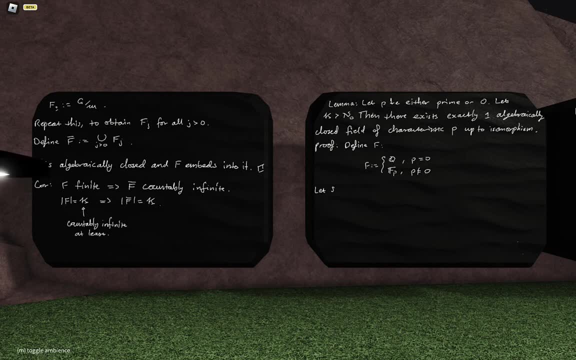 parameterized by a set of cardinality. kappa, kappa, kappa, right, and then i'm going to take the right, and then i'm going to take the right, and then i'm going to take the field of fractions, field of fractions, field of fractions of the polynomial room. in those 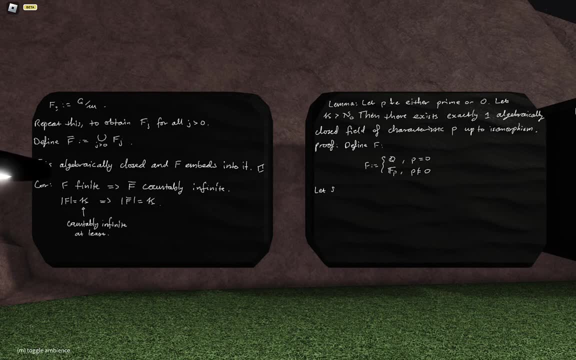 of the polynomial room, in those of the polynomial room, in those interminants over the field f, and then interminants over the field f, and then interminants over the field f, and then take the algebraic closure of that. so take the algebraic closure of that. so 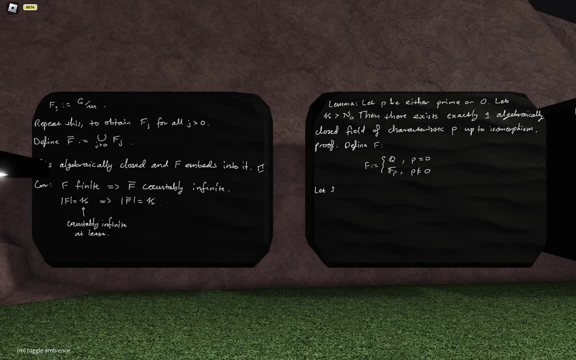 take the algebraic closure of that. so that's the existence and then uniqueness. that's the existence and then uniqueness. that's the existence, and then uniqueness follows from the universal property of, follows from the universal property of, follows from the universal property of algebraic closure. algebraic closure. 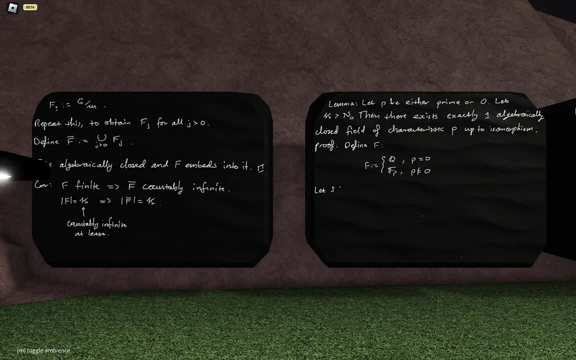 algebraic closure. so it's pretty simple and a little bit. so it's pretty simple and a little bit. so it's pretty simple and a little bit hacky argument, hacky argument. hacky argument. say let s be any. say let s be any. say let s be any set. 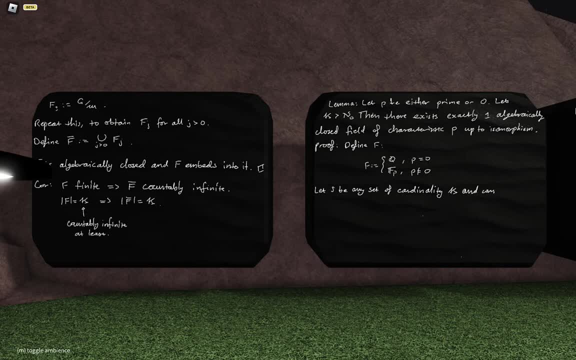 of cardinality, kappa of cardinality, kappa of cardinality kappa, and consider and consider, and consider the field g, which is f, the field g which is f, the field g, which is f price, not square bracket x s price, not square bracket x s price, not square bracket x s, given s is an element of s. 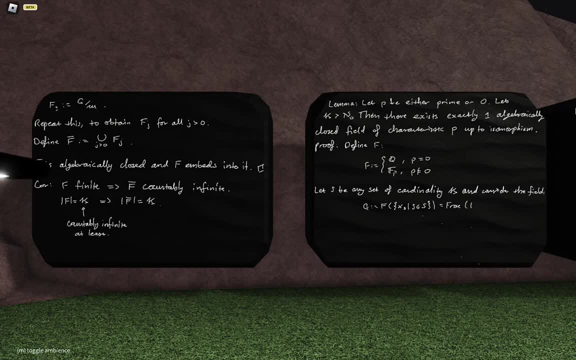 given s is an element of s. given s is an element of s. okay, and that's just the field of okay, and that's just the field of okay, and that's just the field of fractions, fractions, fractions of this polynomial ring, if you're of this polynomial ring, if you're. 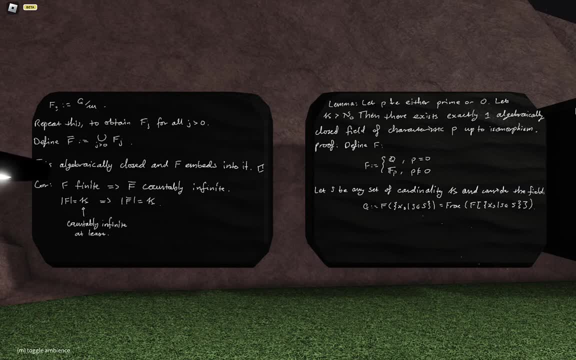 of this polynomial ring. if you're a bit squirmish about the existence of a bit squirmish about the existence of a bit squirmish about the existence of the field that i just wrote down, the field that i just wrote down, the field that i just wrote down, okay, 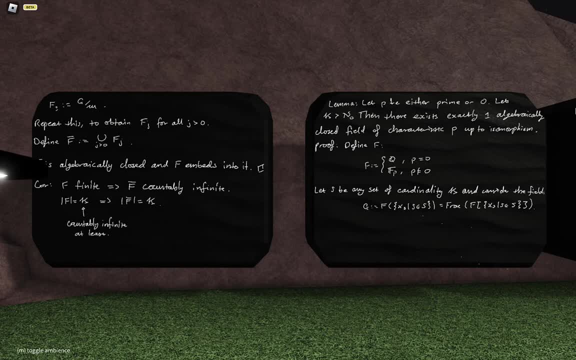 okay, okay, then, from the previous corollary j, then from the previous corollary j, then from the previous corollary j. has cardinality, oh sorry, has cardinality, oh sorry, has cardinality, oh sorry, no, no, not from the previous corollary. no, no, not from the previous corollary. 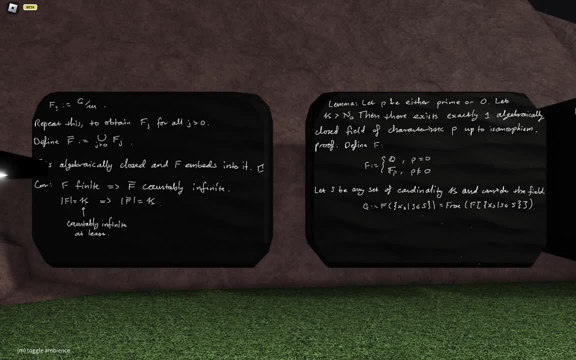 no, no, not from the previous corollary, but just by observation. but just by observation, but just by observation: g has cardinality kappa because of the g has cardinality kappa because of the g has cardinality kappa because of the indeterminates. and then so by the previous corollary. 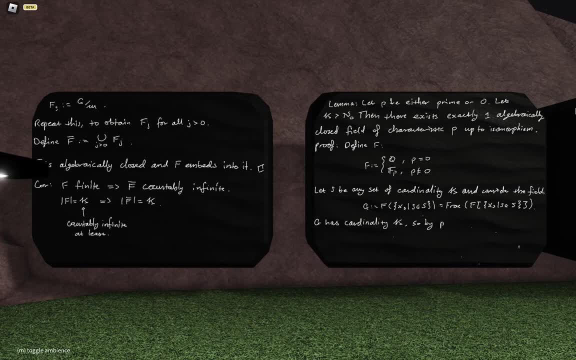 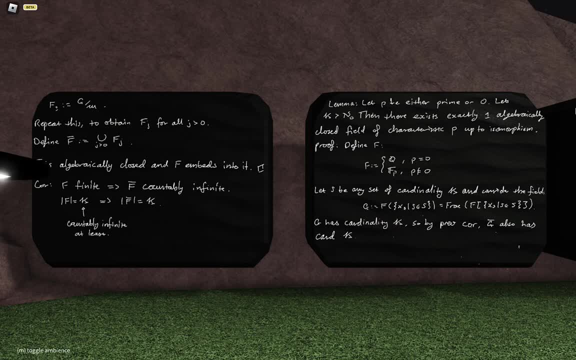 okay, okay, and, as i already said, as i already said, as i already said, could you remind me why the algebraic, could you remind me why the algebraic, could you remind me why the algebraic closure isn't bigger? because we, because we, because we are taking. 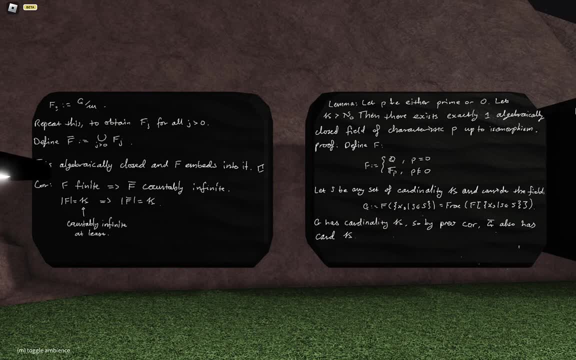 oh, hold on, oh, hold on, oh, hold on. uh, so it's clear. in the case where, uh, so it's clear. in the case where, uh, so it's clear. in the case where, wait, no, so, wait, no, so, wait, no. so the reason why it doesn't have. 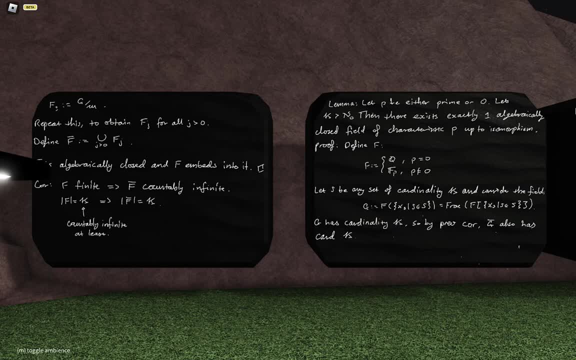 the reason why it doesn't have, the reason why it doesn't have greater cardinality, is because greater cardinality is because greater cardinality is because the, the, the polynomials over a field, the the polynomials over a field, the the polynomials over a field are parameterized, so a polynomial over a. 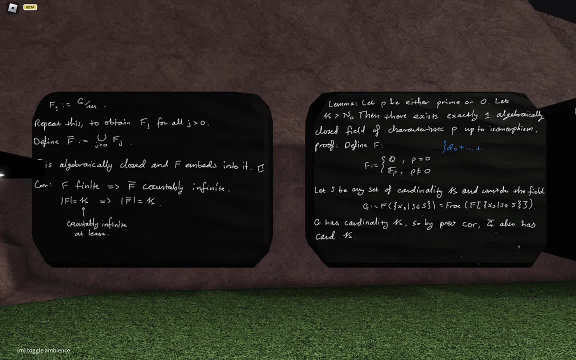 are parameterized, so a polynomial over a are parameterized, so a polynomial over a field looks like this: we're looking at field. looks like this: we're looking at field. looks like this: we're looking at the set of all things alpha naught plus the set of all things alpha naught plus. 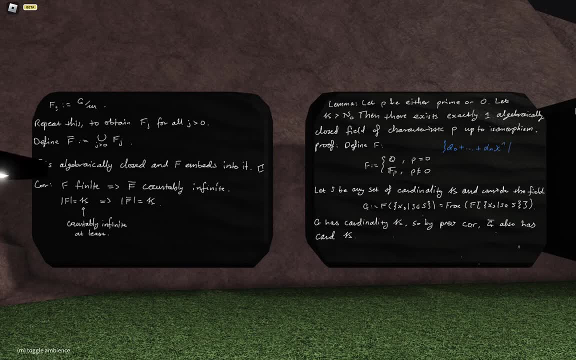 the set of all things. alpha naught plus dot dot dot, plus alpha n x to the n dot, dot dot, plus alpha n x to the n dot, dot dot, plus alpha n x to the n. right given the alpha i are an element. right given the alpha i are an element. 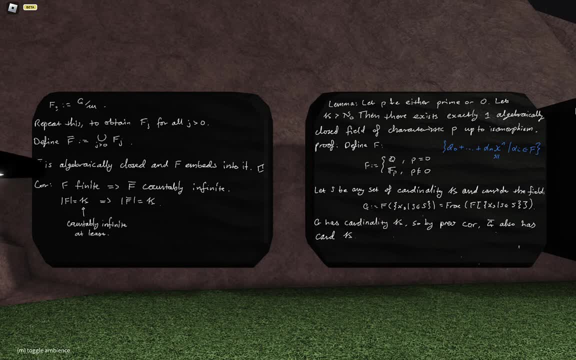 right, given the alpha, i are an element of f, of f, of f, okay, and then, as i said, that's in okay, and then, as i said, that's in okay, and then, as i said, that's in bijection with all of the sequences, bijection with all of the sequences. 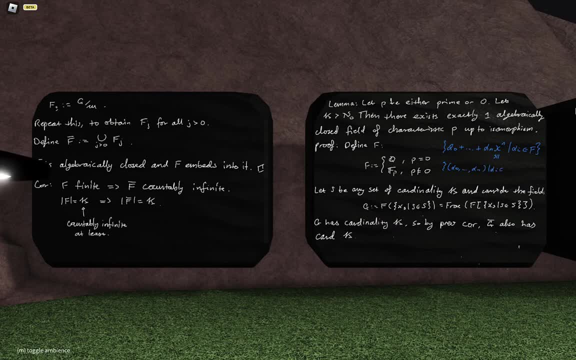 bijection with all of the sequences: alpha naught up to alpha n. alpha naught up to alpha n. alpha naught up to alpha n. given alpha i is an element of n, given alpha i is an element of n, given alpha i is an element of n of f and n is greater than or equal to. 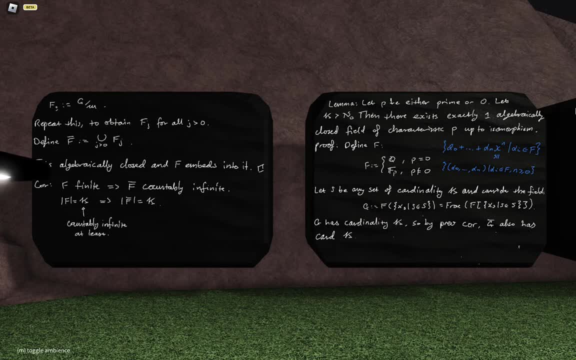 of f and n is greater than or equal to of f and n is greater than or equal to zero, zero, zero, right, and so this is the set of all right, and so this is the set of all sequences: it's a countable union which equals zero. 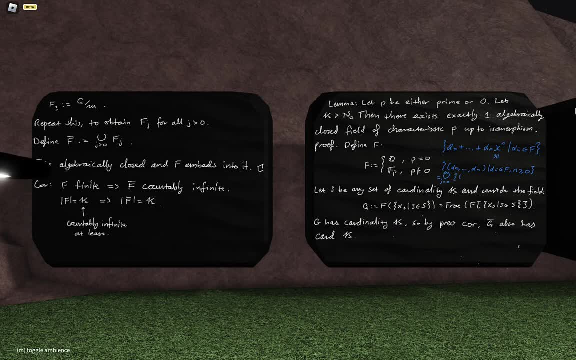 it's a countable union which equals zero. it's a countable union which equals zero up to infinity, up to infinity, up to infinity of the set of sequences of elements inside f, right, and so right and so right, and so the cardinality of that is equal to. 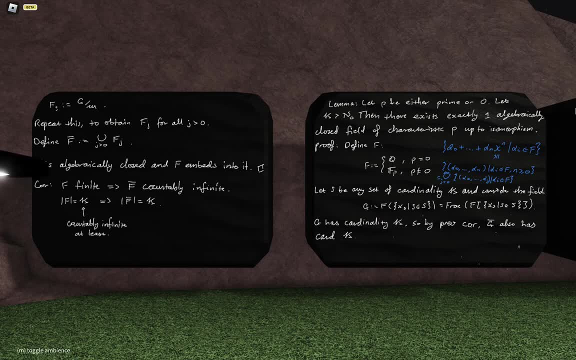 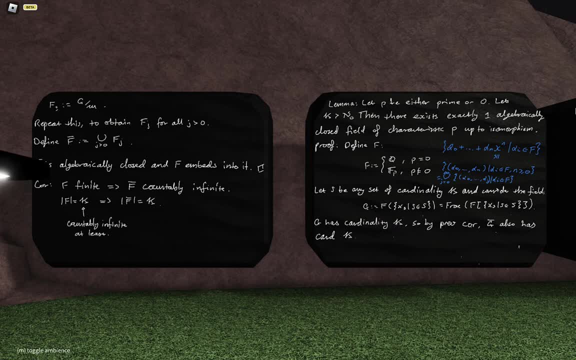 was infinite a priori, was infinite a priori, whereas if f was finite, then this bumps. whereas if f was finite, then this bumps. whereas if f was finite, then this bumps it up to countably infinite, it up to countably infinite, it up to countably infinite. yep. 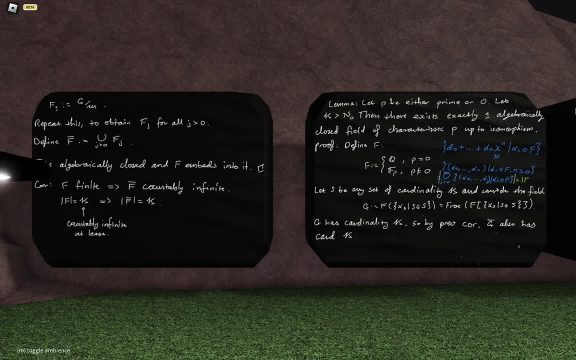 yep, yep, um, um, um, right, right, right. so that's the polynomials over the. so that's the polynomials over the. so that's the polynomials over the field, but then the algebraic closure field, but then the algebraic closure field, but then the algebraic closure involved. like modding out a bit. 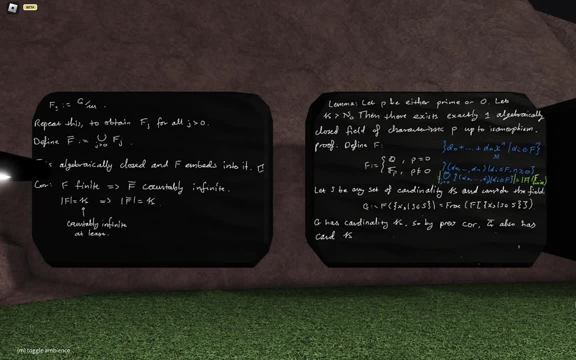 involved, like modding out, a bit involved, like modding out a bit right, right, right. so so so, the modding out, the modding out, the modding out. so are you worried about the modding out. so are you worried about the modding out. so are you worried about the modding out? reducing the size of the algebraic. 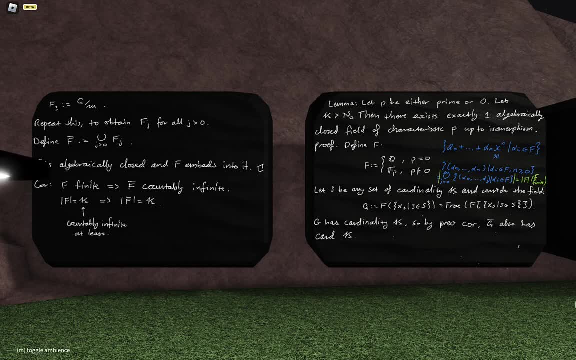 reducing the size of the algebraic, reducing the size of the algebraic closure, closure, closure, uh, uh, uh. yeah, but you said something about f- yeah, but you said something about f. yeah, but you said something about f: embeds into it, embeds into it, embeds into it. yeah, f embeds into it, because we only 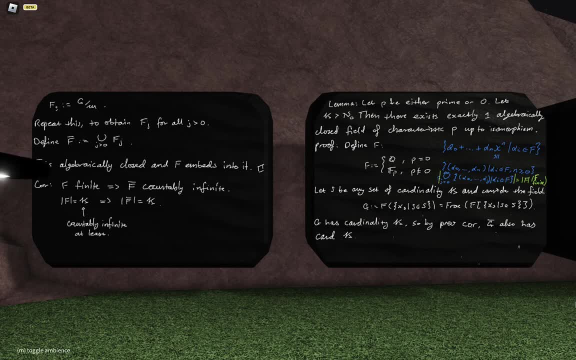 yeah, f embeds into it because we only yeah, f embeds into it because we only ever modded out by in formal, ever modded out by in formal, ever modded out by in formal. indeterminance that we added in. indeterminance that we added in. 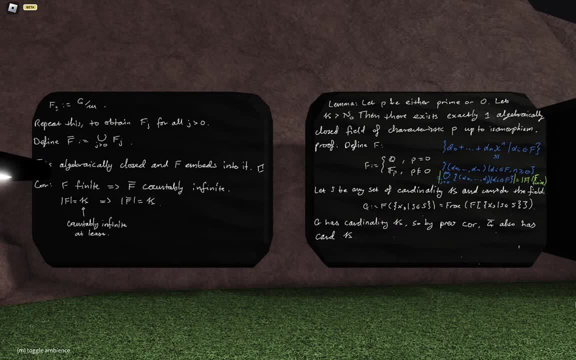 indeterminance that we added in. right right, yeah, right right, yeah, right right. so the coefficients are still there. so f, so the coefficients are still there. so f, so the coefficients are still there. so f, embeds into it, embeds into it, embeds into it. yep. 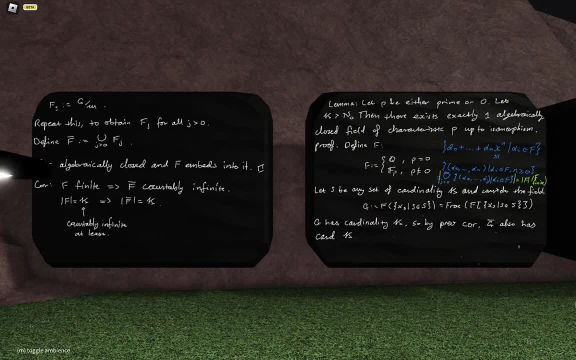 yep, yep, cool, cool, cool, okay, so, okay, so, okay, so, but i need to be careful here in the case. but i need to be careful here in the case. but i need to be careful here in the case. where, where, where p is prime, then fp is. 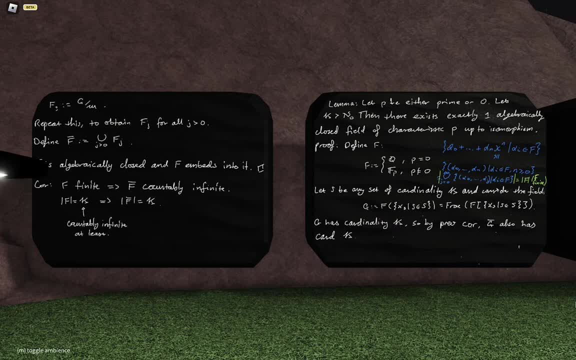 p is prime, then fp is p is prime, then fp is finite cardinality, which means the bottom finite cardinality, which means the bottom finite cardinality, which means the bottom statement is: statement is statement is wrong, wrong, wrong, so. so so g has, g has, g has. yeah, let's no, no, no, this is correct. 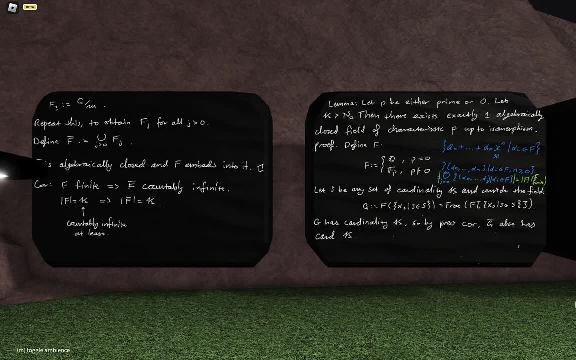 yeah, let's no, no, no, this is correct. yeah, let's no, no, no, this is correct. okay, so i haven't. i haven't used the size. okay, so i haven't. i haven't used the size. okay, so i haven't. i haven't used the size of f here. 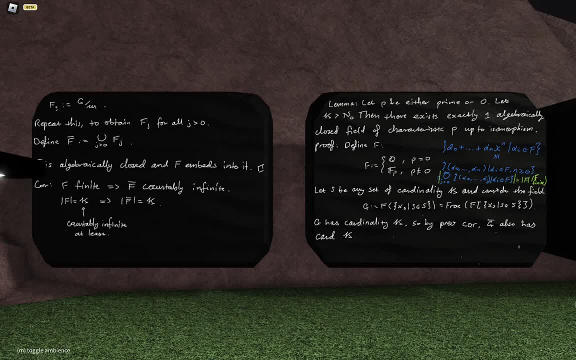 of f here, of f here, um, because um, because um, because f, be it f, be it f, be it a field, a finite field or an or q, a field a finite field or an or q. a field a finite field or an or q. i still, i still. 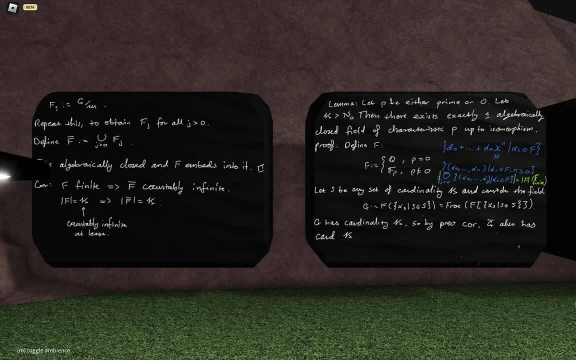 i still adjoin- adjoin adjoin kappa many indeterminates, and so therefore kappa many indeterminates, and so therefore kappa many indeterminates, and so therefore g definitely has cardinality kappa, so g definitely has cardinality kappa, so g definitely has cardinality kappa, so we're fine. 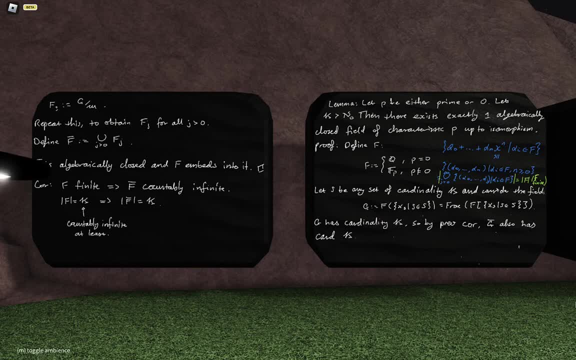 we're fine. we're fine, okay, and now what i need to do is take a. okay, and now what i need to do is take a okay, and now what i need to do is take a transcendental basis, transcendental basis, transcendental basis of uh g, i believe. 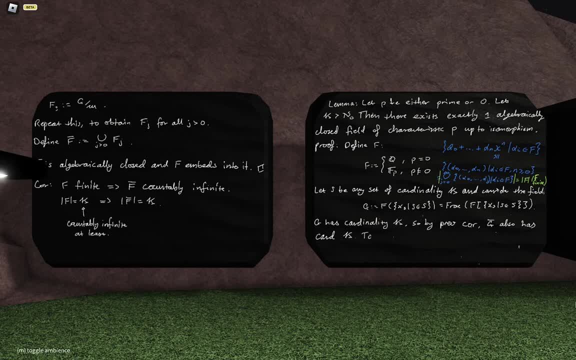 of uh g. i believe of uh g. i believe, yeah, yeah, yeah, yeah, so, yeah, so, yeah. so if i take any transcendental basis, transcendental basis, transcendental basis- a, a, a, of g, and to remind you what that means of g and to remind you what that means, 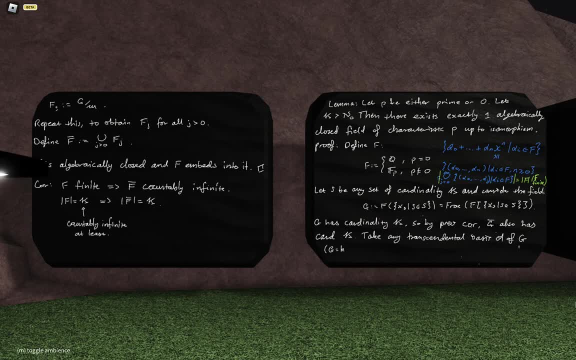 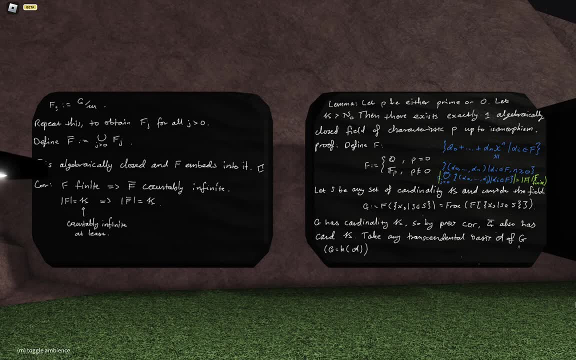 over those elements a right. so that's: over those elements a right. so that's the same notation as beforehand, the same notation as beforehand, the same notation as beforehand. take the polynomial ring with base, take the polynomial ring with base. take the polynomial ring with base. field k: 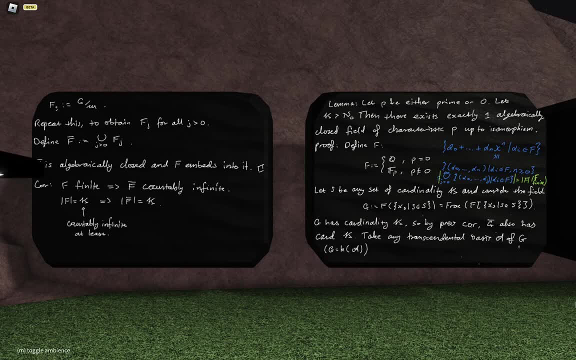 field k, field k over these elements a, and then take the over these elements a, and then take the over these elements a, and then take the field of fractions, field of fractions, field of fractions, if that thing is isomorphic to the, if that thing is isomorphic to the. 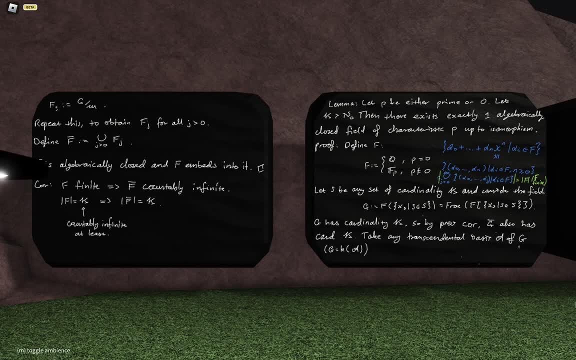 if that thing is isomorphic to the original field that you started off with, original field that you started off with original field that you started off with, and since it's a and since it's a and since it's a subfield, it's, it's equal on the nose. 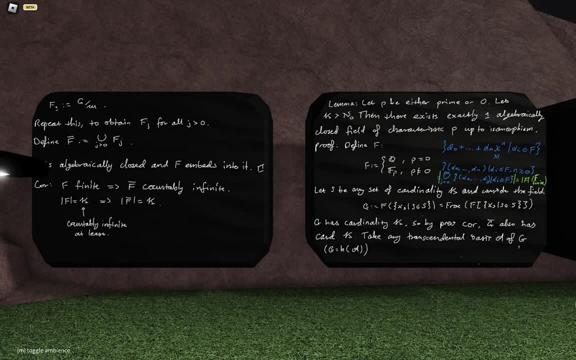 subfield: it's: it's equal on the nose. subfield: it's: it's equal on the nose. if that is the case, then a is called a. if that is the case, then a is called a. if that is the case, then a is called a. transcendental basis of g. 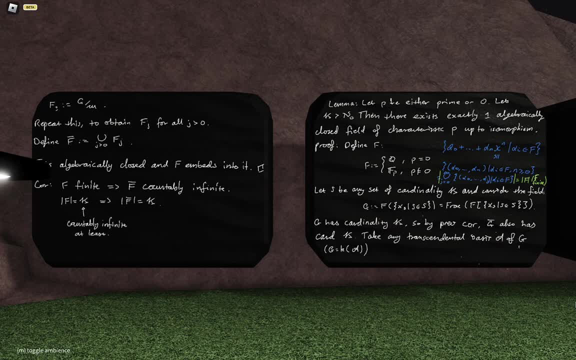 transcendental basis of g, transcendental basis of g, and we observe that a has to have, and we observe that a has to have, and we observe that a has to have cardinality, cardinality, cardinality, kappa, and again it's the same argument that, and again it's the same argument that. 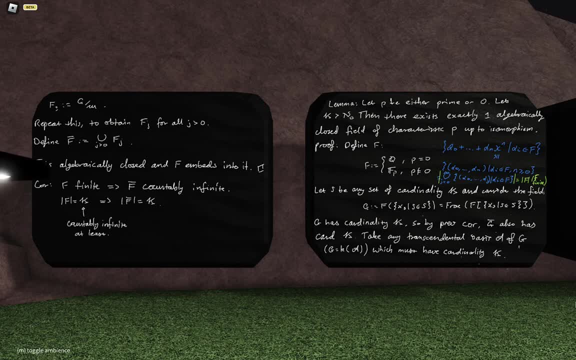 and again, it's the same argument that we've been using. we've been using. we've been using is equal to all of the polynomials, is equal to all of the polynomials, is equal to all of the polynomials over a and so the set that we started. 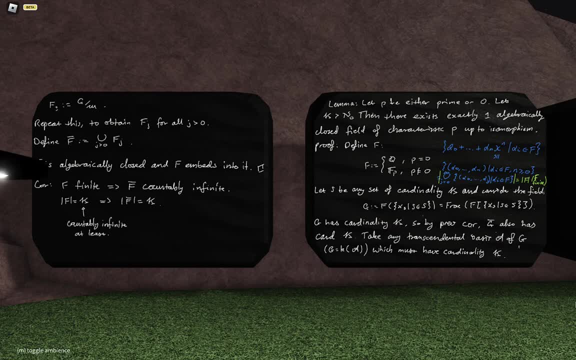 over a, and so the set that we started over a, and so the set that we started off with, off with off with. if that was finite or countable, if that was finite or countable, if that was finite or countable, then polynomials over that would be: 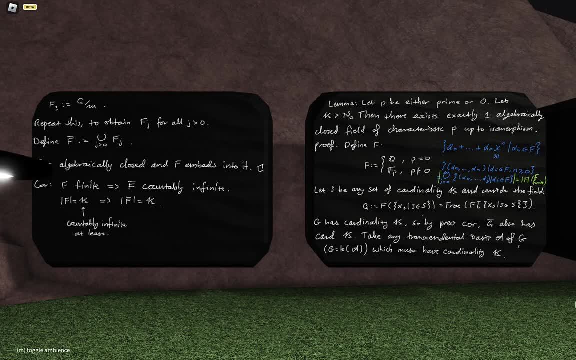 then polynomials over that would be, then polynomials over that would be countable. but we know that kappa is countable, but we know that kappa is countable, but we know that kappa is greater than that, greater than that, greater than that. so therefore kappa, so therefore a has. 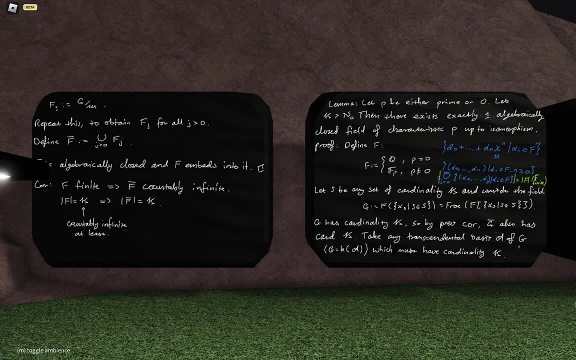 so therefore kappa, so therefore a has, so therefore kappa. so therefore, a has got cardinality kappa, got cardinality kappa, got cardinality kappa. okay, moving on to the next board. okay, moving on to the next board. okay, moving on to the next board. now, if i let h, 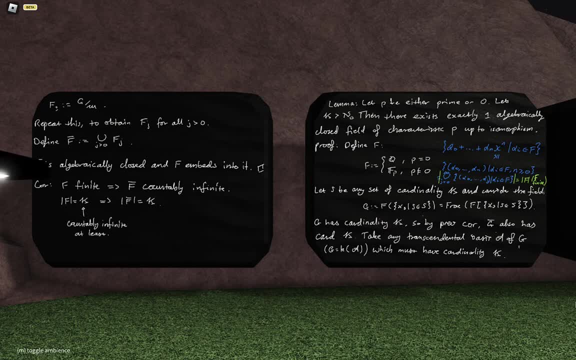 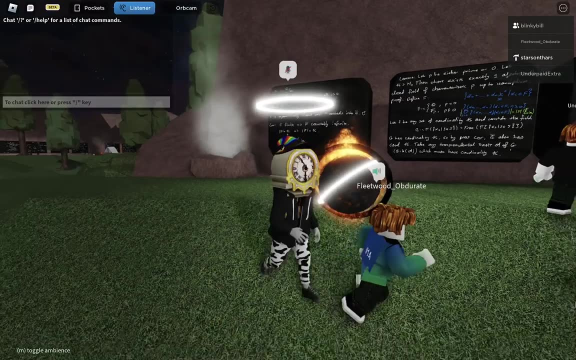 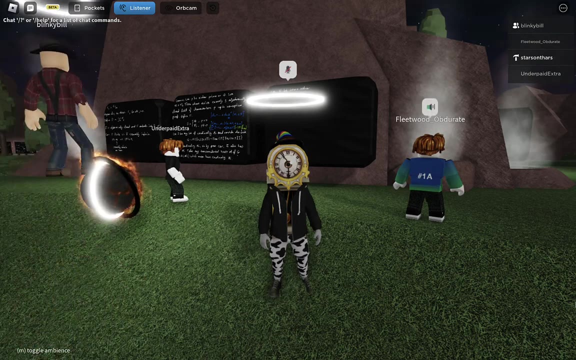 now, if i let h, now, if i let h be some other, um, um, um, you gotta move your character. you gotta move your character. you gotta move your character. i'll do it, i'll do it, i'll do it. oh yeah, sorry, i forgot which. okay, if h was any other. 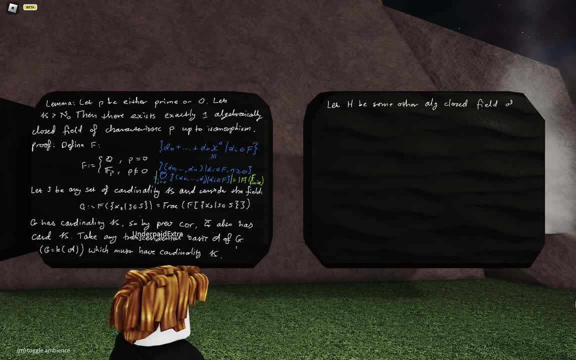 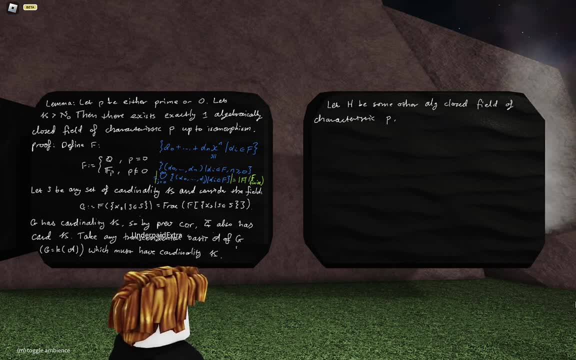 also, also a transcendental basis of h, which has a transcendental basis of h, which has a transcendental basis of h, which has cardinality. kappa. what did i call it? i called it. what did i call it? i called it. what did i call it? i called it. 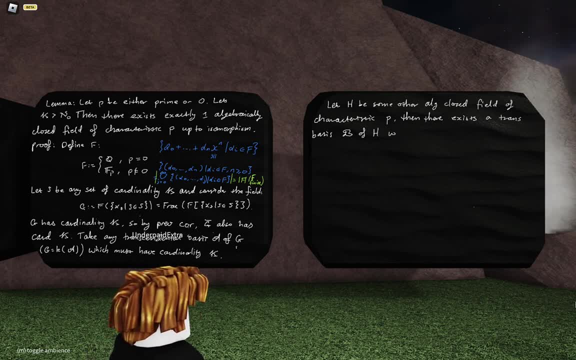 a. yeah, so b a. yeah, so b a. yeah, so b of h with cardinality kappa, with cardinality kappa, with cardinality kappa. so therefore there exists a bijection. so therefore there exists a bijection. so therefore there exists a bijection between a and b. 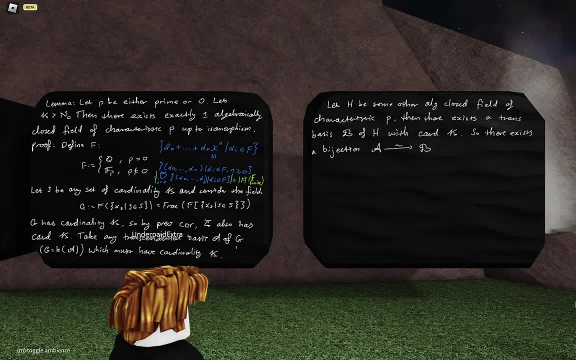 and that induces, and that induces, and that induces an isomorphism between, an isomorphism between, an isomorphism between the polynomial field over a and the, the polynomial field over a, and the, the polynomial field over a and the polynomial field over k. so again, i think i misspoke. so this: 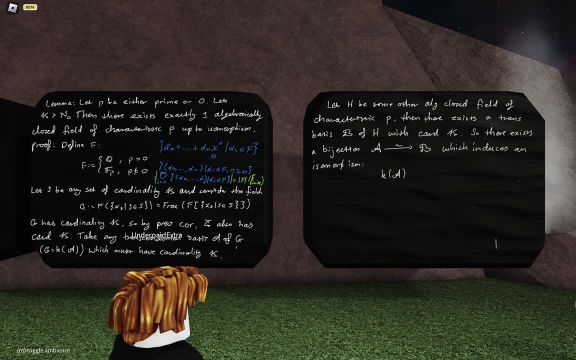 so again i think i misspoke. so this: so again i think i misspoke. so this induces an isomorphism. induces an isomorphism between the polynomial field with. induces an isomorphism between the polynomial field with. induces an isomorphism between the polynomial field with base field, k over a and. 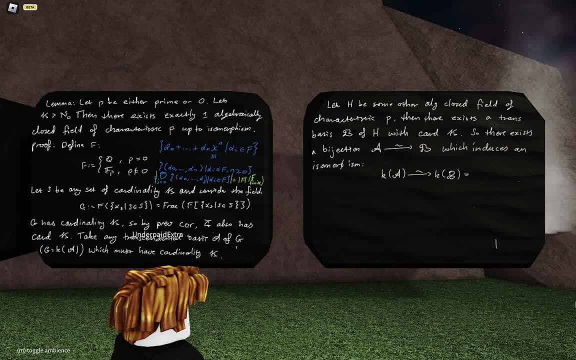 base field k over a, and base field k over a, and the same such thing, but over b. the same such thing, but over b. the same such thing, but over b. and then don't forget that by hypothesis. and then don't forget that by hypothesis. and then don't forget that by hypothesis that one's equal to h. 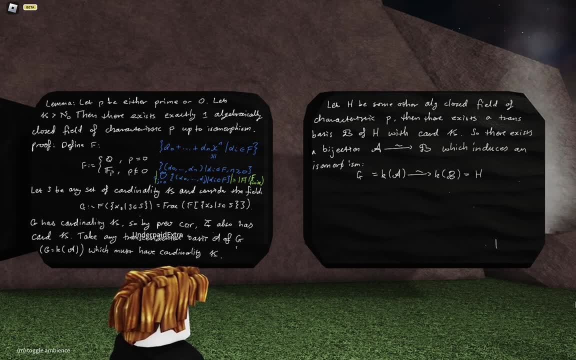 that one's equal to h. that one's equal to h. and this one's equal to g- right, okay. and this one's equal to g- right okay. and this one's equal to g- right okay. and now we just take the algebraic. and now we just take the algebraic. 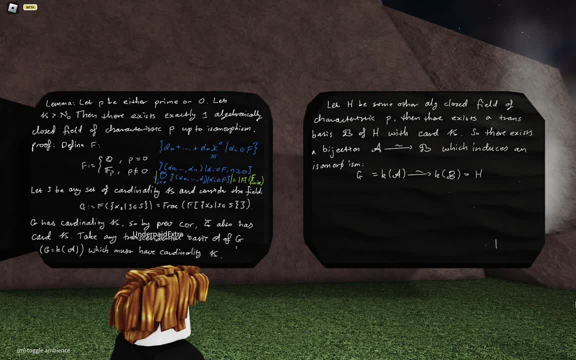 and now we just take the algebraic closure of both sides and closure of both sides and closure of both sides. and since we have an isomorphism of the, since we have an isomorphism of the, since we have an isomorphism of the base fields, that induces an isomorphism. 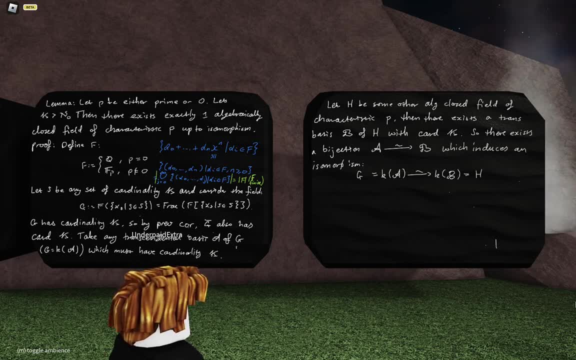 base fields that induces an isomorphism. base fields that induces an isomorphism on the algebraic closures, on the algebraic closures, on the algebraic closures. so we have g bar is isomorphic to k. so we have g bar is isomorphic to k. 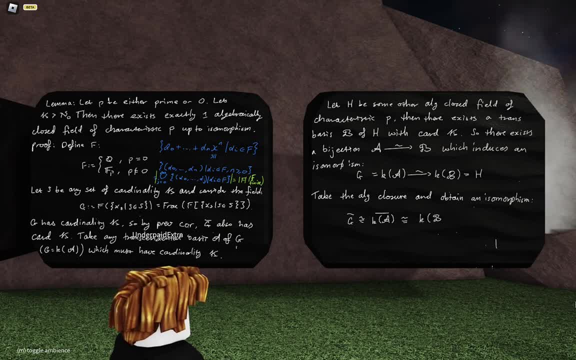 so we have: g bar is isomorphic to k of a bar is isomorphic to k of a bar is isomorphic to k of a bar is isomorphic to k of b bar is isomorphic to h of b bar is isomorphic to h of b bar is isomorphic to h bar. so therefore, g bar is isomorphic to. 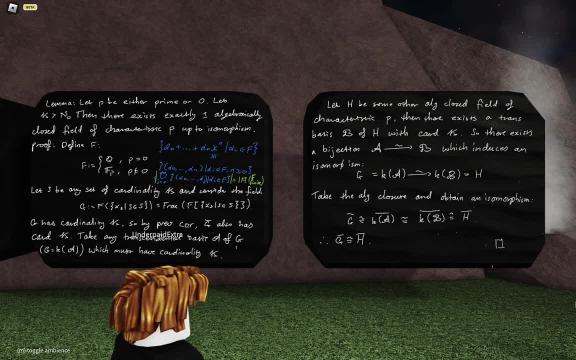 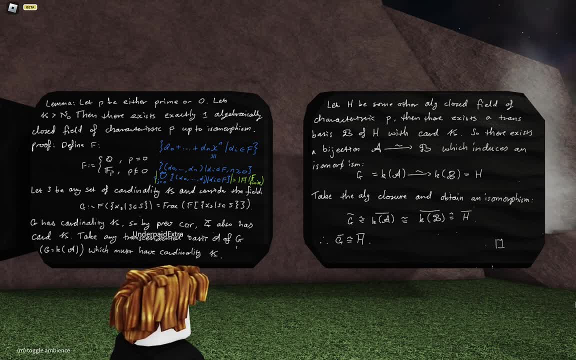 so now we can see that. so now we can see that the first order theories of algebraically, the first order theories of algebraically, the first order theories of algebraically, closed fields of characteristic p or p, closed fields of characteristic p or p, closed fields of characteristic p or p, is at the prime of zero. 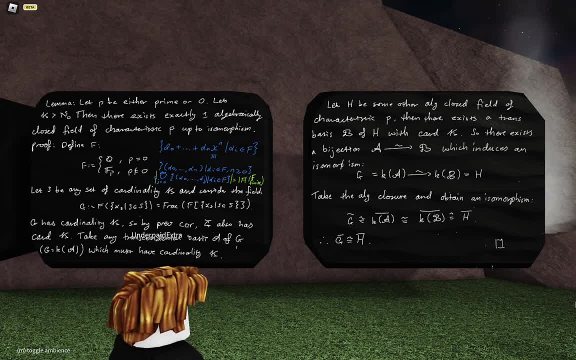 is at the prime of zero, is at the prime of zero, satisfy the conditions of the wash vort, satisfy the conditions of the wash vort, satisfy the conditions of the wash vort. test and so test and so test, and so, therefore, these are both complete. therefore, these are both complete. 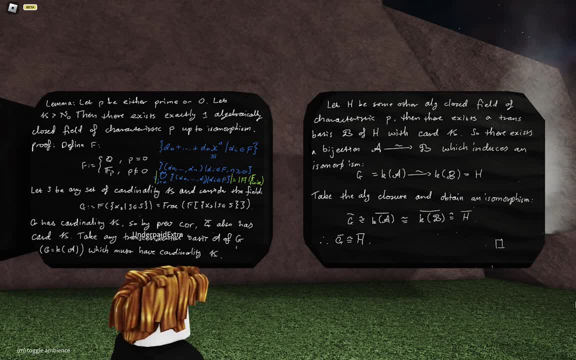 therefore, these are both complete theories and that was the theories and that was the theories, and that was the only remaining assumption that i made in only remaining assumption that i made in only remaining assumption that i made in the first half of the proof which i've, the first half of the proof which i've. 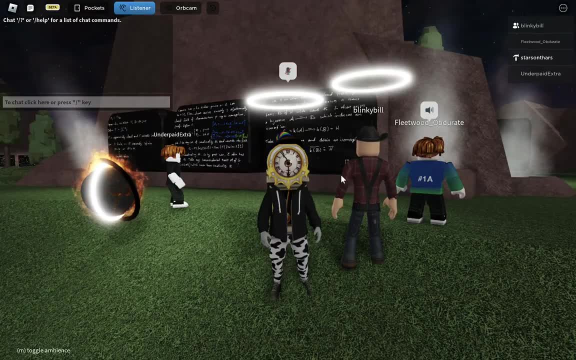 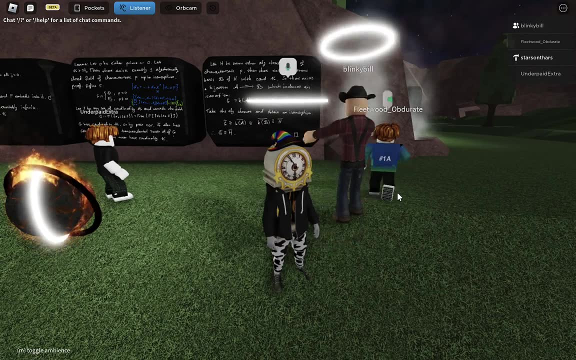 the first half of the proof which i've already done, already done, already done. second place to proof of the x growth. second place to proof of the x growth. second place to proof of the x growth index theorem. any questions on the last bit? any questions on the last bit. 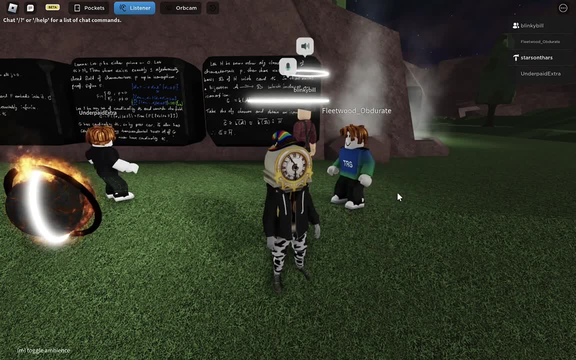 any questions? on the last bit: um i, the. the conclusion of this is that um i, the. the conclusion of this is that um i the. the conclusion of this is that the algebraic closer of g, the algebraic closer of g, the algebraic closer of g and of h- isomorphic, yeah, but 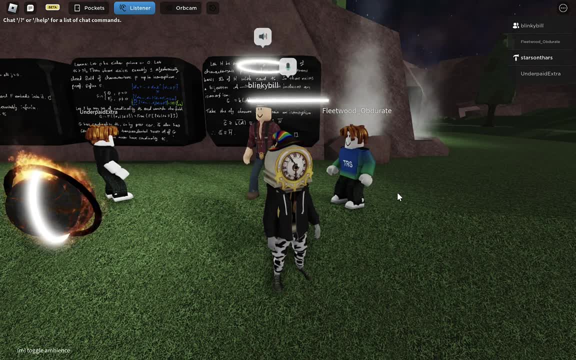 and of h isomorphic, yeah, but and of h isomorphic, yeah, but when g and h the algebraically closed, when g and h the algebraically closed, when g and h the algebraically closed, fields of characteristic p. fields of characteristic p. fields of characteristic p um. 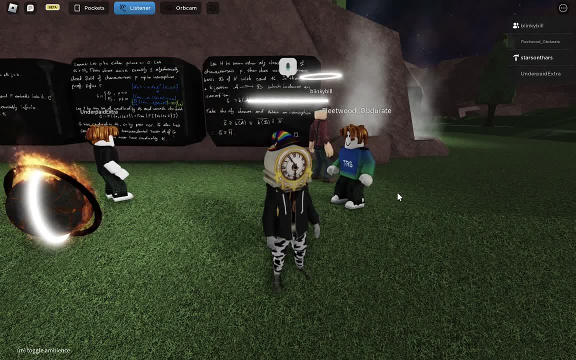 um, um, um, um didn't. we want to show that g and h didn't. we want to show that g and h didn't. we want to show that g and h were, were, were. i saw that's a good point. i mean i have. i saw that's a good point, i mean i have. 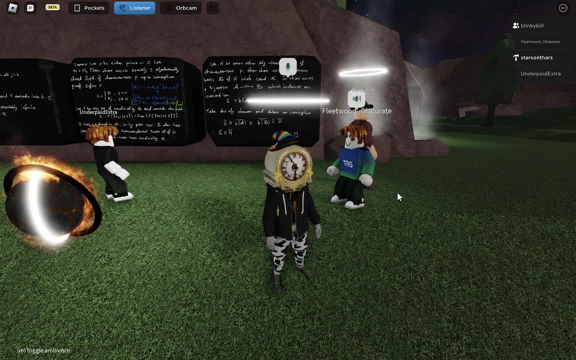 i saw that's a good point. i mean i have that anyway. so wait, what am i trying to that anyway? so wait, what am i trying to that anyway? so wait, what am i trying to say? say, say, oh, i think it's. i think i don't need a bar here, yeah. 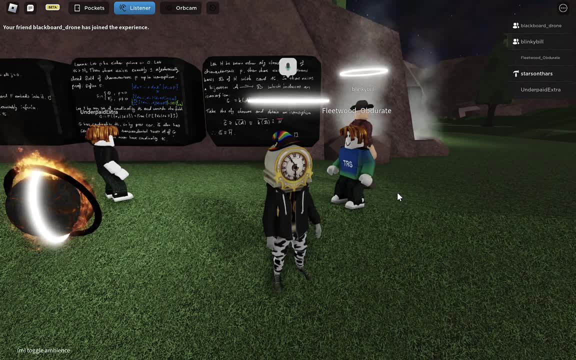 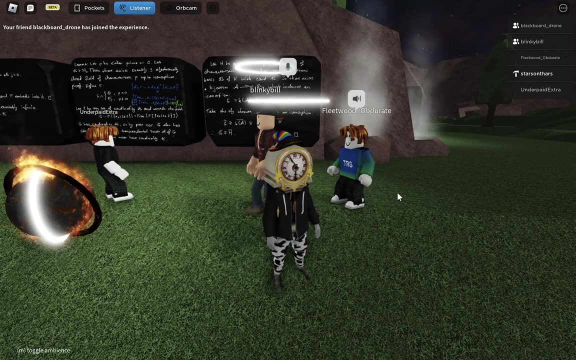 i think i don't need a bar here. yeah, i think i don't need a bar here. yeah, okay, good, so j was not an algebraic problem. so j was not an algebraic problem. so j was not an algebraic problem. yes, because hold up. yeah, there is. 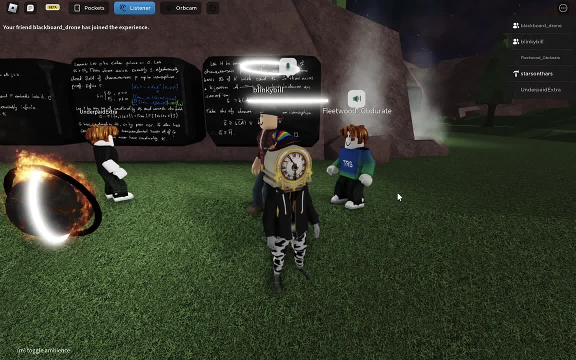 yes, because hold up. yeah, there is yes because hold up. yeah, there is something wrong here, so that's a subset. something wrong here, so that's a subset. something wrong here, so that's a subset. okay, sorry, i made some mistakes here. i okay. sorry, i made some mistakes here. i. 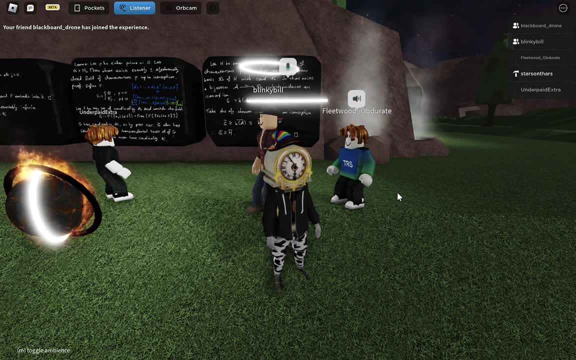 okay, sorry, i made some mistakes here. i don't know it must be tied to that, or don't know it must be tied to that, or don't know it must be tied to that, or something, something, something. okay, i have taken. okay, i have taken. okay, i have taken a transcendental basis for h. 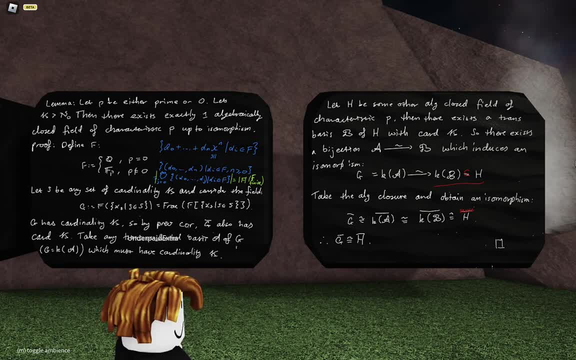 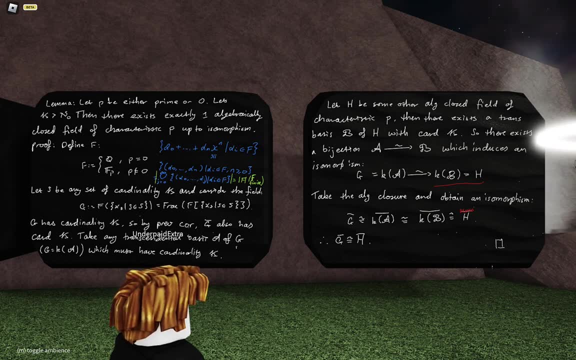 a transcendental basis for h, a transcendental basis for h. so this interesting? so no, no. the equalities are interesting, so no, no, the equalities are interesting, so no, no, the equalities are true, but the last one's true. but the last one's true, but the last one's trivial right. so i take the. 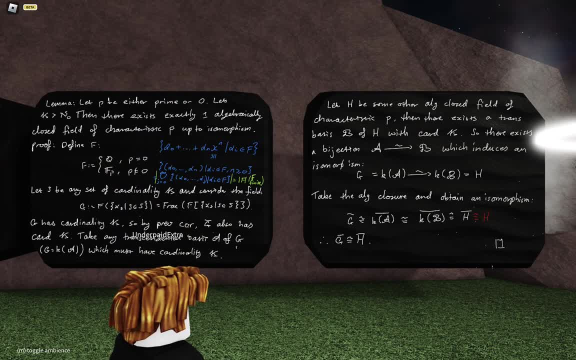 trivial right. so i take the trivial right. so i take the algebraic closure of h. but that's algebraic closure of h, but that's algebraic closure of h, but that's isomorphic to h, isomorphic to h, isomorphic to h. uh-huh. 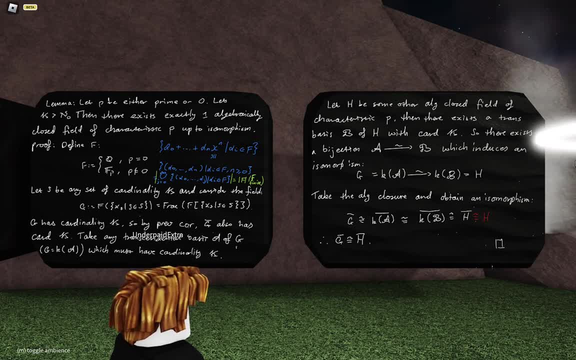 uh-huh, uh-huh, because h was algebraically closed to, because h was algebraically closed to, because h was algebraically closed to begin with, but j wasn't right begin with, but j wasn't right begin with, but j wasn't right j j, j was some field that i constructed, and then i 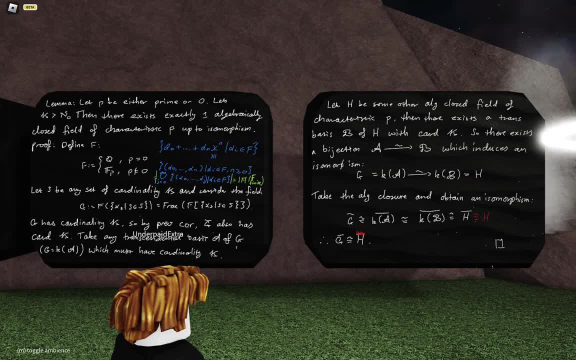 was some field that i constructed. and then i was some field that i constructed and then i took its algebraic closure and then i said, took its algebraic closure, and then i said, took its algebraic closure, and then i said that that thing is unique, and how do i? that that thing is unique. and how do i that that thing is unique and how do i prove that? i assume that i have some prove that. i assume that i have some prove that. i assume that i have some other thing which is h, other thing which is h. 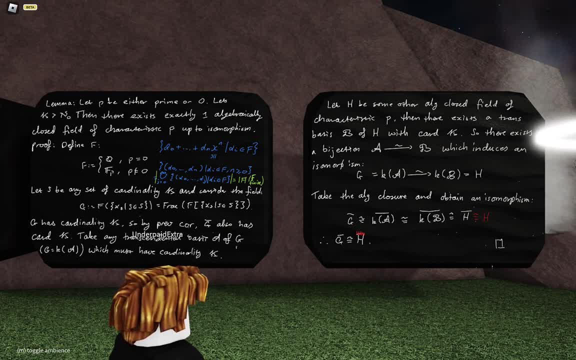 other thing, which is h, which is algebraically closed. so there's which is algebraically closed, so there's which is algebraically closed, so there's no bar, no bar, no bar. and then i prove that there's nice, and then i prove that there's nice. 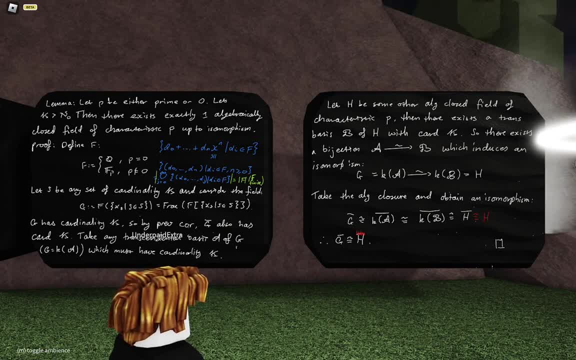 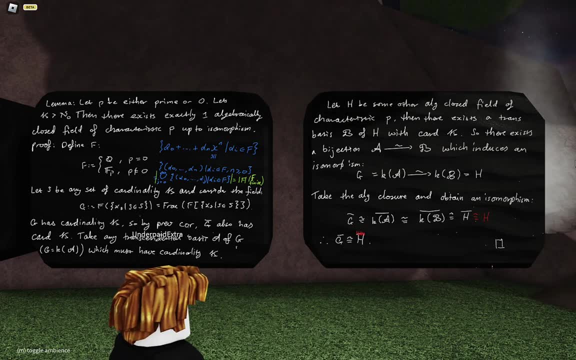 and then i prove that there's nice morphism between them. and sorry, could you go over the first and sorry, could you go over the first and sorry? could you go over the first part of the story, like you started with part of the story, like you started with. 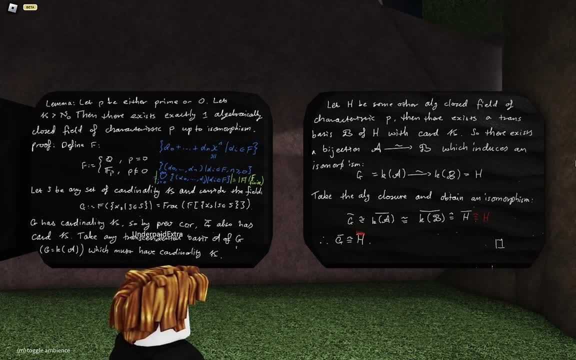 part of the story. like you started with f. what's the role of f and f? what's the role of f and f? what's the role of f and why? why don't we start with f and then? why? why don't we start with f and then? 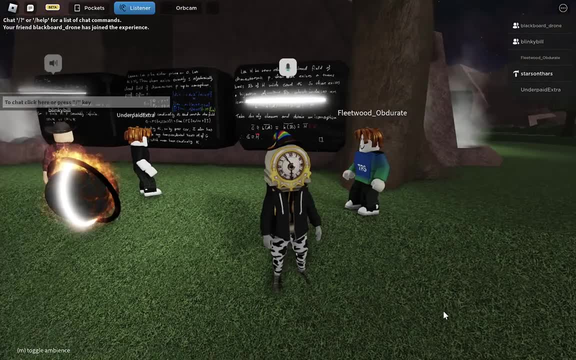 why? why don't we start with f, and then the reason why f disappears. the reason why f disappears. the reason why f disappears. shouldn't we be fixing an arbitrary g? shouldn't we be fixing an arbitrary g? shouldn't we be fixing an arbitrary g, which is an algebraically closed field? 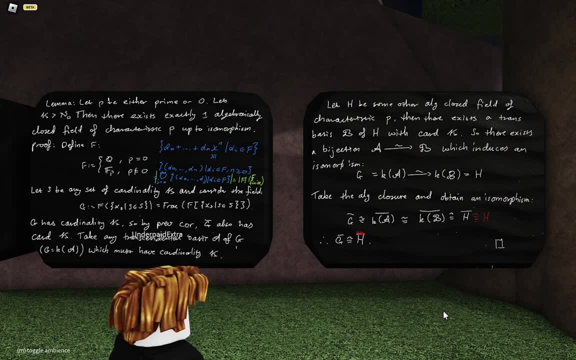 which is an algebraically closed field, which is an algebraically closed field of characteristic p, of characteristic p, of characteristic p, not like this particular one constructed, not like this particular one constructed, not like this particular one constructed from f, from f, from f. so the point is: 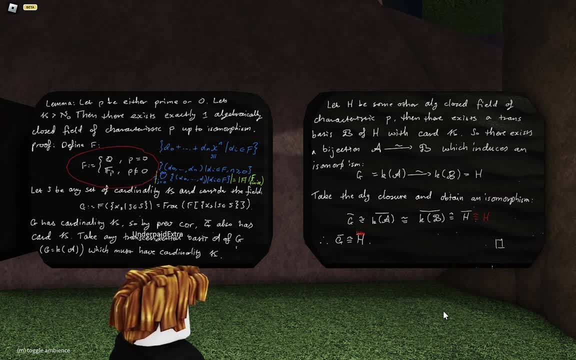 so the point is so. the point is: no matter what j you pick, no matter what j you pick, no matter what j you pick, f is a subfield of it, f is a subfield of it. f is a subfield of it. so you can just take the. 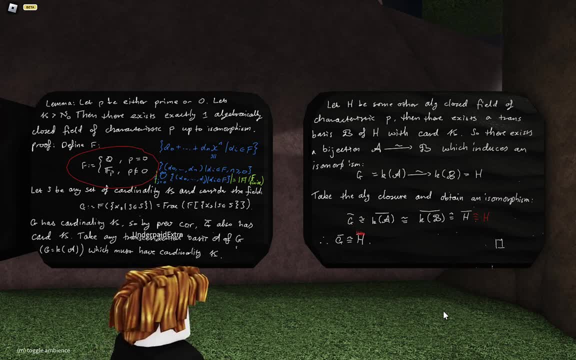 so you can just take the. so you can just take the element one inside your field, and then element one inside your field, and then element one inside your field, and then consider one plus one and one plus one. consider one plus one and one plus one. consider one plus one and one plus one plus one and one plus one plus one plus. 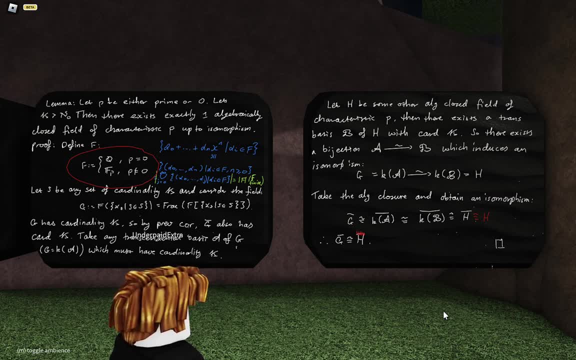 plus one and one plus one plus one plus plus one and one plus one plus one plus one, dot dot. and that gives you a subset dot dot dot, and that gives you a subset dot dot dot, and that gives you a subset which, in fact, is a sub ring, which, in 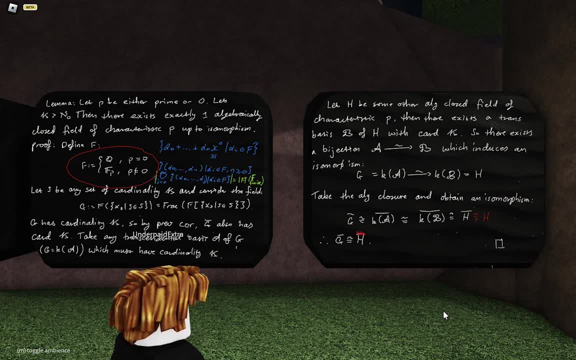 which in fact, is a sub ring, which in which, in fact, is a sub ring which, in fact, is a sub field right fact is a sub field right. fact is a sub field right. and so those sub fields are either q or, and so those sub fields are either q or 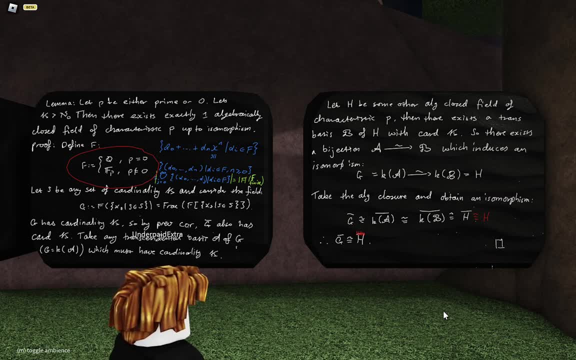 and so those sub fields are either q or fp, as i've written here. so yeah, the fp. as i've written here. so yeah, the fp. as i've written here. so yeah, the statement is about arbitrary g, but the statement is about arbitrary g. but the statement is about arbitrary g, but the point is, any arbitrary g will have f. 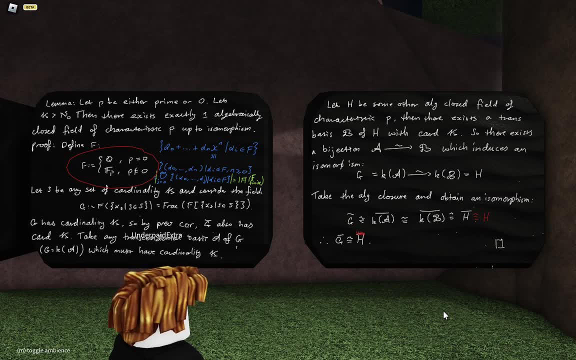 point is any arbitrary: g will have f. point is any arbitrary: g will have f as a sub field. and that's where i as a sub field, and that's where i as a sub field, and that's where i started. and then, what properties of f did you? 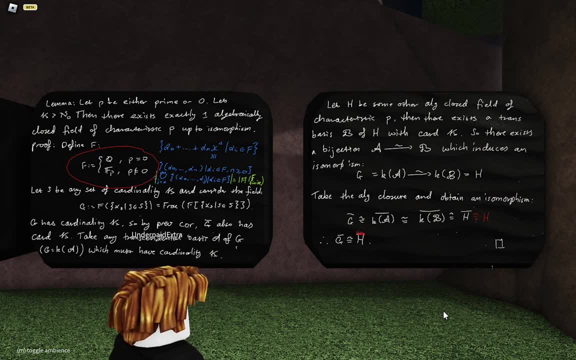 and then what properties of f did you, and then what properties of f did you use? use? use cardinality properties, cardinality properties, cardinality properties. so i quickly, kind of, i quickly kind of, i quickly kind of modded out by, modded out, by modded out by the difference between p- equals zero- and p. 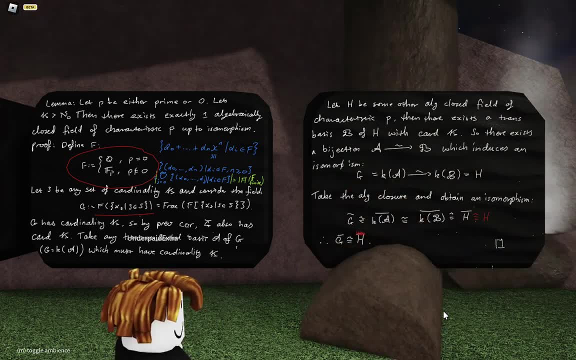 the difference between p equals zero and p, the difference between p equals zero and p not equal to zero, by adjoining all of not equal to zero, by adjoining all of not equal to zero. by adjoining all of these different, these different, these different, um indeterminates, right and once i've 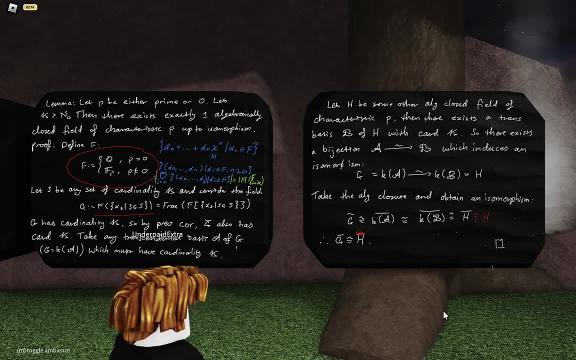 um indeterminates right and once i've um indeterminates right and once i've done that, done that, done that, bf finite or uncountable. this thing now bf finite or uncountable. this thing, now bf finite or uncountable. this thing now has cardinality kappa. 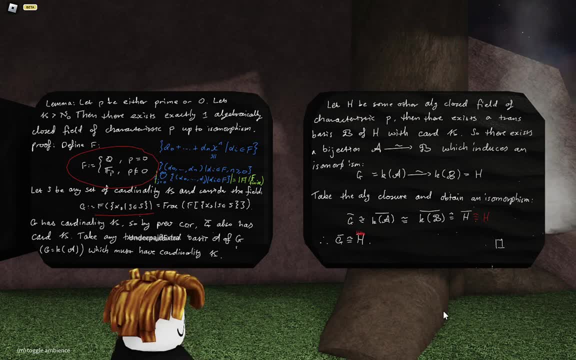 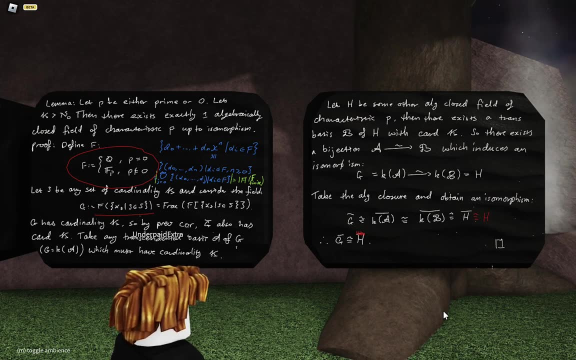 has cardinality kappa, has cardinality kappa, right, so that's a property of f, but not a very so, that's a property of f, but not a very so, that's a property of f, but not a very deep one, deep one, deep one. and then i just worked with j from the 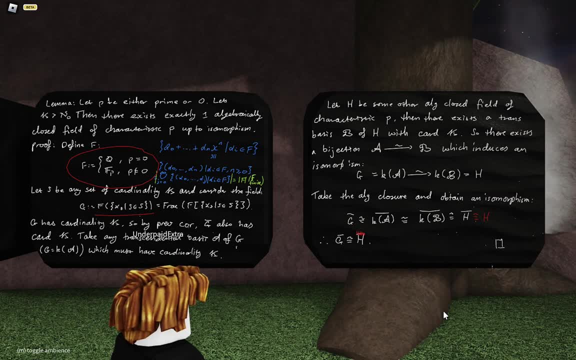 and then i just worked with j from the and then i just worked with j from the other ones, because other ones, because other ones, because i had a. i had a grip on it. okay, all right, are there floating trees again? all right, are there floating trees again? 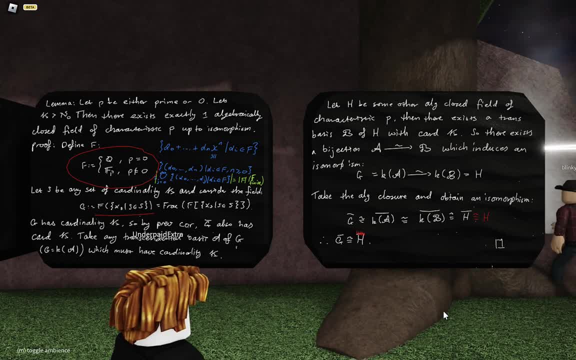 all right, are there floating trees again? yeah, it looks like it. yeah, it looks like it. yeah, it looks like it cool. yeah, all right, there's a tree cool. yeah, all right, there's a tree cool. yeah, all right, there's a tree behind that last board. it just it's. 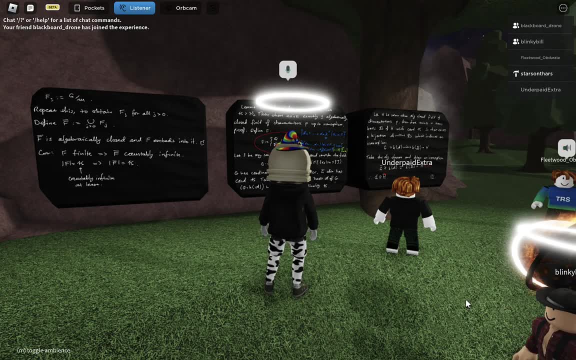 behind that last board. it just it's behind that last board, it just it's just listening, relax, it's interested, just listening, relax, it's interested, just listening, relax, it's interested. oh okay, yeah, i've got nothing to be. oh okay, yeah, i've got nothing to be. 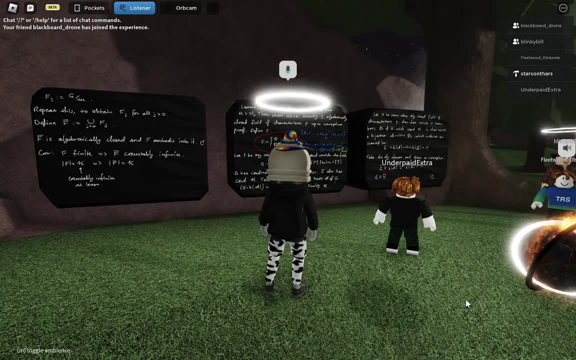 oh okay, yeah, i've got nothing to be scared of, scared of, scared of. it's actually stuck. oh no, it's not, it's actually stuck. oh no, it's not, it's actually stuck. oh no, it's not. anyway you, you are not its prey tonight. anyway you, you are not its prey tonight. 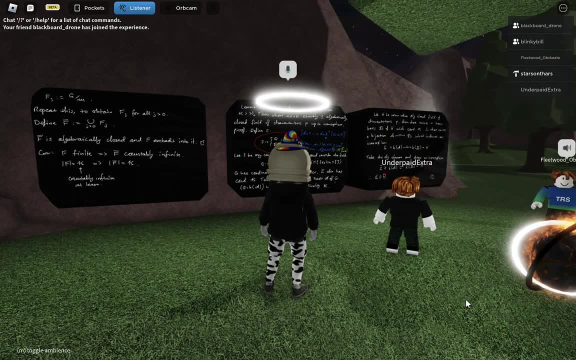 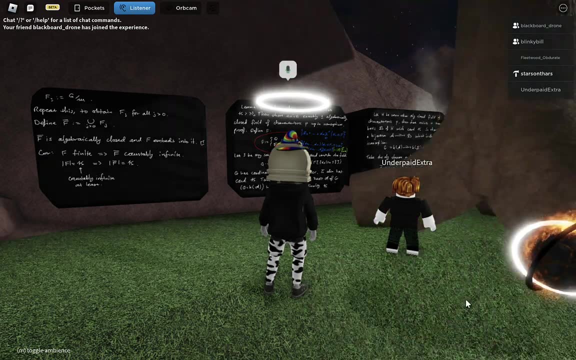 anyway, you, you are not its prey tonight. someone, all right, good, you're trying to trap me, well, you're trying to trap me, well, you're trying to trap me well. no, no, no, um, but i'm about to, i'm about to give my, but i'm about to, i'm about to give my. 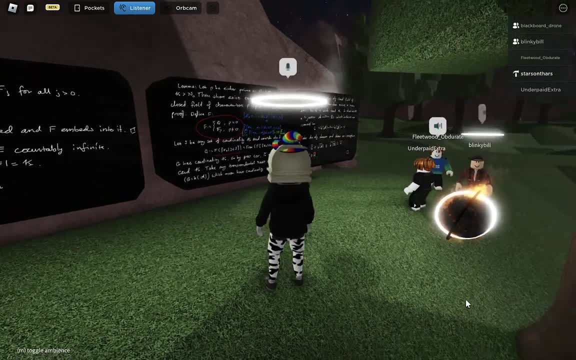 but i'm about to, i'm about to give my claws for claws for claws, for category theory here now. so thanks, i've category theory here now. so thanks, i've category theory here now. so thanks, i've been hit off, but i've got like i've. 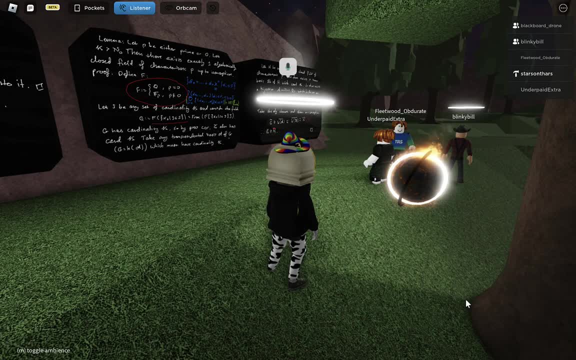 been hit off but i've got, like i've been hit off but i've got, like i've got another minute, got another minute, got another minute. are there any final questions? or we're. are there any final questions or we're. are there any final questions or we're done? i don't have a question, thanks will. 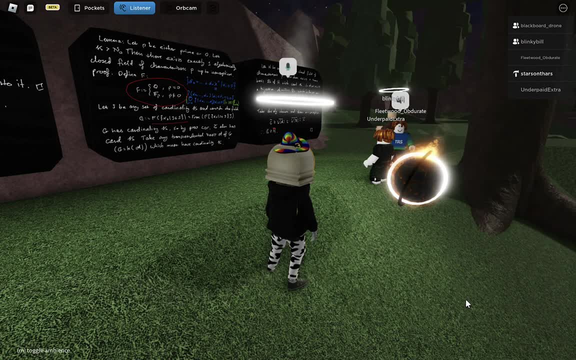 done. i don't have a question, thanks will done. i don't have a question, thanks will. sounds good, sounds good. sounds good, yeah, that's right, thanks. did you have? yeah, that's right, thanks. did you have? yeah, that's right, thanks. did you have any other concluding thoughts about? 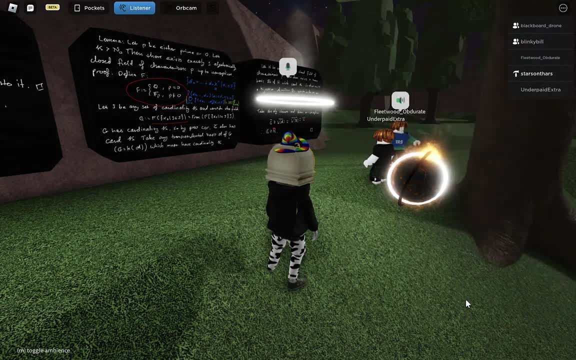 any other concluding thoughts about. any other concluding thoughts about: yeah, i've got a lot of concluding, yeah, i've got a lot of concluding, yeah, i've got a lot of concluding thoughts, but thoughts, but thoughts. but i want to write them out kind of. i want to write them out kind of 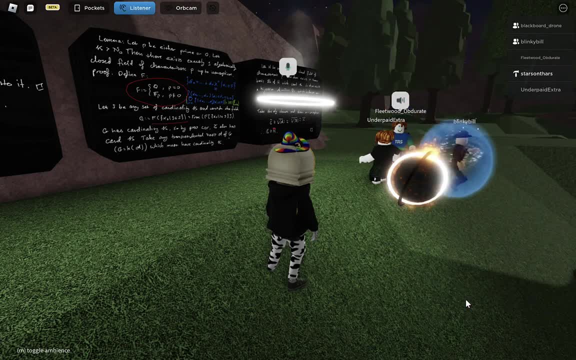 i want to write them out kind of properly, properly, properly, so i won't, i won't send them here, and so i won't, i won't send them here, and so i won't, i won't send them here and i'll save them. i'll save them. 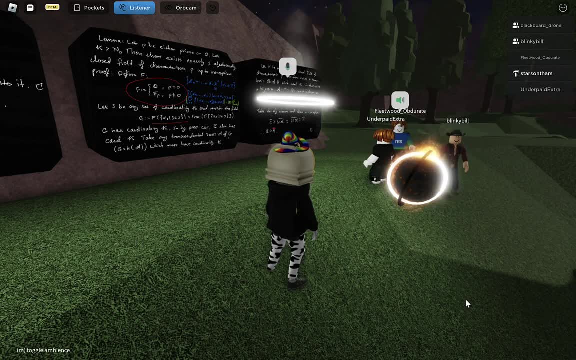 i'll save them from the recording and i don't know post from the recording and i don't know post from the recording and i don't know post them on the them, on the them, on the, on the channel or something on the channel or something on the channel or something. uh-huh cool.